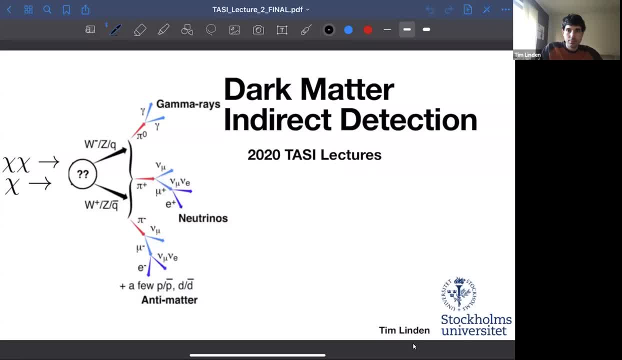 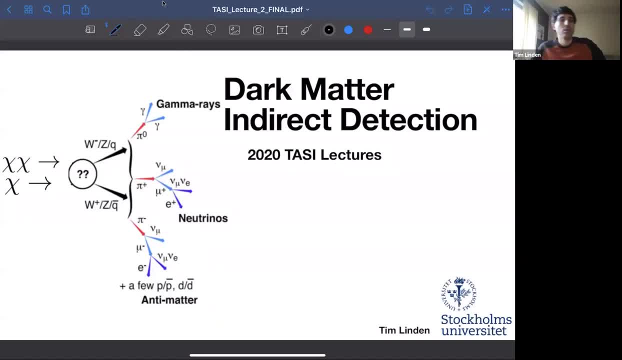 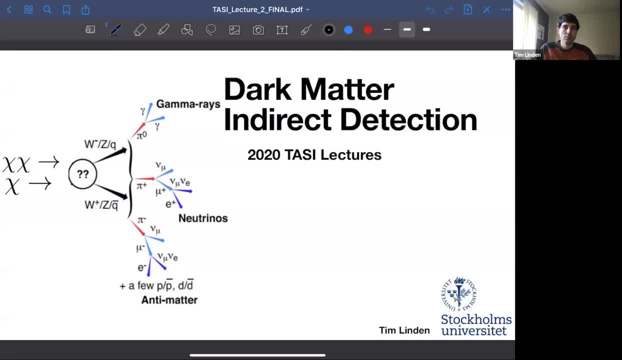 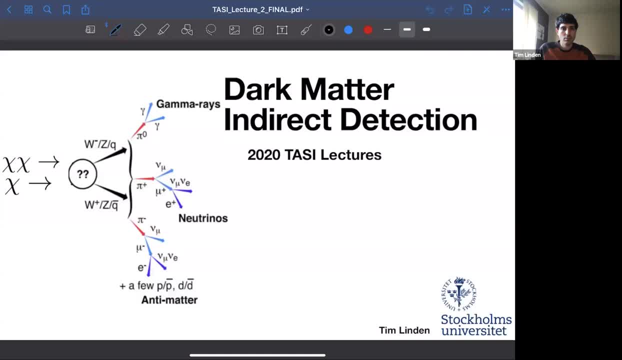 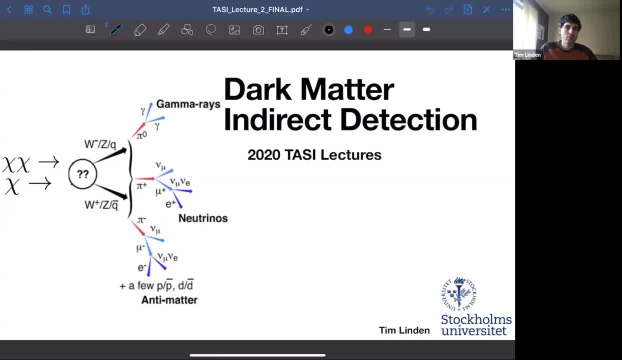 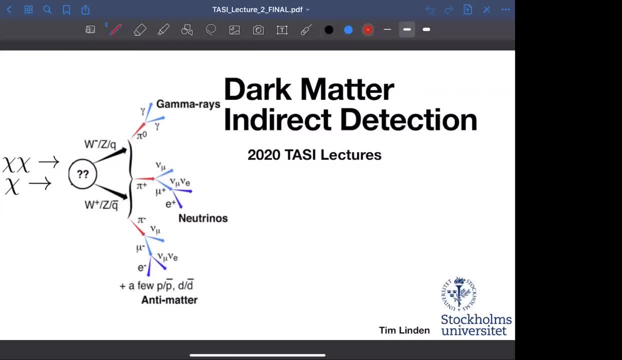 And, as we talked about yesterday, there's an extra lecture today at 3.45 TASI time, and there are no lectures at all tomorrow. We'll remind you of that again at 2 o'clock. So we'll let Tim take it away for his second lecture. 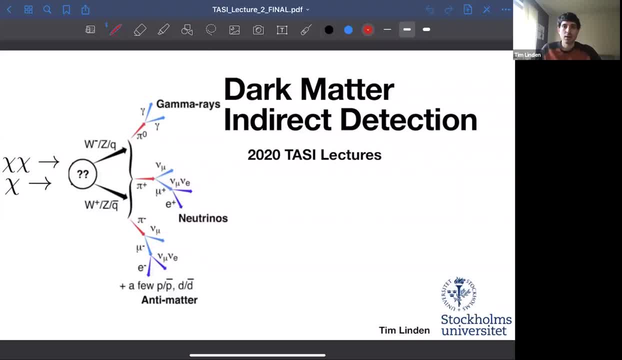 Okay, Thanks for coming by again, And now we're going to go into the second lecture of this three-part series on dark matter in direct detection. So what did we talk about in the last lecture? We went over a few different things. We went over for evidence for dark matter. 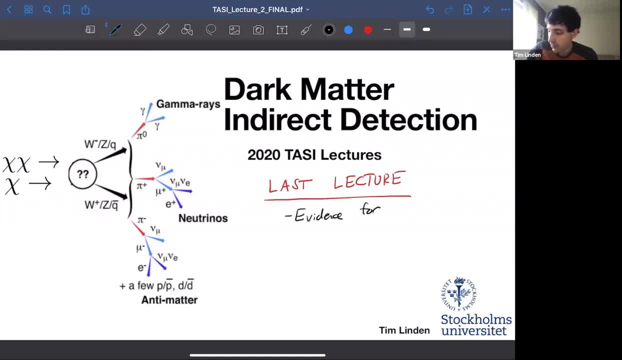 from galactic rotation curves, from the structure of dwarf spheroidal galaxies. That also told us, as a bonus, where is the dark matter. So it gave us a good list of targets. if we wanted to do an indirect detection search, You know what sort of targets we should be looking at. 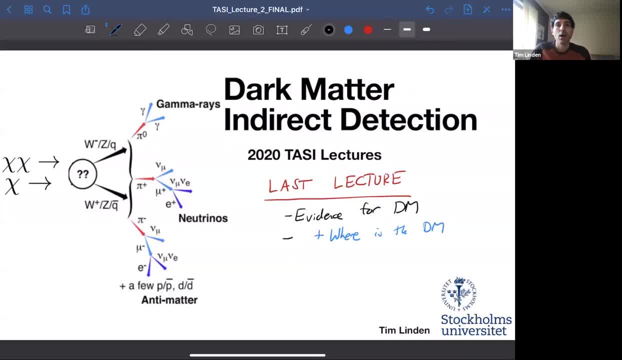 where should we be looking at, what are the profiles of the dark matter in our universe, and so what might be some of the most promising targets? The second thing we talked about is that, in the case of WIMPs, this is potentially detectable. 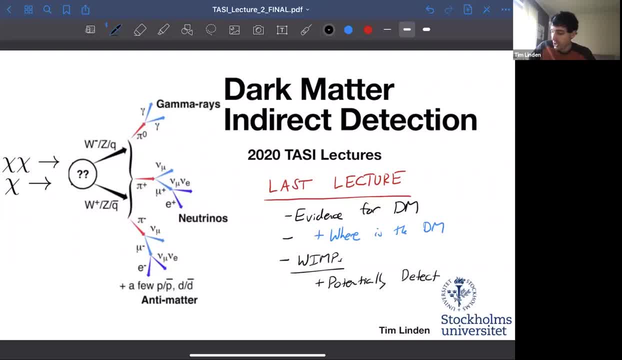 That is, the flux at the thermal annihilation cross-section is large enough that you know this is about what, would we say? a thousand times as bright as the luminosity of the sun, and that is something that we know with astrophysical instruments. 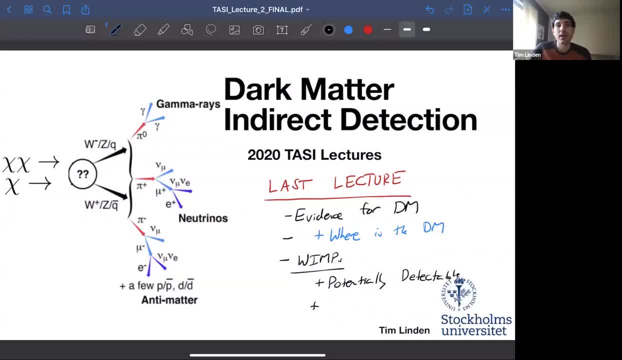 we could potentially detect. And the second thing that's been motivated both by my last lecture but also some of the lectures by Martin is that we're thinking about things at the GEV scale. The thermal WIMP miracle works at scales between- I'm not sure what exactly he said is the lower limit. 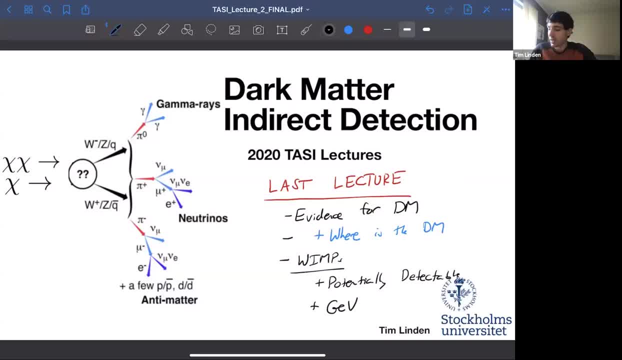 but it's the lower limit of the thermal WIMP: A few GEV, up to 100 TEV or something like that, and in those scales you expect to potentially see emission that can be observed. So we need to now think about the GEV sky. 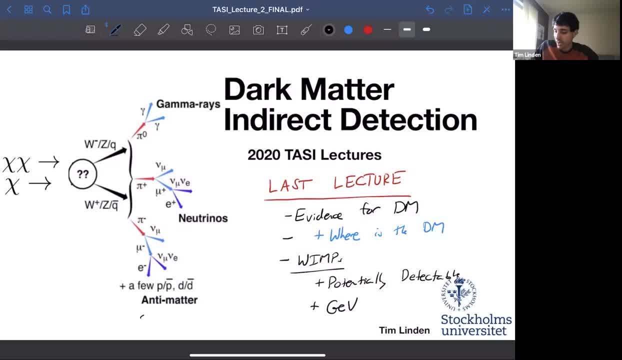 because what we know, the last thing right, is that if we have chi-chi going to two standard model particles, maybe one and it's antiparticle if both of these things are GEV masses or, you know, GEV scale masses. 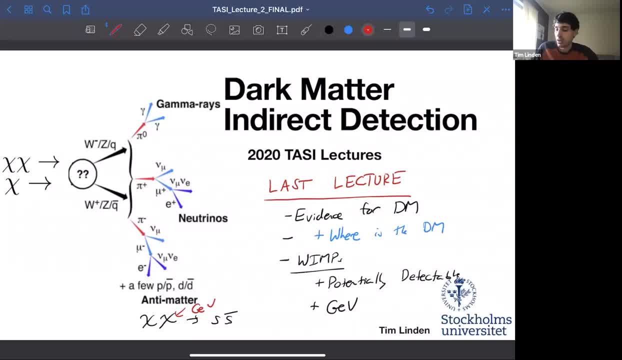 and they're not moving relativistically in the universe, so that most of their energy is just their rest mass, then these things are going to be GEV scale particles too, And maybe these particles are much lighter, but in that case they're going to be relativistic. 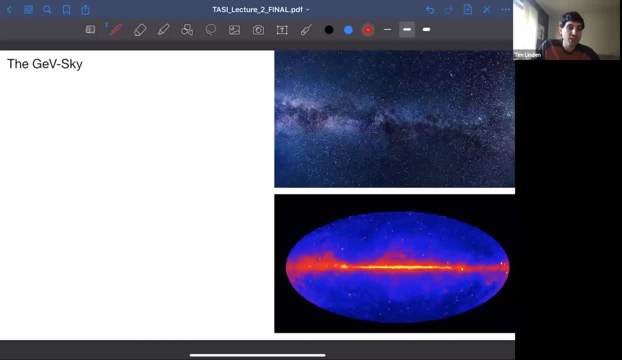 in order to conserve energy. So what does the GEV sky look like? Well, the high energy astrophysics in the GEV sky first I'm going to define for the rest of this lecture is something that is on the order of around 100 MeV. 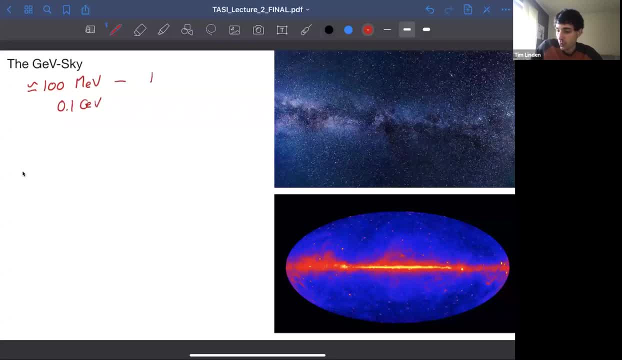 so that's 0.1 GeV up to about 100 TeV, so that is around 10 to the 5 GeV. I'm going to stop there because of unitarity. at the high energies, Of course, gamma ray emission continues infinitely high. 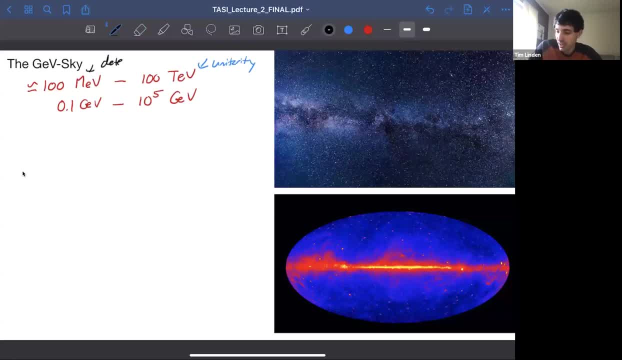 And I'm going to stop here- mostly for detectors, for reasons that might become clear later. So the high energy astrophysics of our universe is unique, So let's think about what we see when we look out in the observable universe. go out at night. 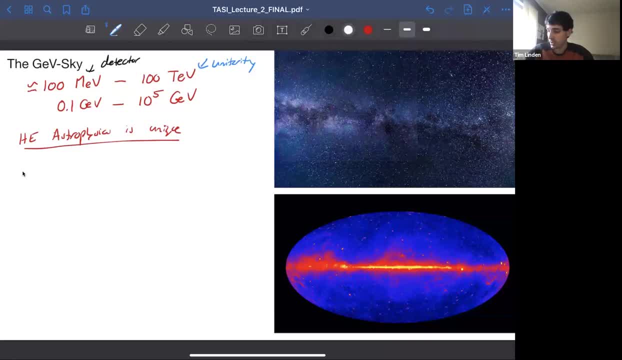 if you happen to be somewhere that is suitably dark at the moment, what you see is a bunch of stars, And then you know you're you're biased. you see a few thousand stars that happen to be close to us. 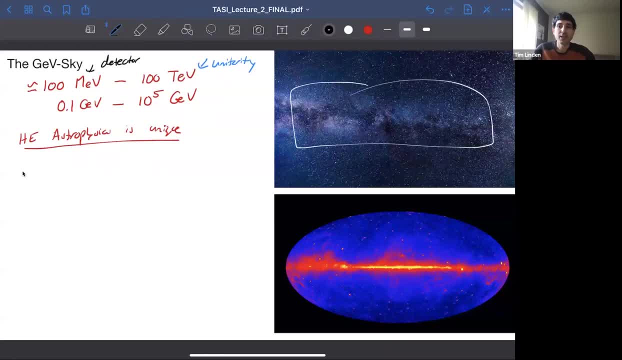 If you look out with a bigger telescope, you see a lot more stars, And so that is maybe what you think of as the dominant source of energy in our universe, And that's the dominant source of, you know, radiation emission we might want to track. 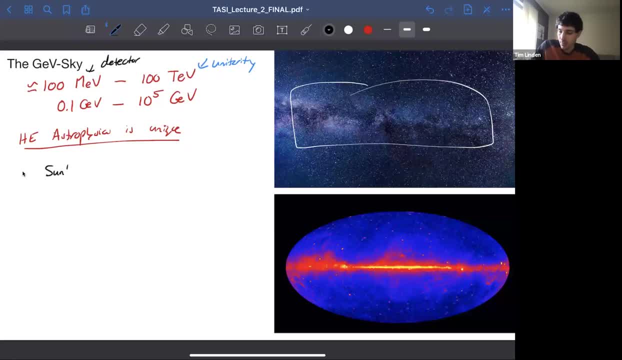 But sunlight, you know, the surface of the sun has a temperature, then that temperature is around 5,000 Kelvin, So it's a black body at the surface of the sun with that sort of temperature And that means that the energy scale. 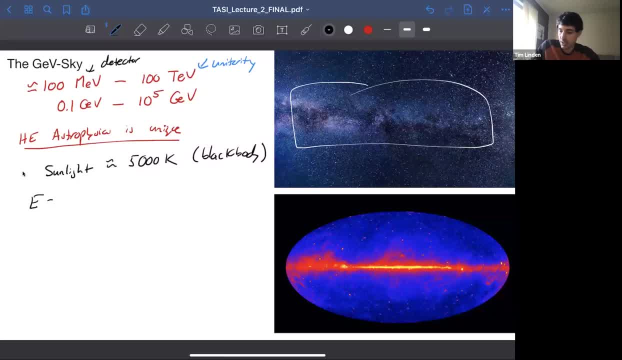 that we're thinking about is around 5,000 Kelvin times the Boltzmann constant, which is 8.6 times 10 to the minus five eV per Kelvin. So the energy scale is around one eV. So that's where for almost any star. 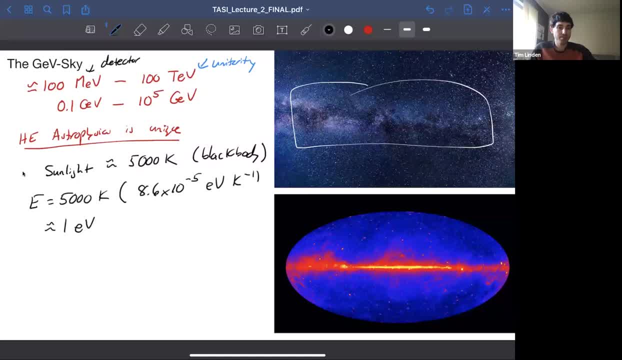 most of the light is emitted at those sorts of temperatures- low plasma temperatures- And they just you know you can do the black body for something with a temperature of 5,000 Kelvin. ask how many GeV gamma rays are produced. 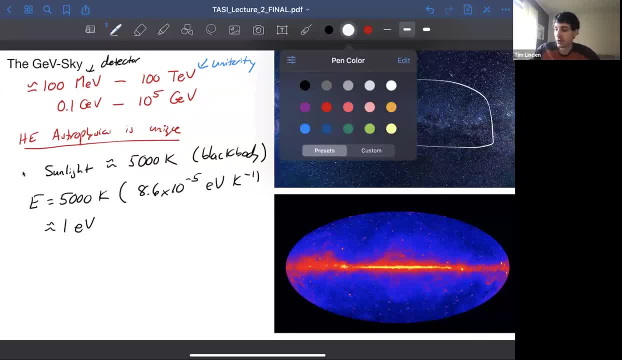 and the answer is zero. If you don't believe me, do that exercise. So what does that, you know, look like when we're looking at, maybe, the GeV sky, compared to the optical sky that we see every day? So what is the luminosity of the Milky Way optically? 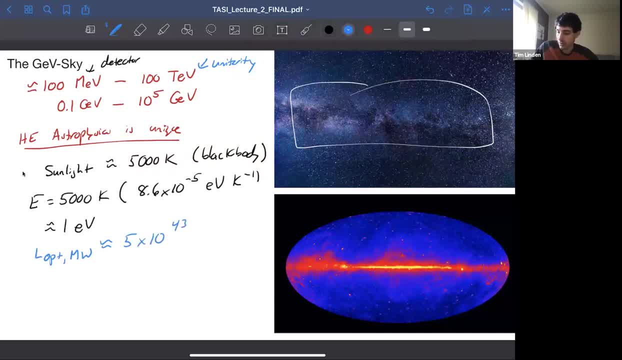 It's around five times 10 to the 43 ergs per second, which is the exact number. So the first is this weird astronomy unit, but the exact number doesn't matter. What is the gamma ray luminosity of the Milky Way? 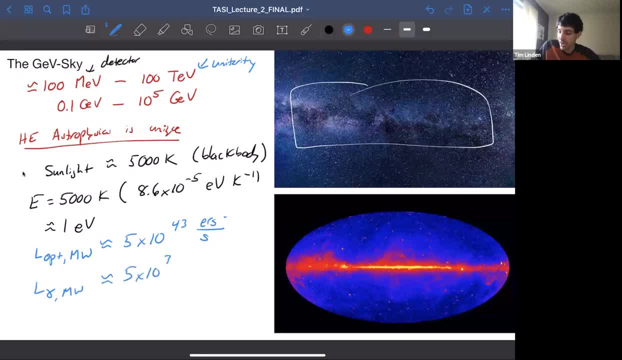 It is around five times 10 to the 38 ergs per second. So most astrophysical sources, most of the emission from the Milky Way, is not a GeV energy. It's in the optical range or maybe even in the far infrared range. 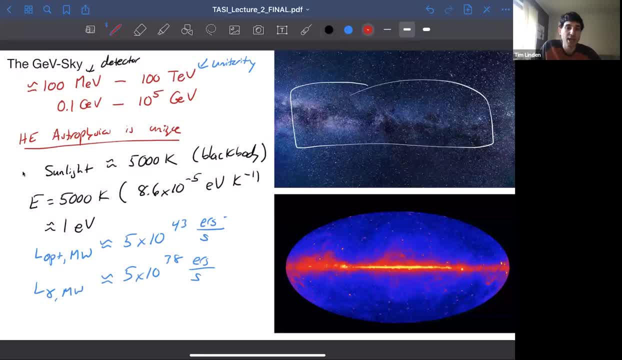 which you can see with different telescopes but which is not gonna affect any of our telescopes. So it's not gonna affect any of our telescopes. So it's not gonna affect any of our dark matter observations. here, Most astrophysical sources are not energetic enough. 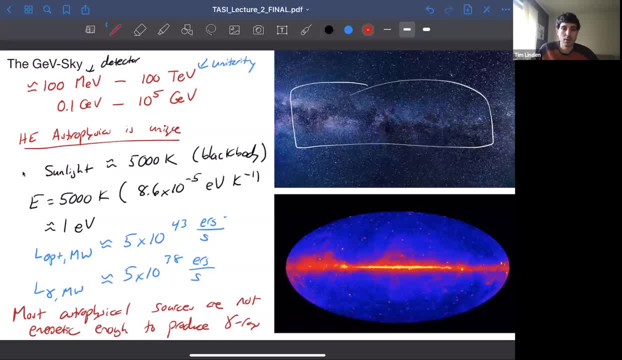 So that means that we're thinking about a very specific class of sources that are not just stars. We're thinking of things that produce, have very high energy scales and produce lots of very high energy emission. So the rest of this talk, which is gonna be only slightly a dark matter talk, 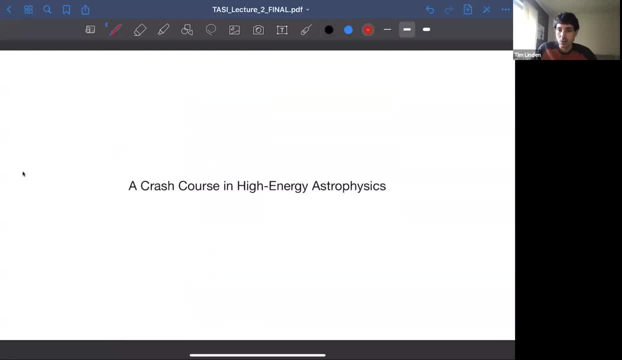 but it's gonna provide a lot of background for what we wanna do. The question is: what determines galactic emission? I think in just a few slides that'll become a lot clearer. So I'll defer that question for a few minutes. So the rest of this talk is gonna be basically: 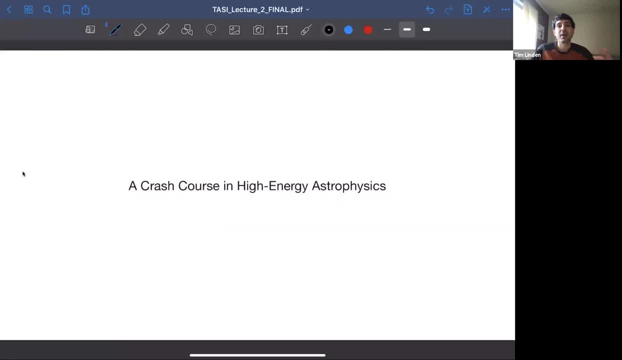 a crash course in high energy astrophysics. What are all of the expectations when we look at the GeV sky from all of the astrophysics that we expect to see? and we're gonna need to somehow subtract that up if we really wanna do any sort of dark matter. 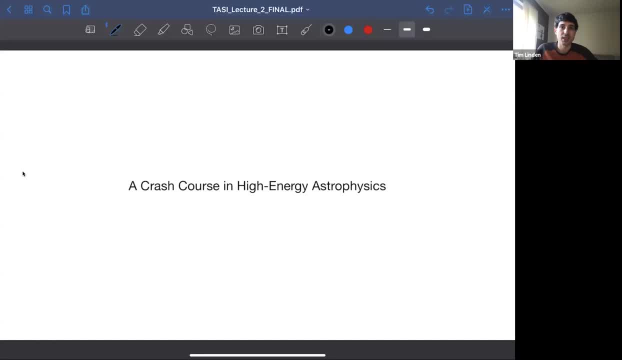 and direct detection. So before we can look for small excesses that might be due to a dark matter signal, we have to have a really good idea of what the GeV sky actually looks like. So what makes high energy emission? You can think like a particle accelerator. 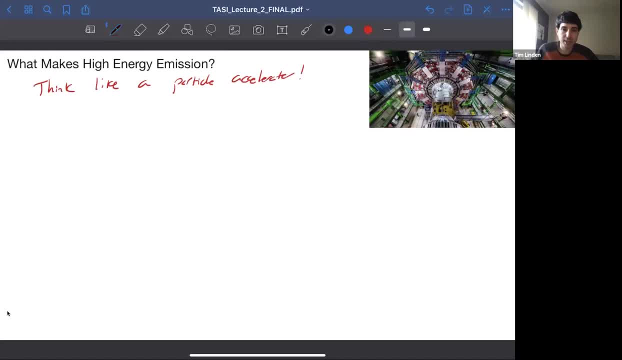 So, basically, whether we stole the idea from the universe or the universe stole the idea from us. but step one is that you use time, variable magnetic fields, to accelerate the particles to high energy. Step two: those particles do something. They can be very powerful. 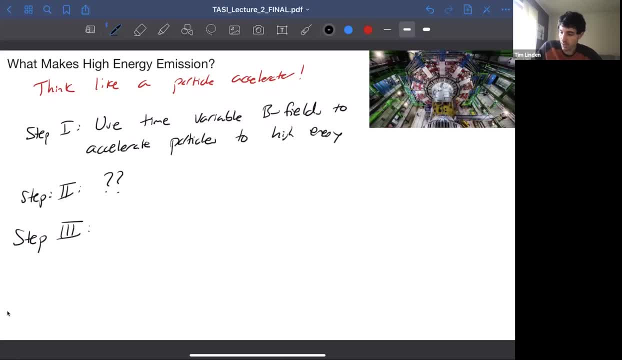 And step three, you have the particles interact with things, And those particles interact with things and they produce a mission that you might be able to see. So what are sorry? what makes? what can we search for? Well, we could search for cosmic rays. 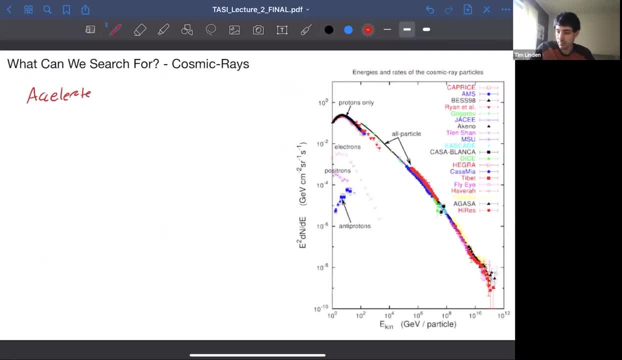 You can accelerate charged particles. So that means you can move things to high energies, And then those particles are gonna, you know, move through the universe or the galaxy. They're eventually going to make it. we might set up an instrument somewhere and that instrument is going to look. 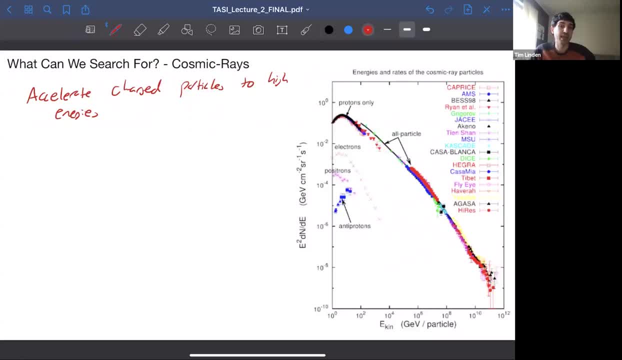 for the high energy particles that hit it. So here is an example of this. This is the kinetic energy of the particles that we're looking for. This is mostly the flux of high energy protons that are hitting it. This is mostly the flux of high energy protons that are hitting it. 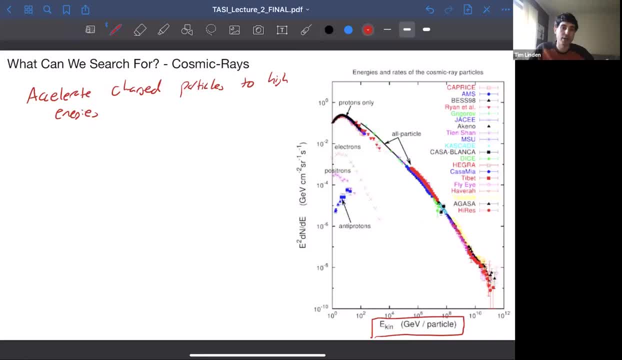 some detector and that detector is either in space or on the Earth, depending on the energy scales. This is over many, many orders of magnitude in energy. This is 1 GeV down here. This is 10 to the 12 GeV up here, which is nearing what we call ultra-high energy, cosmic. 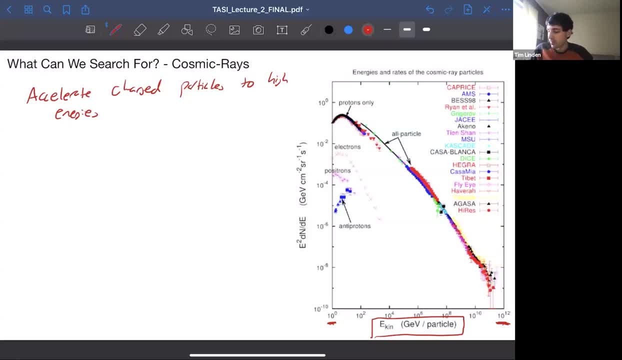 rays. This is in the territory of ultra-high energy cosmic rays at 10 to the 21 EV. This here is a useful unit for astrophysics and really, I think, any physics. E-squared DNDE. E-squared DNDE is very useful because it tells you where the energy actually is in these large 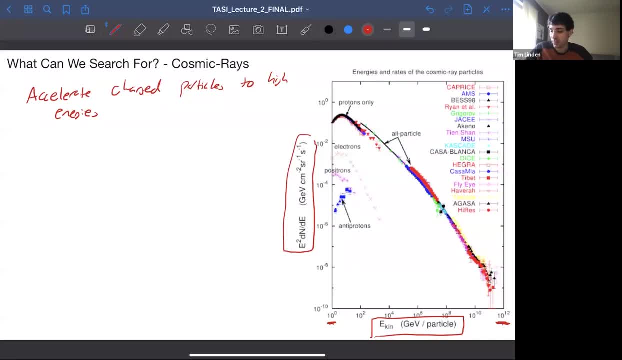 spectra. DNDE is a differential spectrum, so it has units of inverse energy. but then you multiply by E-squared so that the units are, say, GeV per cubic centimeter, or sorry, per square centimeter, because it's hitting some detector Per second is kind of obvious. 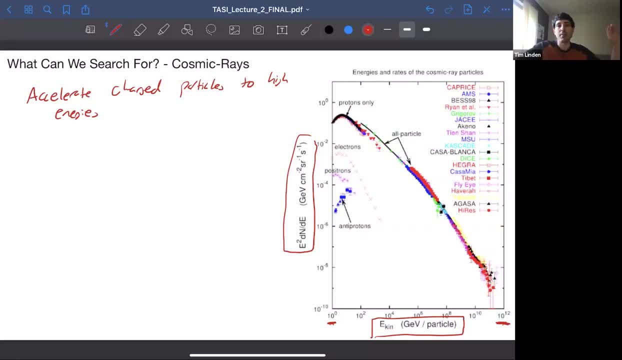 How long did your detector sit there? Then per steradian, and then maybe you look out of the whole universe, or something like that. This gives you an energy scale. This tells you where the energy of the universe is actually high and where it's low. Here's the spectrum of protons. 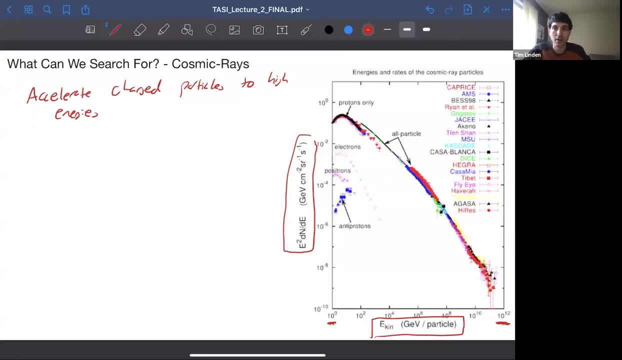 You can see now this is a very smooth power law over many, many scales in energy. Here we're approaching the proton rest mass itself at about 1 GeV. so you're seeing some sort of a turnover in the kinetic energy of particles you can produce. but then you 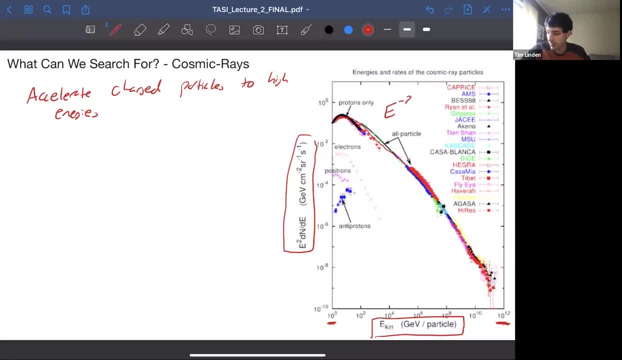 see something that is roughly E to the minus 2.7.. That's maybe a number worth knowing. Then E-squared DNDE, that makes it E to the minus 0.7.. DNDE is a proportion of E to the minus 2.7. 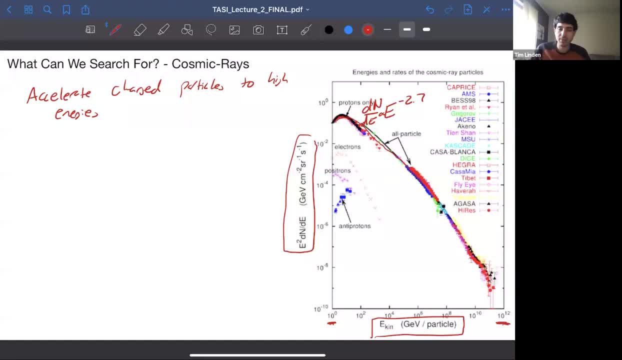 over many, many orders of magnitude. That's something you can look for Higher energies here. you might not be able to tell the difference between protons and everything else anymore. The answer is these are mostly still protons, but maybe we just 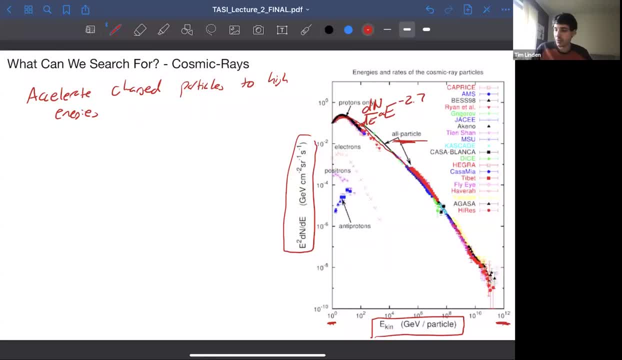 add everything together. That's one thing we could look for. We can look for, maybe, protons. that way, We can look for electrons. We can look for nuclei- where nuclei include things like carbon and helium are important, and literally all the other ones as well. Also, we can look for all the 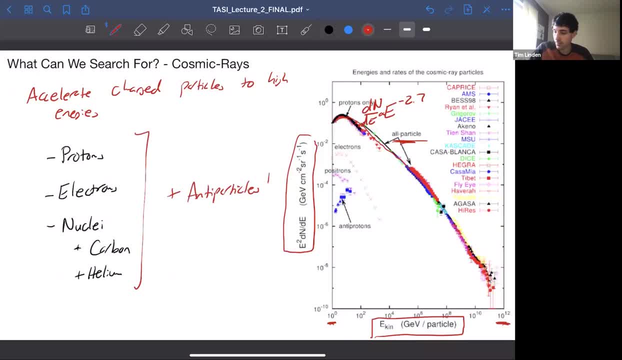 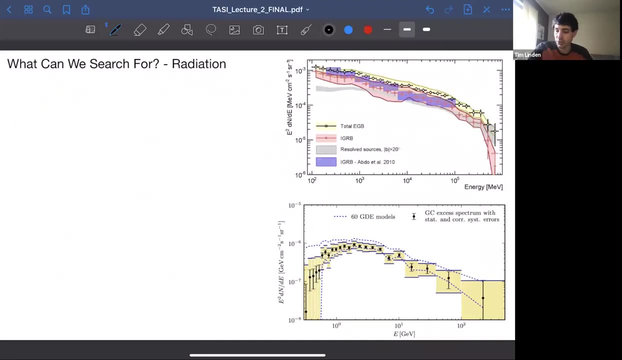 antiparticles. We can't look for neutrons. Neutrons decay while they travel through the galaxy. What else can we search for? We can search for radiation. Here we look at what do the charged particles produce? They might produce, for instance, gamma rays. 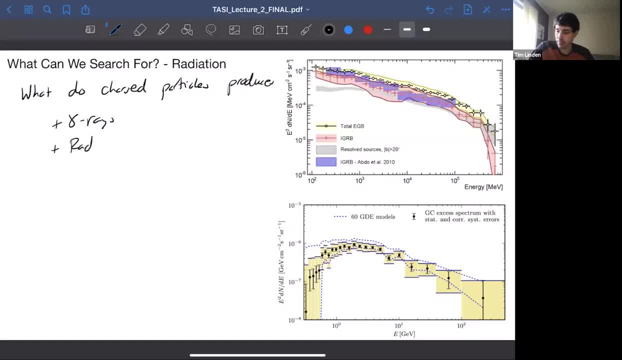 They might produce radioactivity, They might produce radioemission, They might produce neutrinos which would also travel directly to us in straight lines. Here are some spectra of gamma rays. Here again, E squared DNDE. Now the energy scale is set by the Fermi instrument that's measuring these. 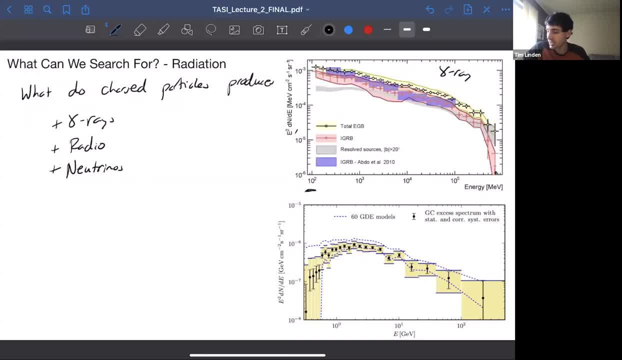 100 MeV up to 10, to the 6,, 100 GeV or something like that. Then here is, this is the integrated gamma rays over the entire extragalactic space. you just subtract, You can take off the Milky Way and look at everything else that's there. 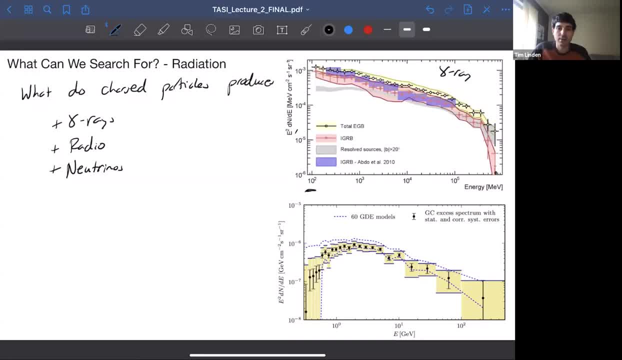 And then this is the galactic center excess. The details aren't important here, But what are some of the important things that actually make these sorts of gamma rays? The first thing is pi zero decay. So this is when a high energy proton comes in. It's moving relativistically. It strikes some, some gas atom in space, maybe a hydrogen atom, maybe a helium atom, maybe just the nuclei of those things. This is a high energy particle collision and you probably know how these go. It produces jets, produces a bunch of other stuff and maybe in one of those jets is, say, a pi zero. 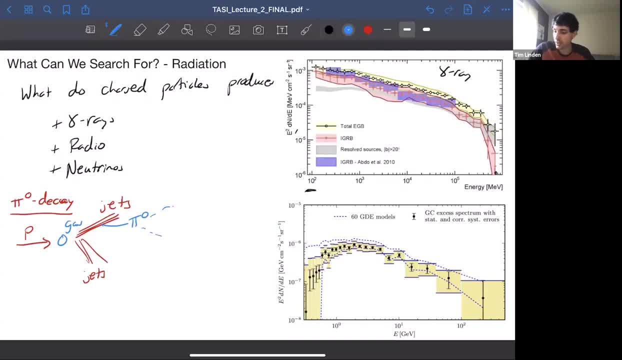 Pi zero comes out in these jets and the pi zero very, very quickly decays into gamma, gamma And the energy scale between, you know, this proton and the gammas that you see is calculable. I mean, this can be done in collider physics, it can be done, you know, in beamed up experiments. whatever you know you could, you can also do it analytically. 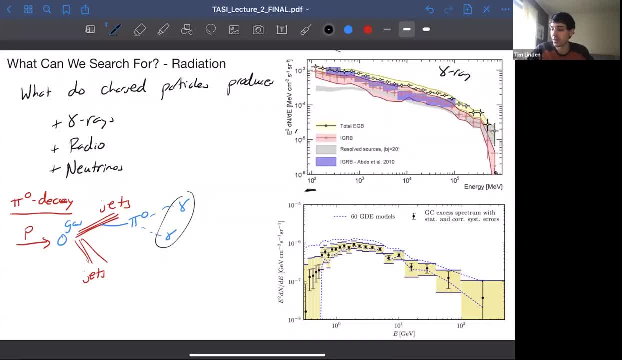 And so you can calculate, for high energy protons coming in, what the gamma ray energy coming out is. A second important thing is inverse Compton scattering, which is not spelled anywhere like that. This is the inverse of Compton scattering, as the name might suggest, which might be a process you're familiar with. 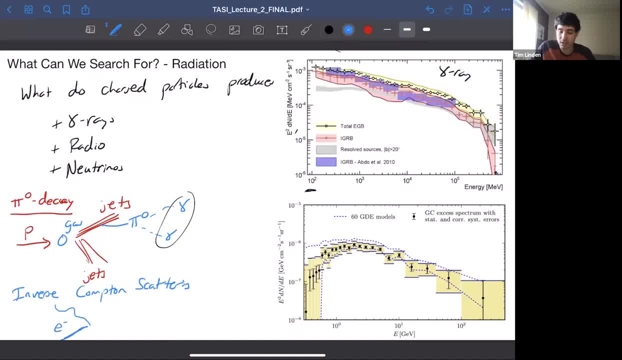 So a high energy electron comes in the electrons moving relativistically because it was accelerated in some electromagnetic field. It hits some photon and then these things just scatter off of each other and they go their very ways, except now in the lab frame. 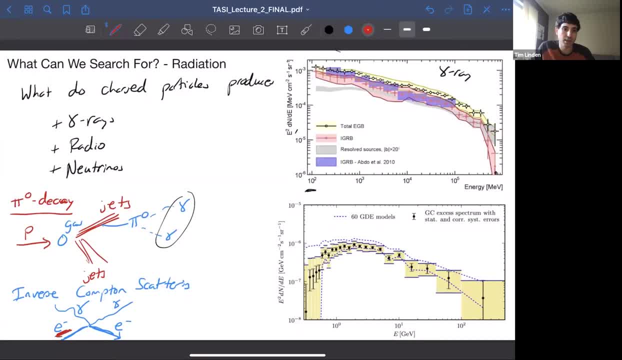 this was very high energy and moving relativistically. This is where it's the inverse of normal Compton scattering. In normal Compton scattering, this comes in with a lot of energy and accelerates the electron. In inverse Compton scattering, the electron in the lab frame comes in with a lot of energy. And then this is some soft photon. This is maybe starlight. 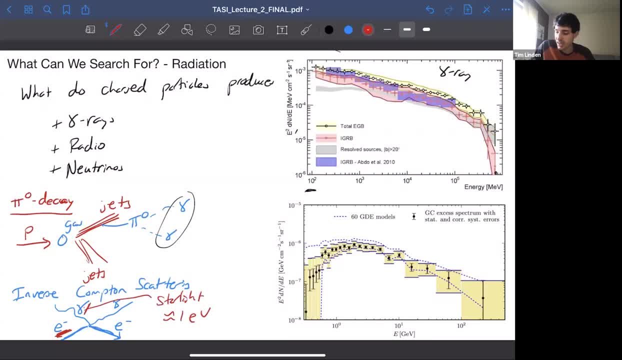 In starlight. we said the energy is around 1 eV, And then so this electron loses its energy and it produces a gamma ray out of this sort of emission. And then you can also have some attribution from Brems-Scherlong. 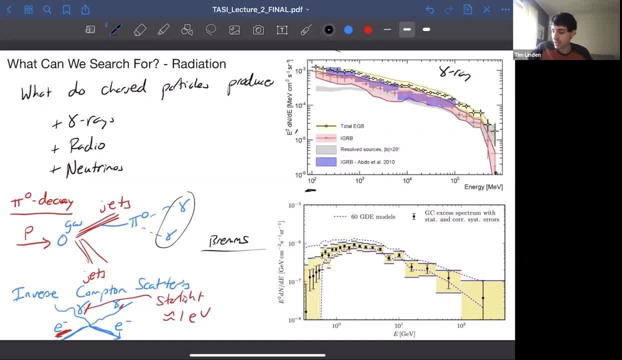 which I'm not going to try to spell because I'll fail. but an electron comes in and scatters off the outside of a molecular gas nucleus, Right. so electron comes in here, it changes its path after some impact parameter, with the nucleus here and some e minus cloud there, and that produces, as it changes its path, some sort of gamma ray emission that you might see. That's usually subdominant. 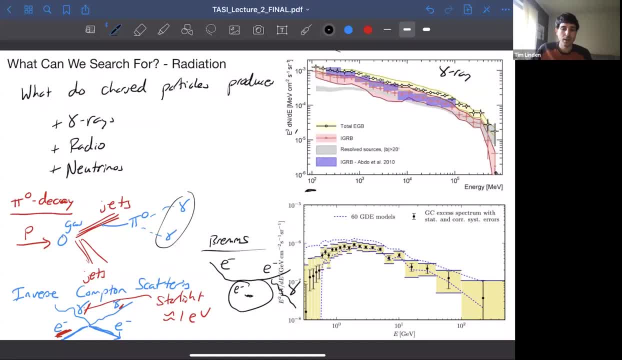 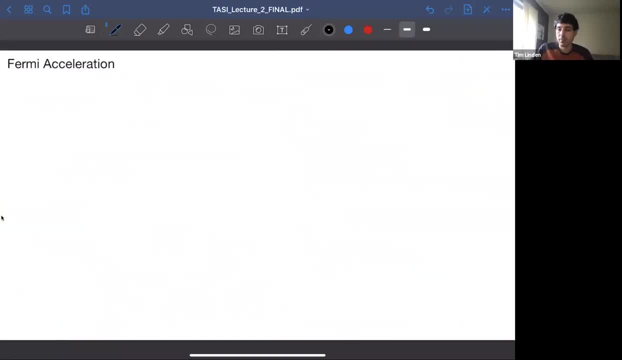 Okay, so that's the other signals we could search for. Now how do we get the high energy particles? Let's go into a little bit more detail here. In an accelerator experiment you get to tune. you know exactly how do the magnetic fields in your accelerator changes a function of time. you get to plan out exactly the cadence of these things. you get to track the particles going through. you know, basically optimize the problem. 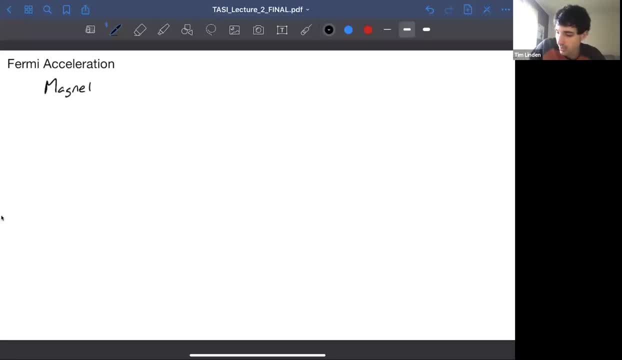 And you know the same principles hold. The magnetic fields can't do work. So what you need is some sort of time variable magnetic field so that you get e does not equal zero in order to accelerate the particles. So there are two types of what we call Fermi acceleration that produces high energy particles in space. Because there are two, we have aptly named them. first order: 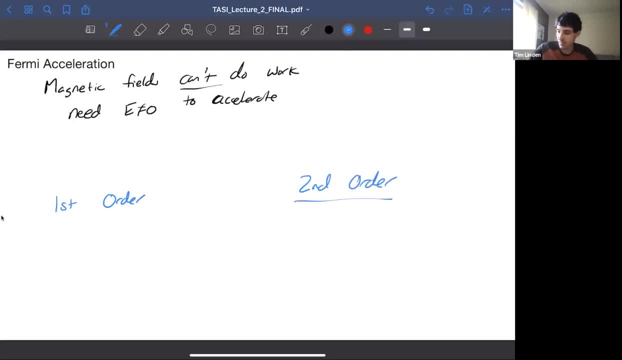 And second order. First order: Fermi acceleration is any scenario where the average e field over some region is not equal zero. So this would be an example, like a unipolar inductor, A shock front, where maybe you're only considering what's happening exactly on the shock and you know there's some electromagnetic field moving out from some sort of explosion. Second order is the scenario where 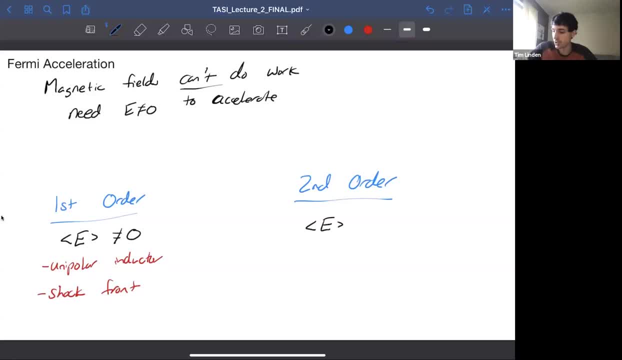 the average electric field over some reason acceleration region. it does equal zero, But it has some sort of uncertainty where the variance in that magnetic field does not equal zero. So there are positive and negative acceleration regions that you have to worry about And what we'll see is that you still get a net acceleration from that sort of scenario. So this happens in molecular clouds. 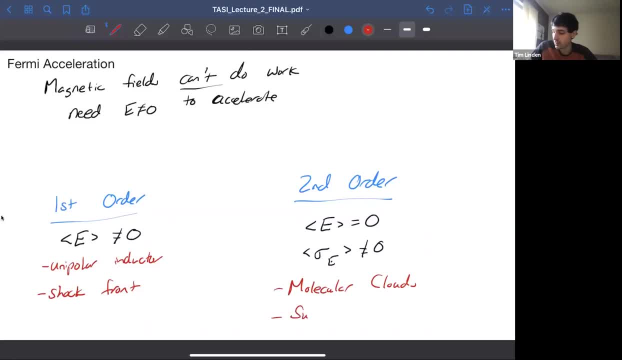 Which we'll talk about in some detail. This happens in supernova remnants. This is actually the primary acceleration mechanism, is second order. So a schematic detail of what is first order Fermi acceleration. You can imagine that you have two reflective plates or something like that and they are moving towards each other and they both have a velocity v. 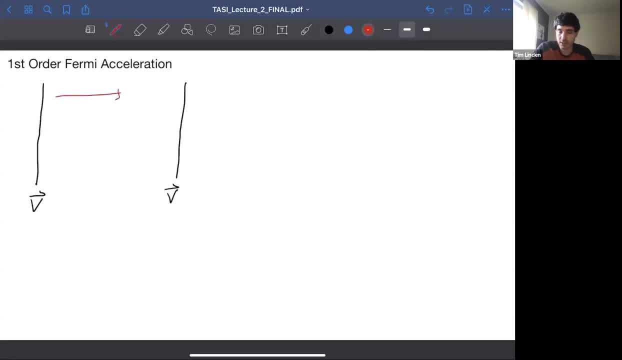 And you have a particle that is bouncing back and forth between these two things with a velocity u And then it is bouncing off and then it's coming back with some velocity u. prime, This could be the trash compactor on the Death Star. could be two players running towards each other with ping pong rackets. 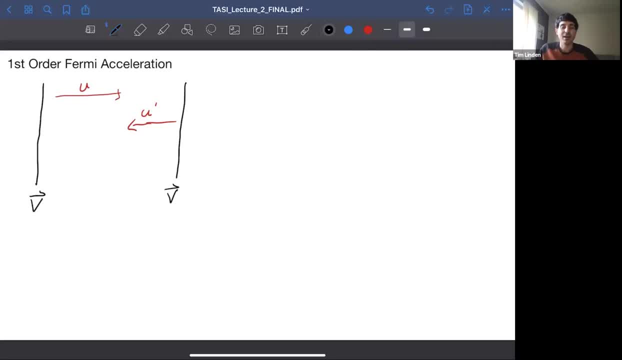 bouncing something back and forth. if you wanted different classical mechanics definitions or you know, this could just be some strong magnetic field region that the particle can't penetrate. So it's just bouncing back and forth between these. So we're going to assume spelling is not my strong suit today, Assume. 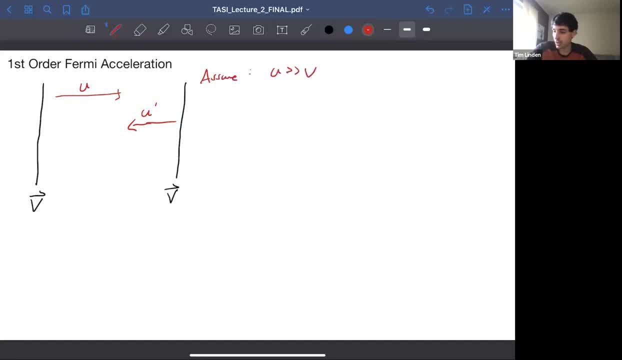 u is much, much greater than v And in fact u is around the speed of light. So this is basically a relativistic problem. And then you say: what is the change in the energy of the particle? The last thing you're going to assume is that these plates are huge and the particle is small, so nothing happens to the plates as they're moving towards each other. 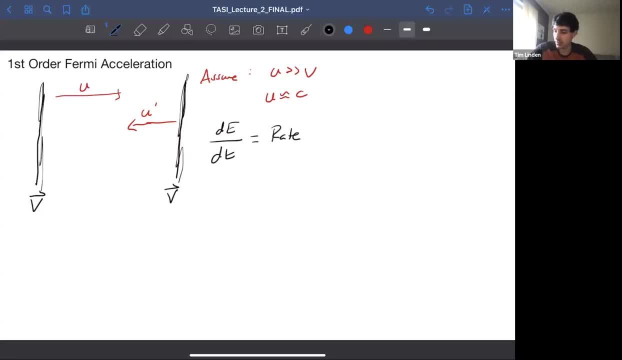 So de dt is the rate of collisions times, how much energy you get per collision. That's, I guess, relatively self explanatory. Delta e of the collision, if we assume this is relativistic, is: delta e is around gamma, m, v, c, which is the velocity of these plates. 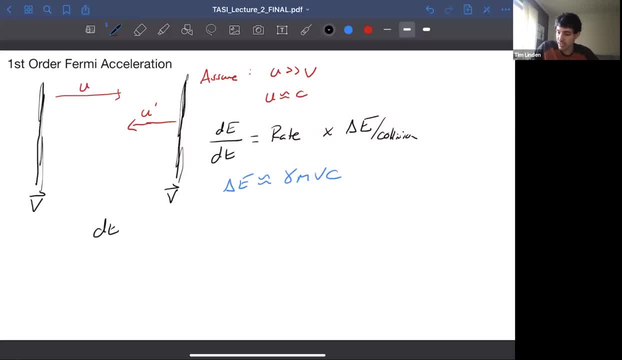 And that's what's going to be added to the particle. So then, dE, dt for the particle is approximately the rate, which is u, the velocity of the particle over L, the distance between the two plates, which I did not specify. L there times gamma mvc, And this is approximately now, if I take u to be. 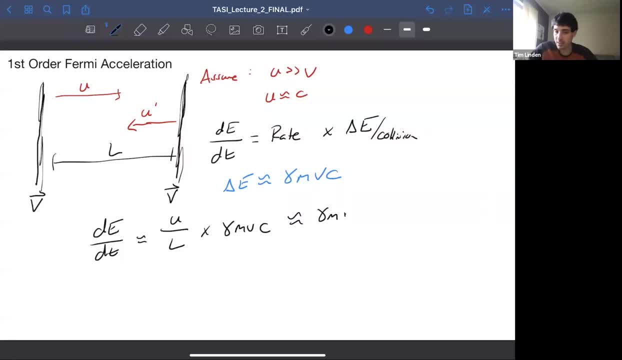 approximately c. this is approximately gamma mvc squared over L. Good, And what this tells you is dE, dt or sorry, gamma mv, gamma mc squared, where m is the particle is equal to e, and then I have v here. so this is e times the velocity of the plates over L. 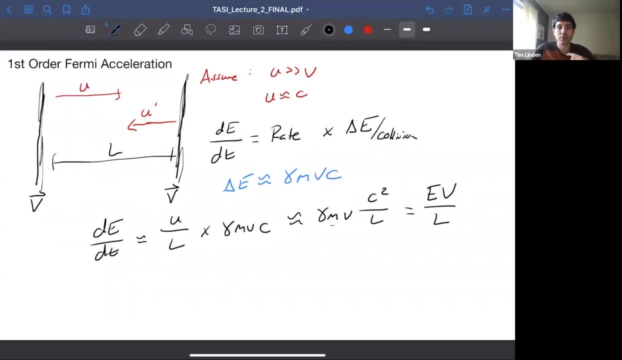 V is the velocity of the two plates that are moving towards each other. So I guess one has positive v and one has minus v in this scenario, or one has v and one has zero, I guess, and then you just change your reference frame. Okay, what's important about this, right? 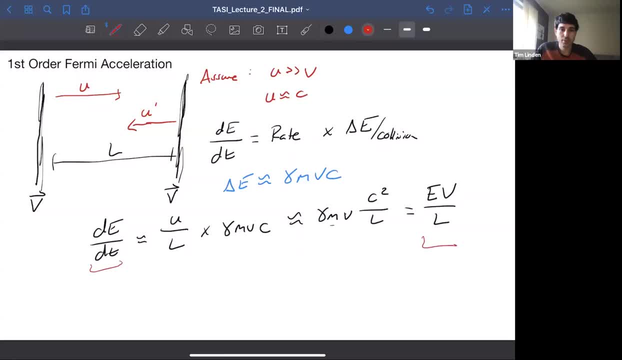 is that this is d e d t and it depends on e right, which means that a very small change, which means, I guess you know d e d t is in some ways proportional to e over tau, where tau is some time scale, that this is operating over Small changes. 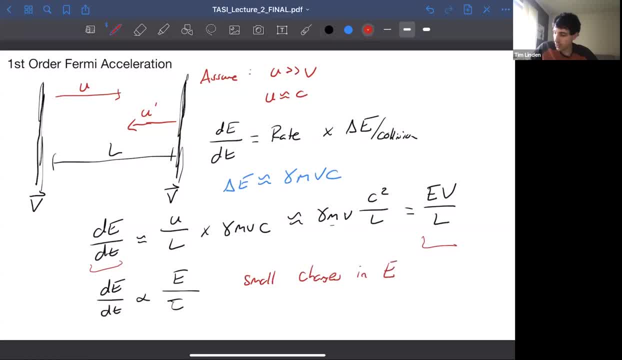 in e zero lead to large changes in e final right. So if I start with just a bunch of particles that are at very low energies and you know some distribution of thermal energies, or they actually have to be slightly above thermal, which is its own problem, I guess the 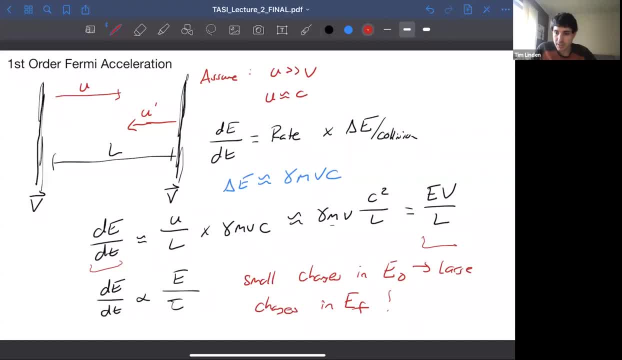 you know- I think that was a response to the last question- Yes, gamma mc squared equals e exactly, And v is the velocity of the plates. and then we assumed u is approximately c, which is how we got that extra factor of c in there. 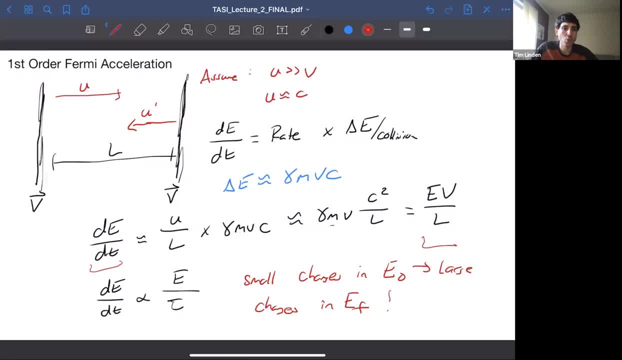 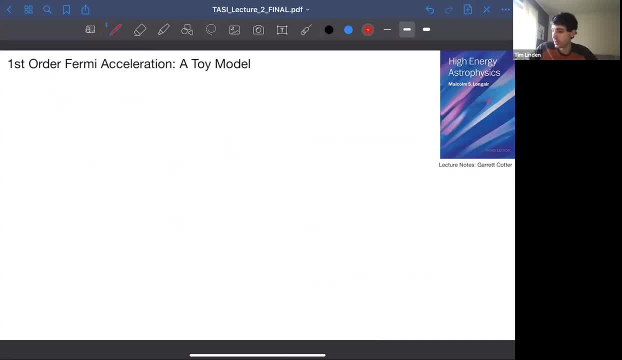 Good. So this is going to lead to some distribution that's relatively wide in the energies of the particles themselves. So there's a. I'm going to use a toy model here. The toy model comes from some nice lecture notes by Garrett Cotter. If you really want. 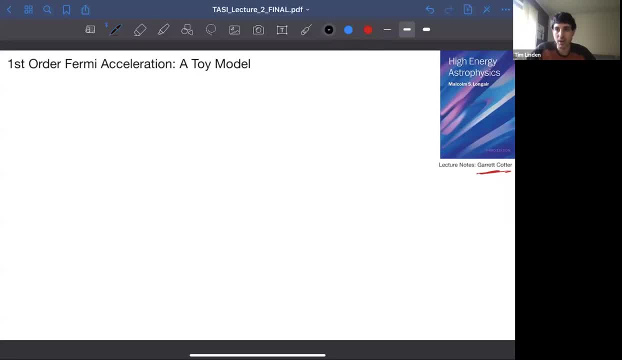 if you want a detailed dive, I recommend the Long-Air book, which is kind of the bible of high energy astrophysics. There's also lecture notes you can find online from Pasquale Blasi. Those are quite detailed. Blasi goes through quite a bit everything and you will. you will learn everything He does. assume that you have memorized Jackson as a precondition of learning anything from his notes. 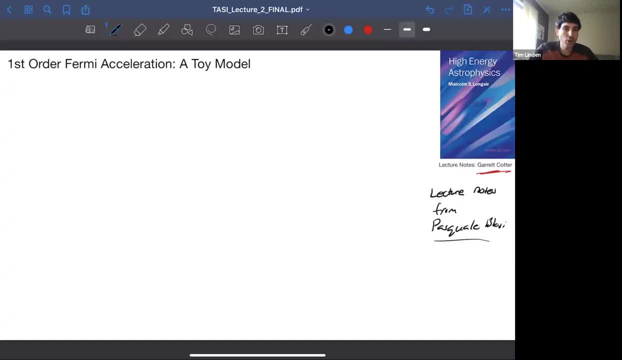 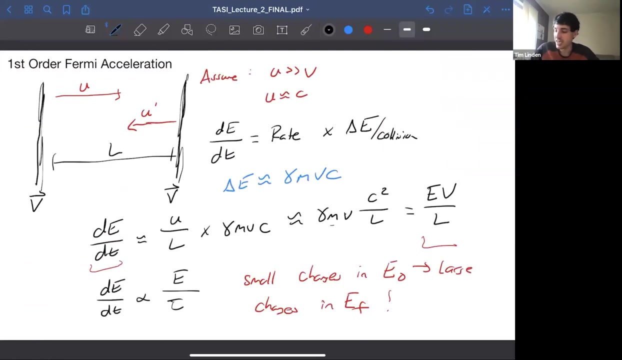 Anyway. so a toy model. So let's assume there are some n crossings with e to the n plus one over e to the n, equals beta. just some energy gain that I get every time I do a crossing Note that is different than the dE. dt equals e over tau. 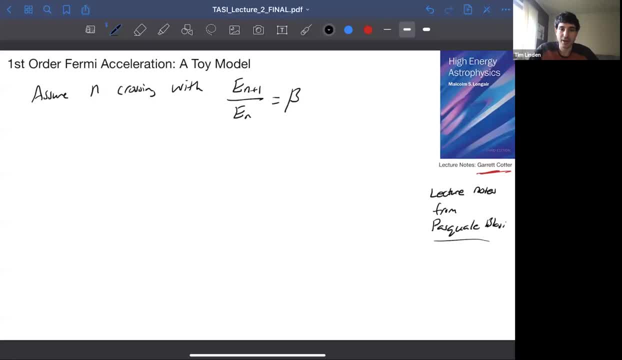 It turns out that that doesn't change the final answer for this very simple toy model. In that case, e final is equal to e initial times, beta to the n power how many crossings there are, and also assume each crossing provides some chance of escape, So the particle might just bounce in the wrong direction, The person hitting the ball with the racket might miss, and then you're done. 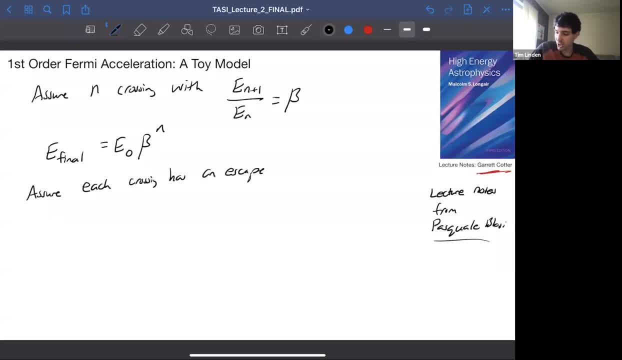 E is an escape chance of p zero, less than p, less than 1.. In that case, n final, the number of particles that are there at the end is equal to n zero, p to the n. Take the log of both of these and set them equal to zero. 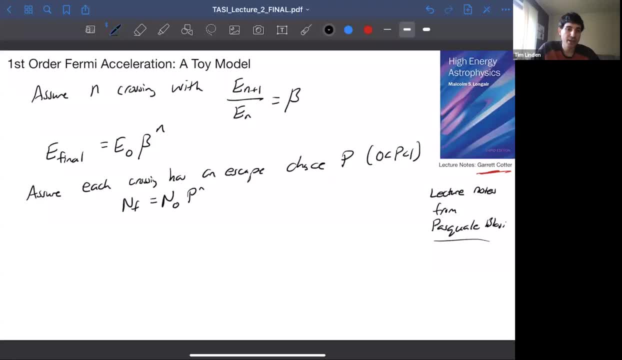 so n final minus an initial, and then take the logarithm and then do that for both sides. you can calculate that the lan of e final minus natural log e initial minus n natural log of beta equals zero, equals the natural log of n final minus the natural log of n zero minus n the 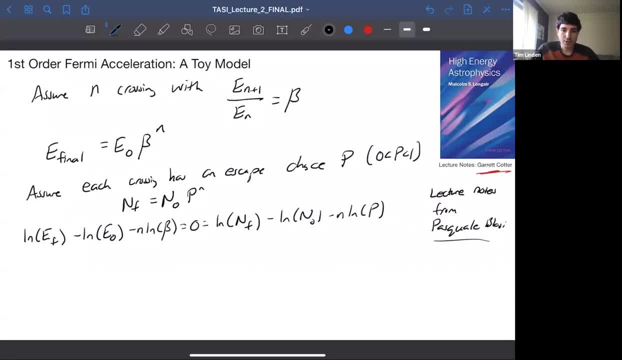 natural log of p, And then you can set these equal to each other and move some terms from one side to the other. move the final terms to one side, move the initial terms to one side and you get the natural log of n- final over an initial divided by the natural log of e, final. 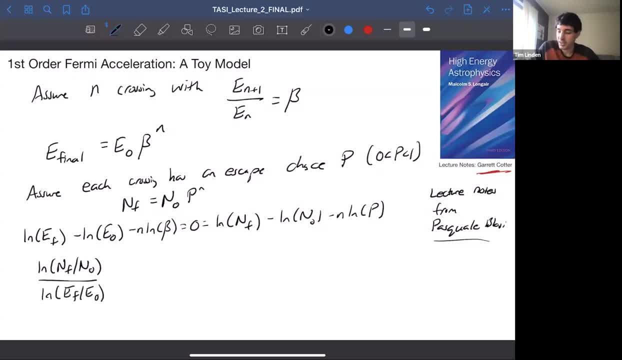 over e initial. so how many particles are there as a function of final energy at the end is equal to n over n. the number of crossings cancel natural log of p over natural log of beta And that leads to n over n. zero equals e over e zero. to the power of lan p over lan e. 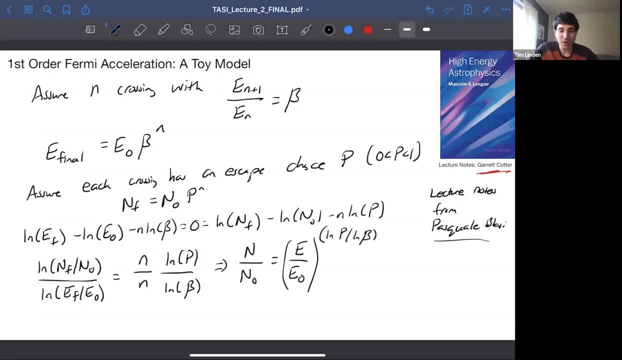 I'll just put parentheses there to make that even. And if you then take the differential form of this, instead of deriving it out by n zeros, you find that d n, d e is proportional to some constant times e. you lose one power here: p over n, beta minus one. 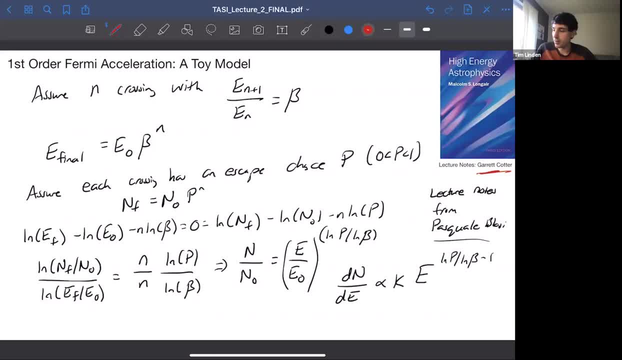 And it turns out that if you do the careful calculation which is given in the long error book, which I'm not doing here, you can calculate that in first order Fermi acceleration lan p over natural log b equals minus one as well. So this is going to be d n, d e. 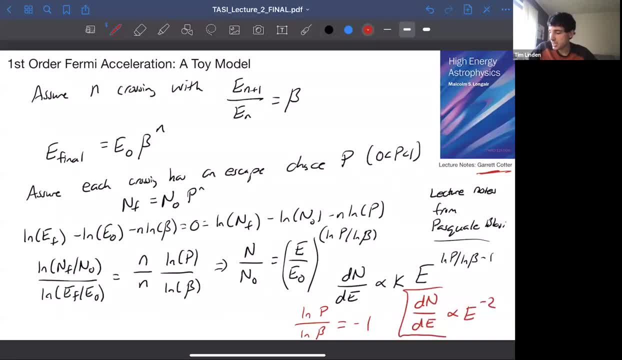 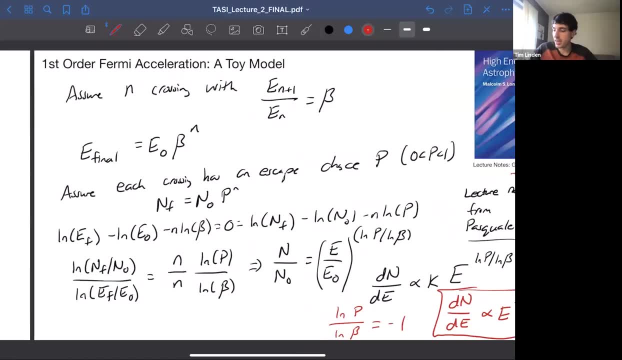 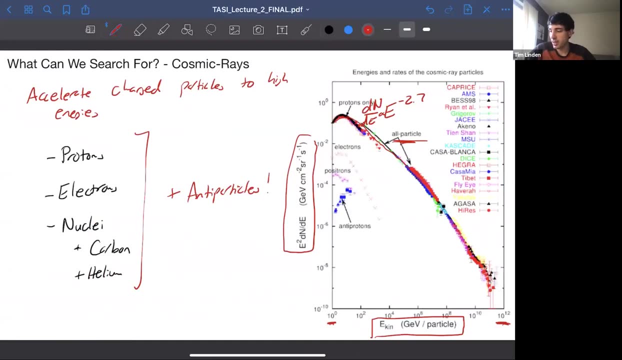 is proportional to e to the minus two And that is a standard result in high energy astrophysics And it's very similar. we went back a couple slides- I'm sorry if you're flipping through sides too fast- to the proton spectrum that's observed, which is e to the d n d, e equals e to. 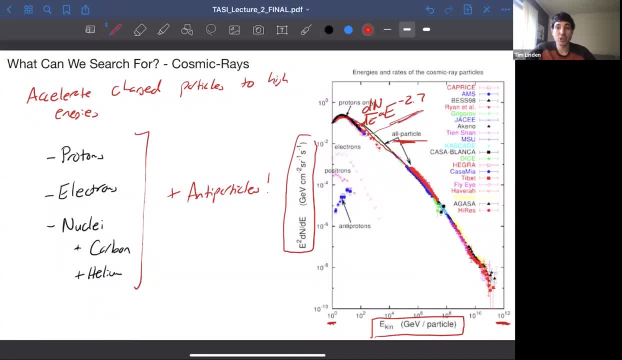 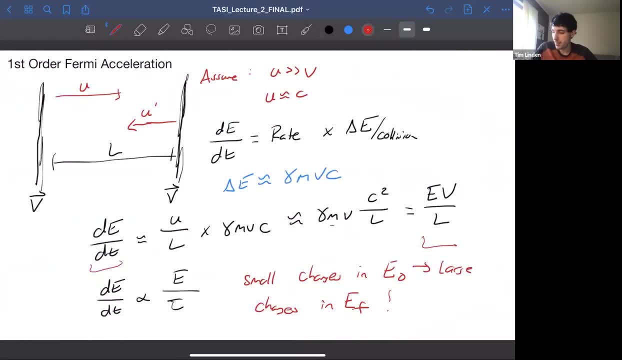 the minus 2.7.. So you get e to the minus two from the injection, from first order Fermi acceleration, and later in this talk we're going to realize where the minus 0.7 comes from. Okay, what is second order Fermi acceleration? Second order Fermi acceleration. I'm just going. 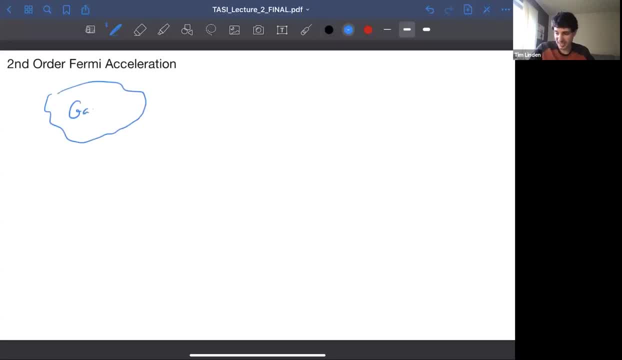 to sketch out pictorially here. So I have a bunch of gas clouds. They are floating through the universe. This is my artistic. this is really kind of the limit of me as an artist. So they are scrolling here at various random directions. 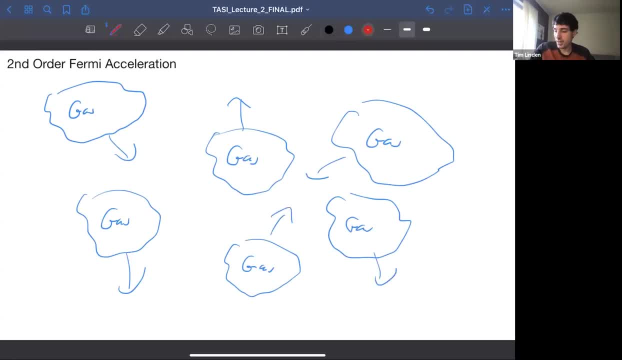 Okay, I'm pretty happy with that. And then I have some particle and the particle bounces off this and it bounces off this and bounces off this and it goes in some random orientation. I don't know why I turned it there, Okay, so it's bouncing off all of these gas clouds. Sometimes it hits a cloud. 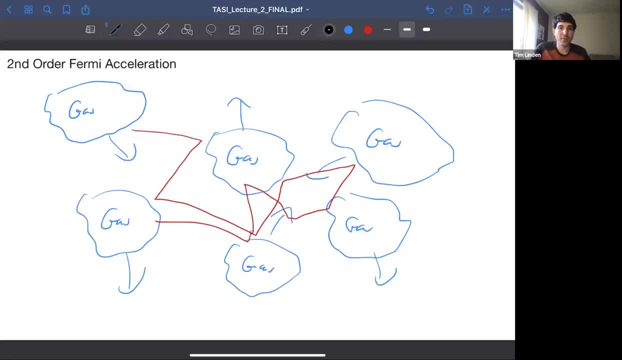 that was approaching it. and when it hits a cloud that was approaching it from the previous discussion- it gains energy, right, But it might also hit a cloud that's receding from it with some velocity and in that case it loses energy. The point of this: 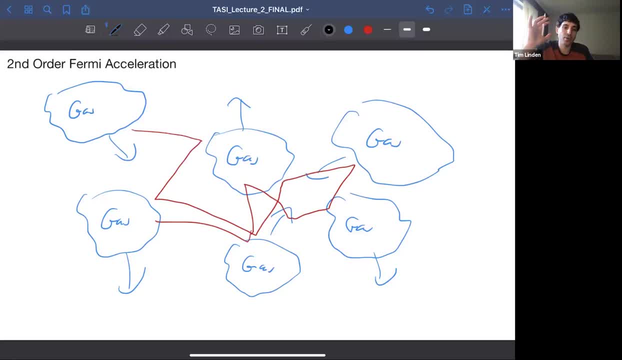 the fear that you have of having to be around the source in this example is: it doesn't really matter. one explosion take place in your field is really important. So I'm going to tell you a shorter story, right? So let me show you how that story is. 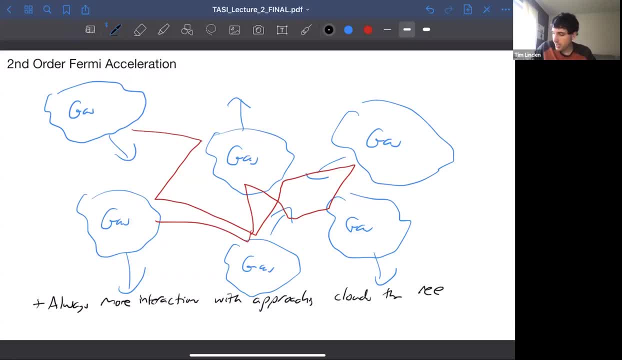 So how the story is right. if I have a billion clouds and the clouds are moving in random directions, At the end there are always more interactions with approaching clouds. feel totally unsafe and you'll find that still there's more oncoming cars in the 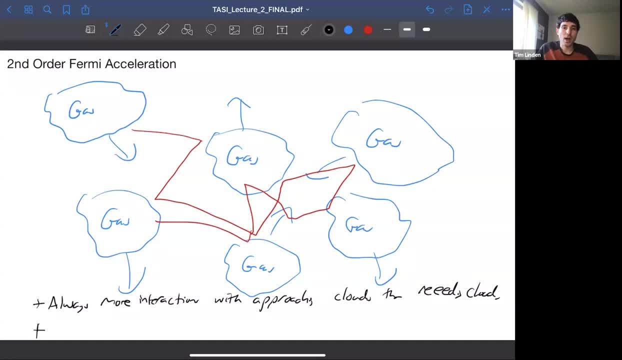 other lane than there are cars that you pass in your lane just because of the relative velocities. so you have many more chances for unfortunate collisions with those oncoming cars. But because there are both, you know ways to gain energy and lose energy. the energy gain is second order, is second order. second: 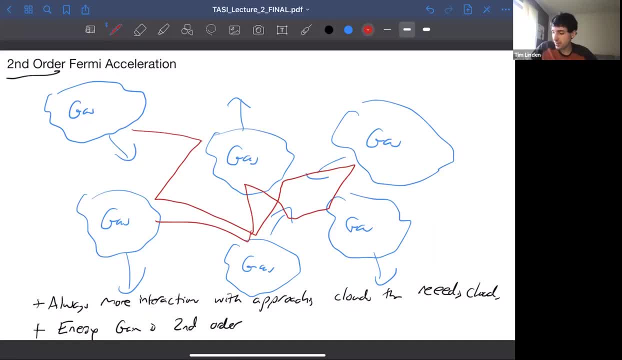 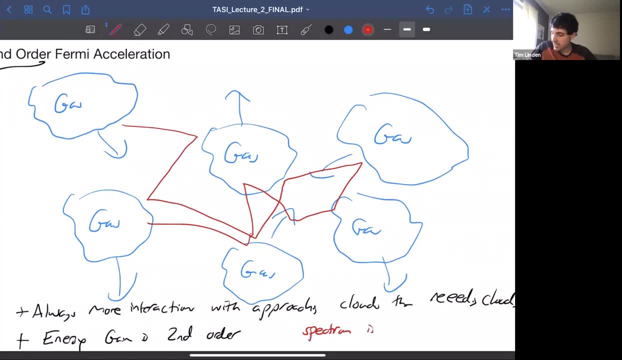 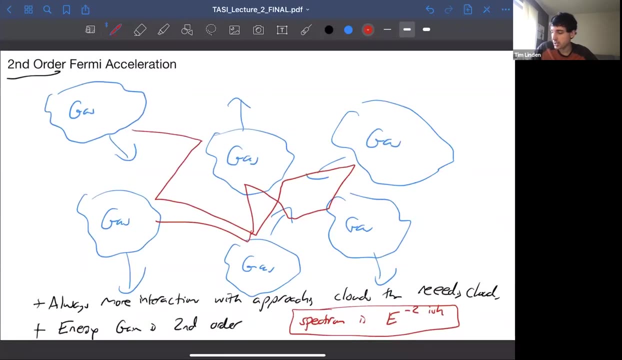 order from the acceleration, The spectrum that you get out of this calculation if you do it carefully- we're not going to do that here- is e to the minus 2-ish, and it depends on the configuration of the clouds and the bouncing conditions and things like that, and it's usually more effectively e to 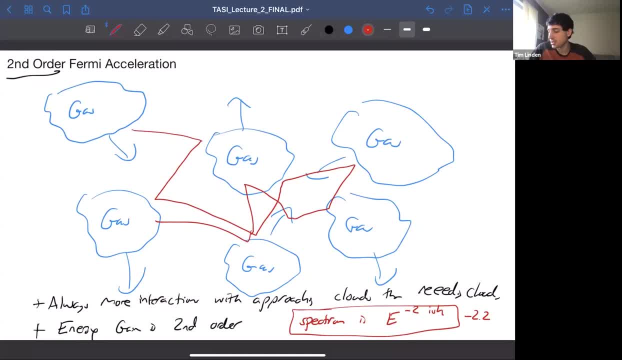 the minus 2.2 or something like that. so that gets us partway to our e to the minus 2.7.. The last thing I wanted to talk about is the energy gain. So if you're going to be driving a car, you're going to want to. 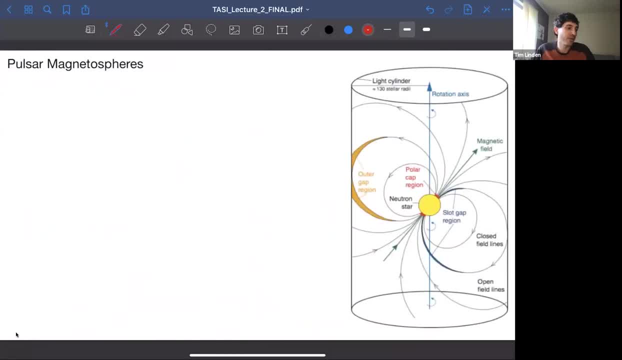 remember that the energy gain is a constant. So I'm going to go ahead and talk about that. So you know, the energy gain is a constant. So if you're driving a car, you're going to want to remember that the energy gain is a. 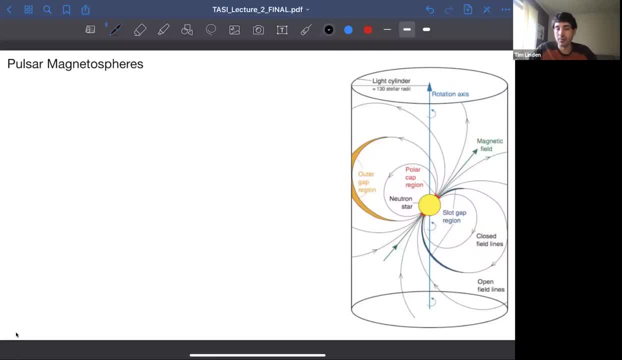 constant. So you know, that's one of the things I wanted to talk about. The last thing I wanted to talk about is pulsar magnetospheres, and there are two reasons I wanted to mention them in this lecture. The first is because they're the 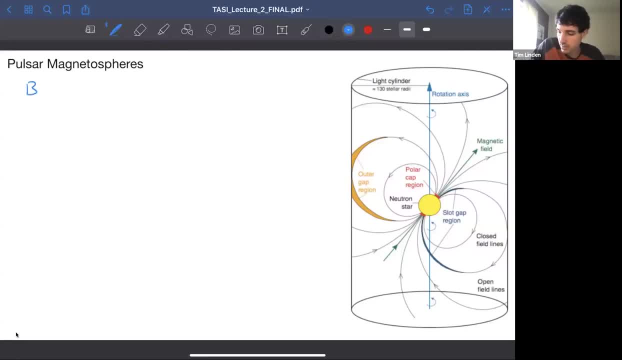 coolest thing I think in physics to just throw numbers into The second thing sometimes. stop and think about this again. So the magnetic field of a pulsar is around 10 to the 10 Tesla. So that means the energy density right. 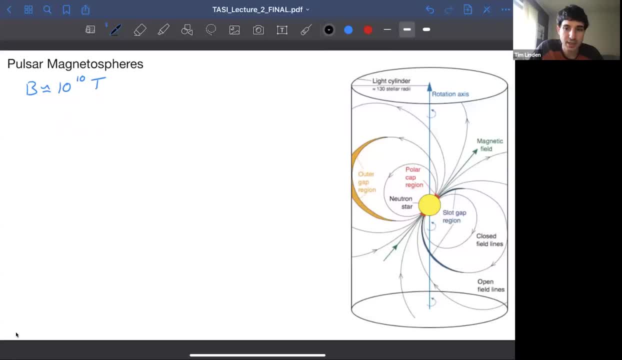 in the pulsar is 20 orders of magnitude higher than, say, an MRI or something like that. The radius of a pulsar is around 10 kilometers And inside that 10 kilometers we have a mass that is about 1.4 times the mass of the sun. 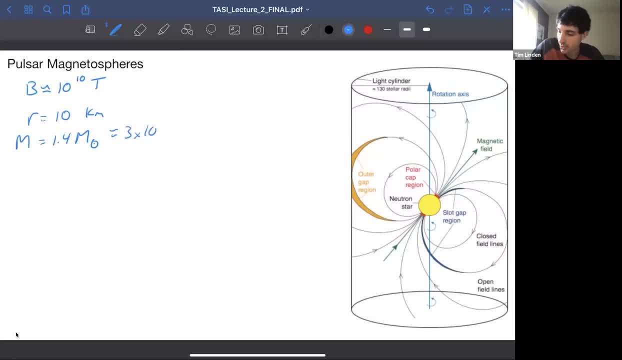 And so that is around 3 times 10 to the 30 kilograms. The fastest pulsars can spin with a period of about 1 millisecond, about 1.5 milliseconds actually, which means that I'm moving 10 to the 30 kilograms on the surface. 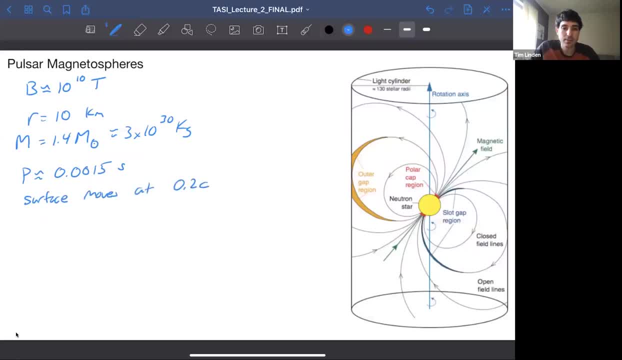 It moves at 0.2 C right. So this is taking like huge objects and moving them fast, which is cool. And so what does this do? How does this accelerate particles? Well, magnetic fields can't accelerate particles. 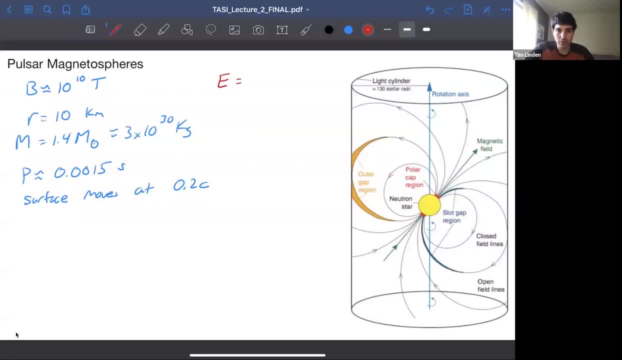 but they're spinning rapidly. So this induces an electric field, which is omega or spin. Is a magnetic black hole, some sort of Fermi accelerator? Potentially, if you had a massive and spinning black hole, you could accelerate particles outside of the event horizon. 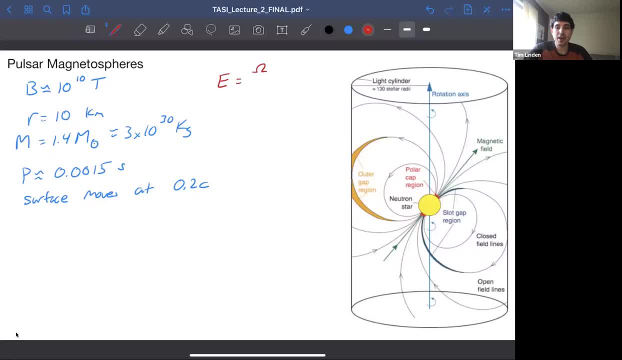 But most black holes are thought to not be heavily charged Like you can have charge on a black hole that's, you know, often thought of for in kind of conceptual studies, but they're not expected to have magnetic fields on this scale. 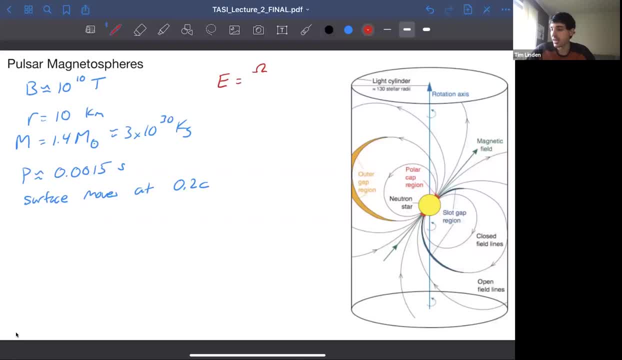 This is because everything in here is a neutron and you know, electrons and protons collapse when it was spinning rapidly. then you get really strong electromagnetic fields at the surface. So the electrical field is omega times r, So you get a really strong electric field. 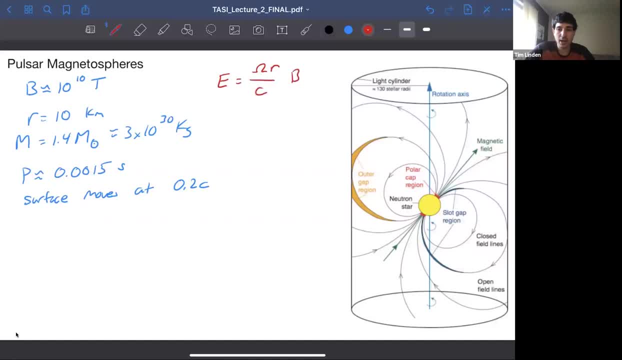 divided by C times the magnetic field strength, And so this gives you an electric field which has a strength of 3 times 10 to the 5 volts per meter, And that's again a huge number. Think about that again at some point, because it's. 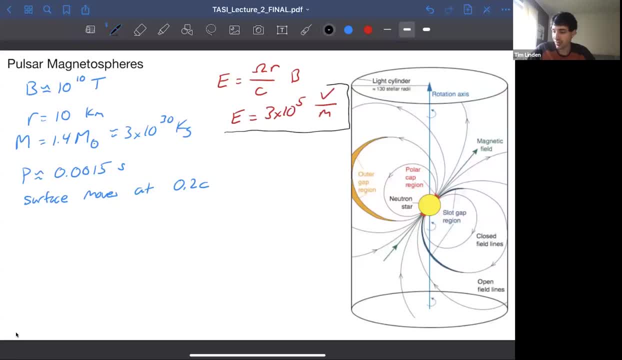 cool. So what does that do if I produce that sort of electric potential on the surface of this object? It just takes. I have neutrons, that are electrons and protons stacked and it just takes the electrons and pushes them off the surface. We call this like boiling electrons: Boils electrons off surface. 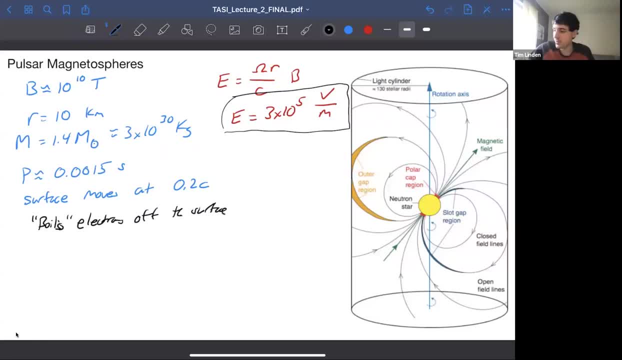 And those electrons get accelerated along these field lines as the pulsar is spinning. If it's a closed field line, it comes back and nothing happens. But if it's open field, but you can also get open field lines And the reason you get 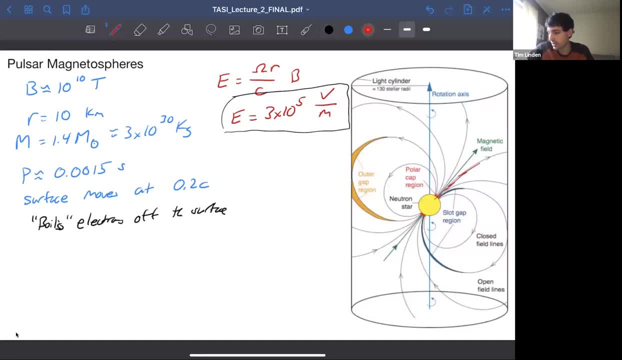 open field lines with a rapidly spinning pulsar is because they're not going to be able to get back to where they were supposed to be in time. So what you can do with a rapidly spinning pulsar is: you know, this field line here would want to. 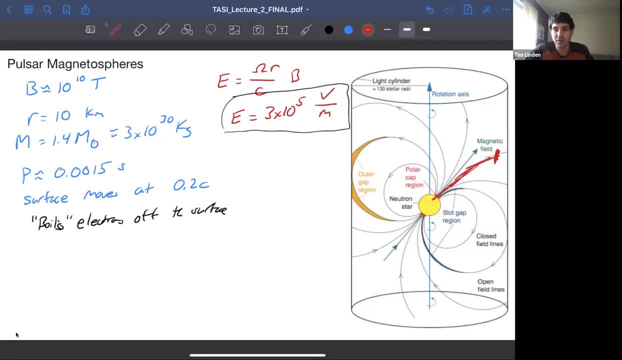 close. but eventually, here this thing is spinning so fast. right, it's spinning 0.2 C at the surface, Here it's spinning faster than the speed of light, and so you can't close that field line anymore. Like the, you know the particles in the 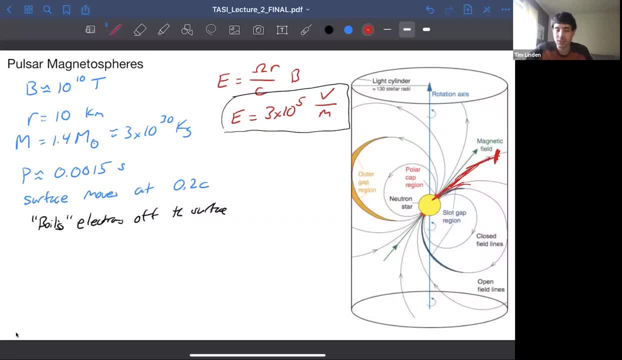 magnetic field structure can't get back to where it's supposed to be in time, So they accelerate. There's a gap here where the closed field lines go to open field lines And then, vaguely, what happens? So you have an electric, an electron, and that. 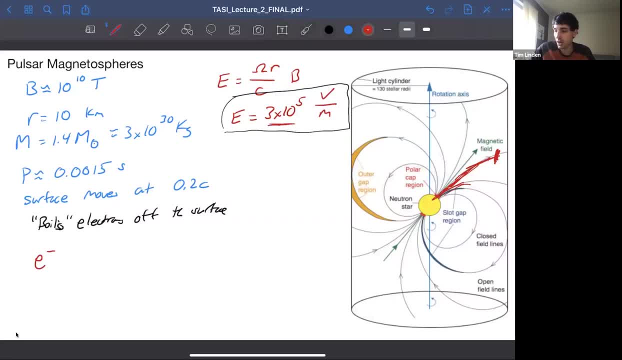 electron is being accelerated by this 3 times 10 to the 5 volt per meter electric field And it hits, it has a, it interacts and produces synchrotron radiation. Why does it produce synchrotron radiation? Because it's in a 10 to the 10 Tesla. 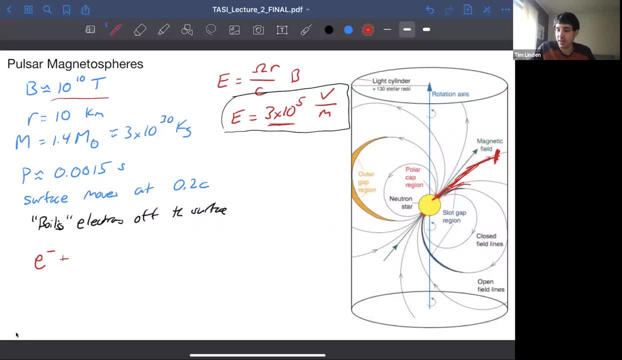 magnetic field. So I have this high-energy electron that's been accelerated and then produced synchrotron emission, And so that's you know, electron plus some photon, which virtual, virtual, virtual, virtual, virtual photon for the magnetic field leads to a really high-energy photon plus an. 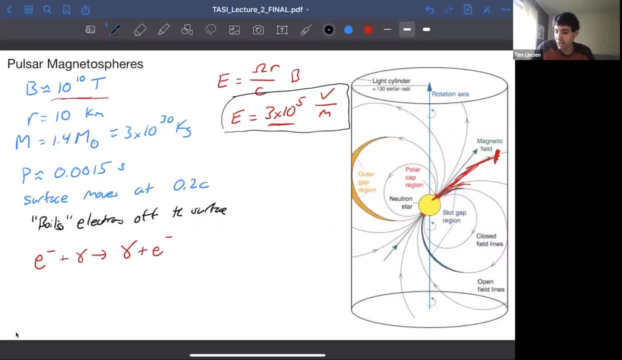 electron, And so this, you know, we're used to thinking about synchrotron emission inside of, say, a particle accelerator that is relatively low energy, This is very, very high-energy synchrotron emission, usually much more than a TeV. And so now I have this gamma ray, synchrotron gamma ray, and it is you. 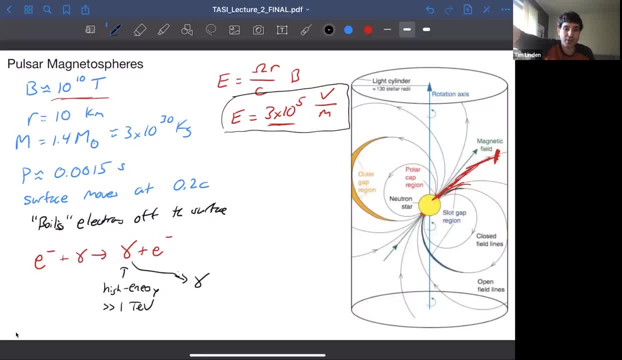 know a TeV and it is now moving through this electromagnetic field. And if you go back and review Jackson, inside strong magnetic fields your gamma ray photon can go to E plus E minus. Normally you can't just have gamma go to E plus E. 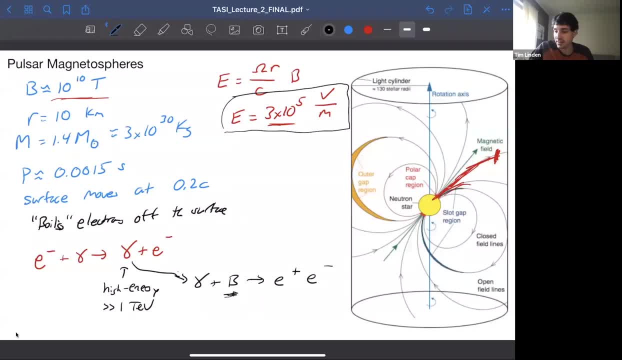 minus. you can't conserve quantities. but this magnetic field strength, again 10 to the 10. Tesla kicks in here and produces more E plus E minus. What do those E plus E minus do? They are in a huge electromagnetic field, so they get. 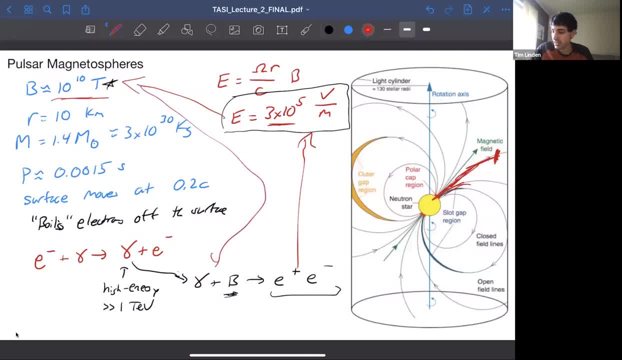 accelerated. they synchrotron radiate, they produce these. these go back to these. you can see the loop that is being produced. Eventually, boiling one E minus off the surface leads to 10, to the 5 E plus E minus. 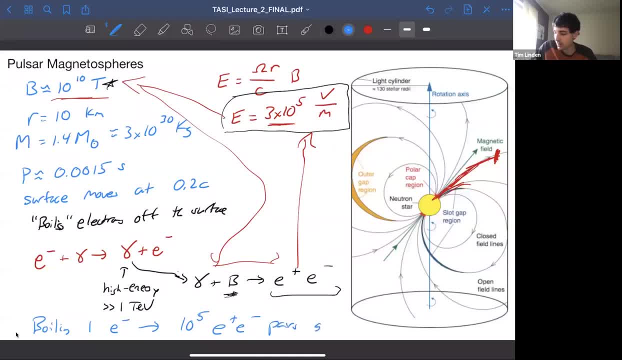 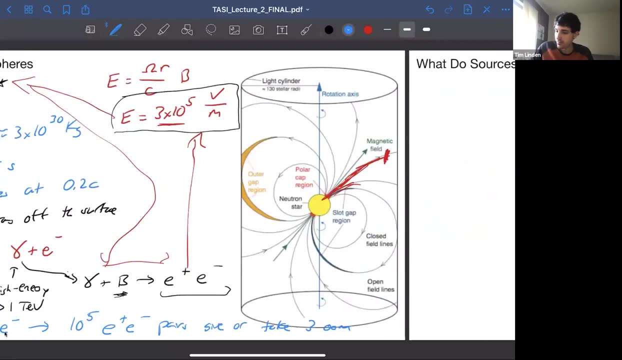 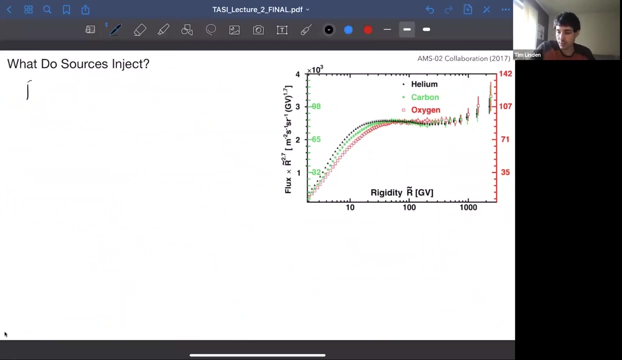 pairs give or take three orders of magnitude depending on who you ask, But a lot of E plus, E minus pairs come out of the single initial electron. Okay, So what do these sources inject? So we just talked about pulsars. Pulsars inject. 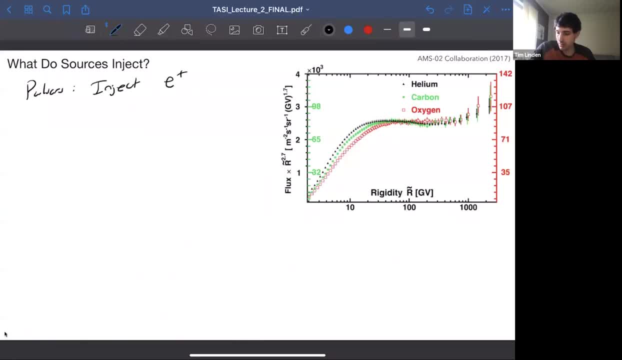 E plus, E minus, And that's just because the electrons are easier to boil off the surface than, say, protons or something like that. The second thing is supernovae, which are also cool. Supernovae produce a key number. 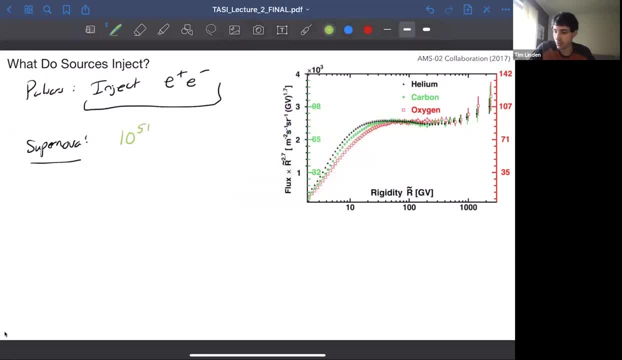 to know in astrophysics is 10 to the 51 ergs. is the total energy of a supernova. in kinetic energy, The actual total energy of a supernova explosion is 10 to the 53 ergs, 99% directly to neutrinos which then don't do anything. 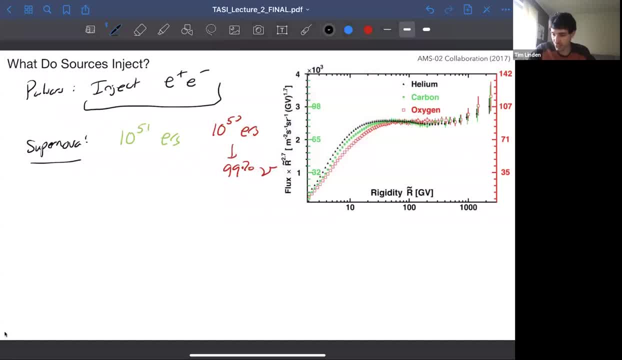 So 10 to the 51 ergs is what's available for a high-energy astrophysics. Again, tremendous amount of energy. And what do those inject? It ejects and accelerates everything that is around a large star when a large star explodes. So that is protons. 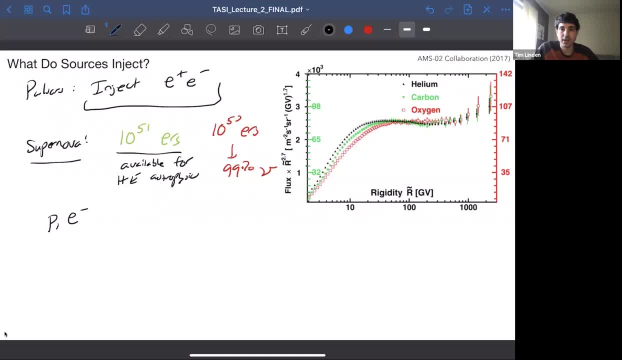 some electrons- not positrons, because there is not much antimatter around stars, but you know protons, electrons, but also helium. There's. a lot of hydrogen is fused already into helium and then it's fused more into things like carbon or carbon dioxide and then it's fused into helium And then it's fused more into things like carbon or hydrogen. but again, we're talking about a lot of hydrogen that's fused already into helium And then it's fused more into things like carbon or hydrogen, And then it's fused more into things. 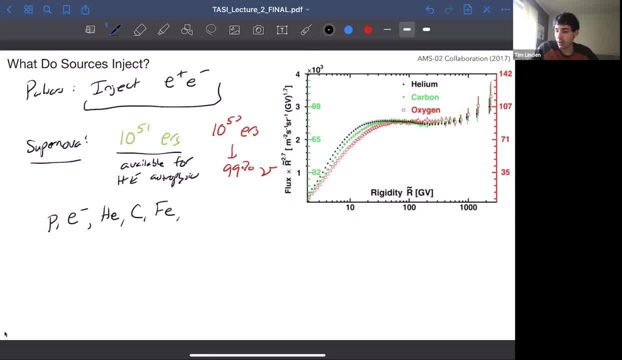 or iron or you know whatever, every other thing that you might care about. So that's what these look like here and these are the spectrum. So here flux. now they've multiplied by r to the 2.7, which is committing an observer's sin. 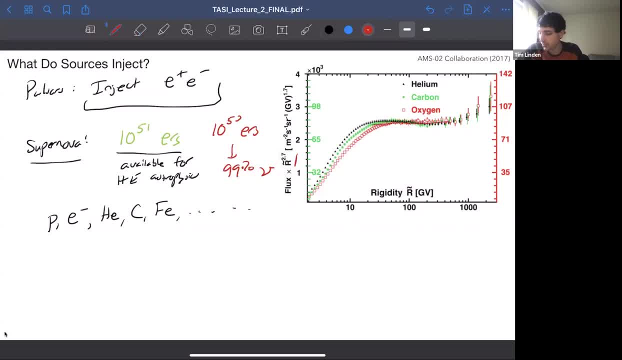 but I'm okay with it here. So they multiplied by r to the minus 2.7, which means this is going to look really flat, which it does. and then this is a function of rigidity, which, you know, at very high rigidity is similar to total energy. So here's what helium looks like. 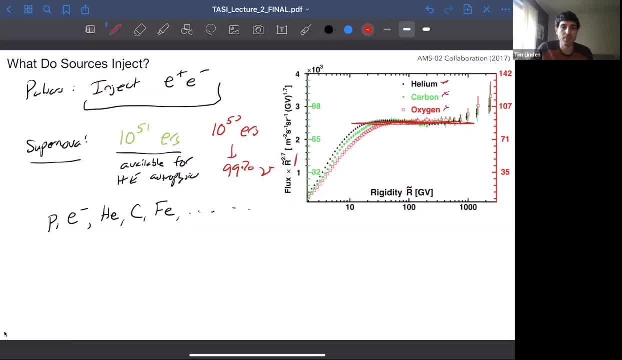 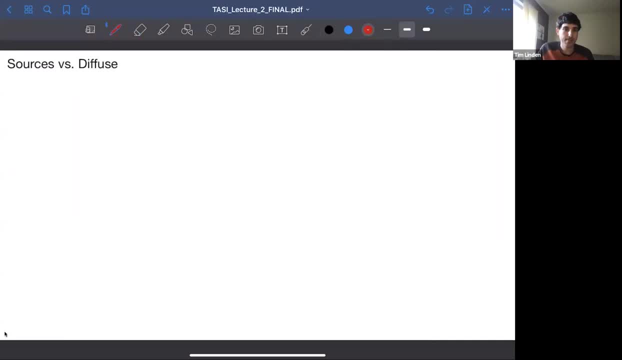 here's what carbon looks like. here's what oxygen looks like. They all look the same because they're all being accelerated by the same sort of object. Okay, So what happens then? So a supernova goes off and what we said? the number we should know. 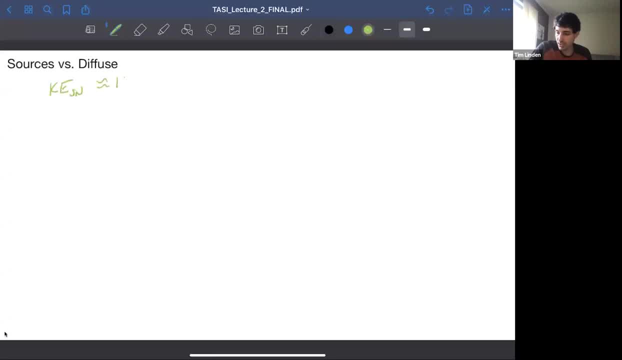 is that the kinetic energy of a supernova is around 10 to the 51 ergs. So maybe that just you know, all the particles deal with the supernova energy, which is very high, and things happen, et cetera, et cetera. Another random number to know and then we'll compare them. 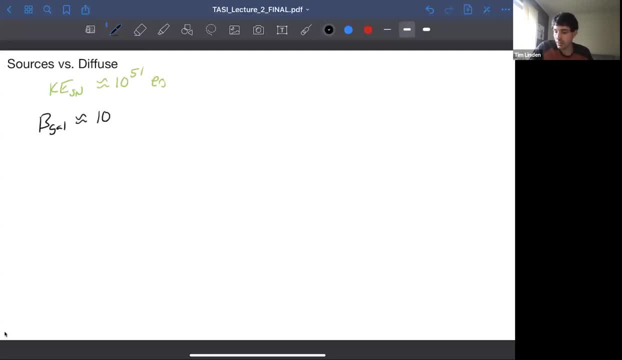 is that the average magnetic field strength in the galaxy that we can measure is 10 to the minus 5 gauss. Gauss is CGS units, but it's just 10 to the minus 4 tesla. So this is 10 to the minus 9 tesla. It's a small number where the neutron star was a big number. 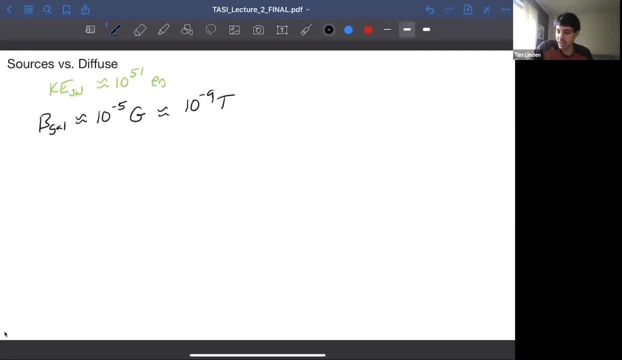 Now the reason CGS units are nice for these sort of calculations is that the magnetic field energy density- I don't have to worry about the permeability of free space anymore- just 1 over 8 pi e squared in these units. So this is 10 to the minus 10 ergs percentile to the third over 8 pi. 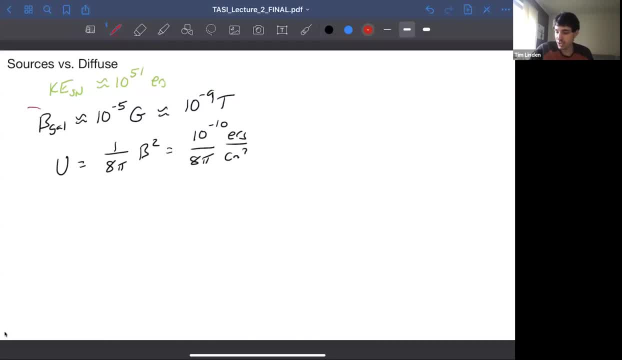 So how large of a region. so if this is, this is the whole Milky Way, has something like this over the whole Milky Way, how large of a region can this supernova influence if it has 10 to the 51 ergs to work with? So that's just some some unit multiplication here, 3 times 10 to the minus. 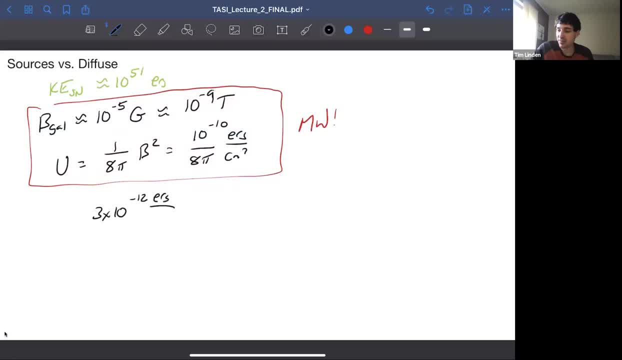 12 ergs, that's 10 to the minus 10. divided by 8 pi 3 times 10 to the minus 12 ergs. per centimeter cubed times some volume, it's equal to 10 to the 51 ergs. I'm not going to. 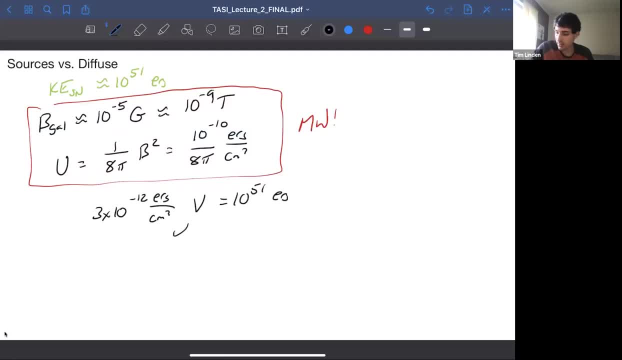 you know, take this out. The answer is that r that gives you that volume is 4 times 10 to the 20 centimeters, which is around 100 parsecs. So in a region you know near, it's actually going to. 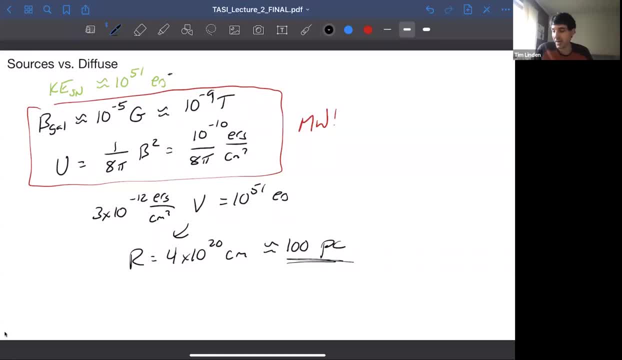 be smaller than 100 parsecs, because the supernova does other things besides: produce magnetic fields. but in some region that's around 100 parsecs or so, the supernova can be dominant And then outside that region background are dominated and we call it diffuse region where many supernovae are contributing small. 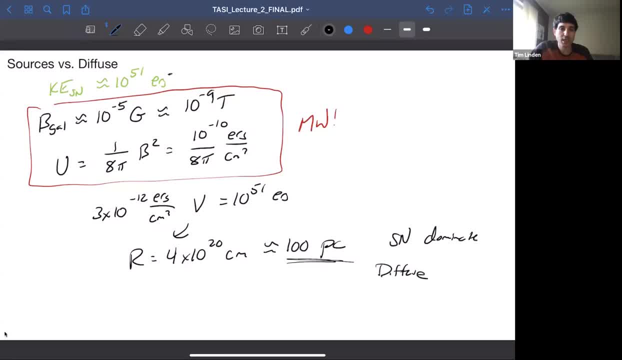 amounts. But you know, one single supernova is not producing what or influencing what the particles do outside that region. So let's think about this real quick. You know, we had our picture of the Milky Way here. We said this was 500 parsecs in height. We said this was 20,000 parsecs. 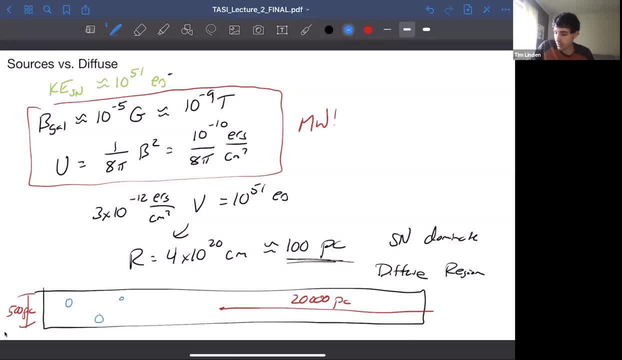 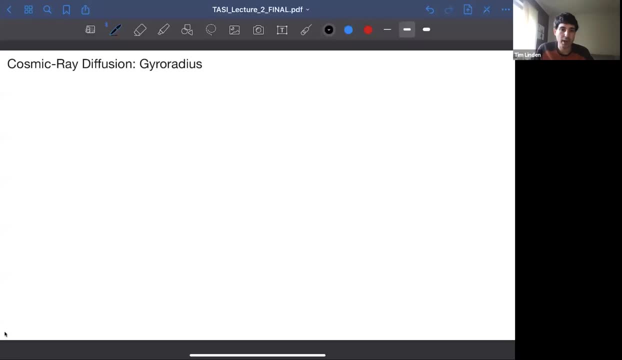 So you'll have a bunch of regions- you know this is going to look like a chocolate chip cookie or something- a bunch of regions here where different supernovae dominate in our galaxy, and then a bunch of diffuse regions outside. So what does a particle do in one of these diffuse regions with a microgas? 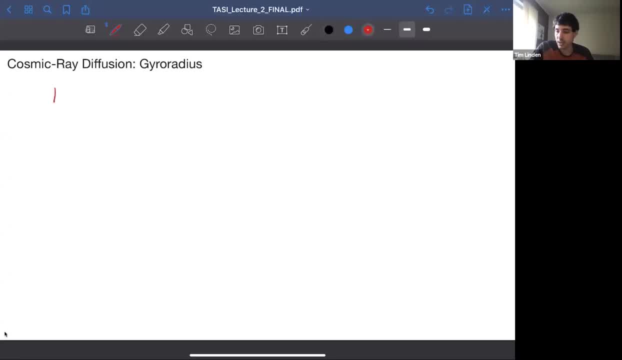 magnetic field. How do particles move through the ISM? And the ISM is called the interstellar medium. It's just that diffuse region outside of different supernovae. ISM, random interstellar medium. Okay, so what's the gyroradius of these particles? 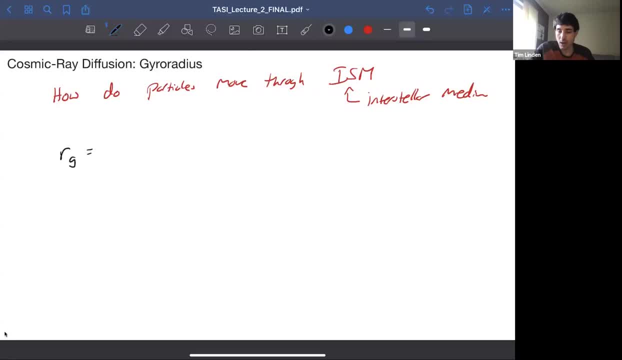 So you might know the gyroradius of particles from colliders or something like that. You know I might have a number in mind for the LHC. It is m v over the charge of the particle magnetic field strength. This is 3.3 meters. 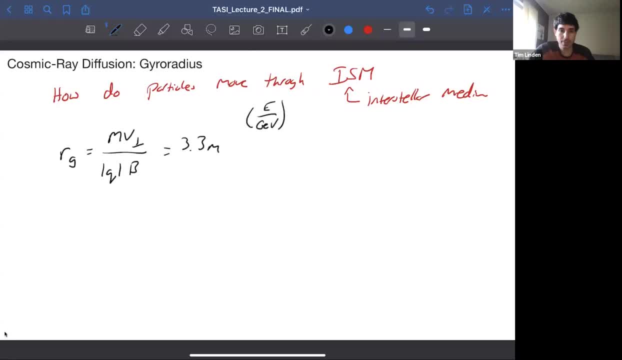 for an energy that is 1 GeV. Beta is velocity of the particle, Q is the charge of the particle and the magnetic field strength is 1 Tesla. So, okay, so 3.3 meters at these values. So what? at about 10 microgauss or so? 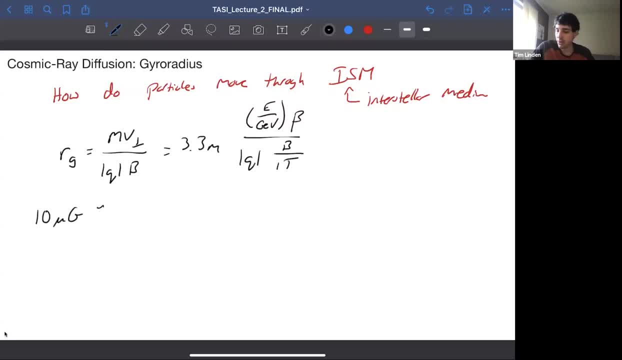 which is the average for the galaxy, which is, you know, around 10 to the minus 9 Tesla. Then Rg is around 3 times 10 to the 11 centimeters times e over 1 GeV. So for a 1 GeV particle, 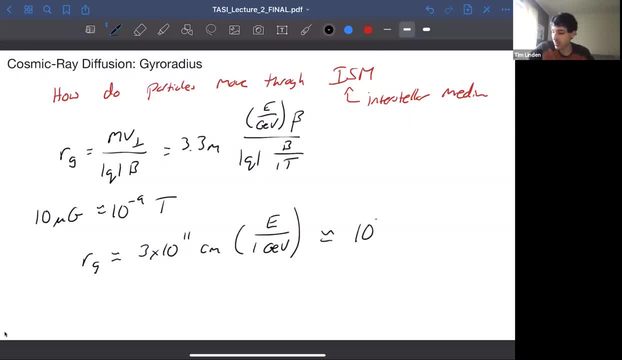 it's around 10 to the 11 centimeters. That sounds big, but that is 10 to the minus 7 parsecs, which is very small compared to the 20,000 parsecs of the galaxy, And the- you know, moral of that story is that particles do not cross through. 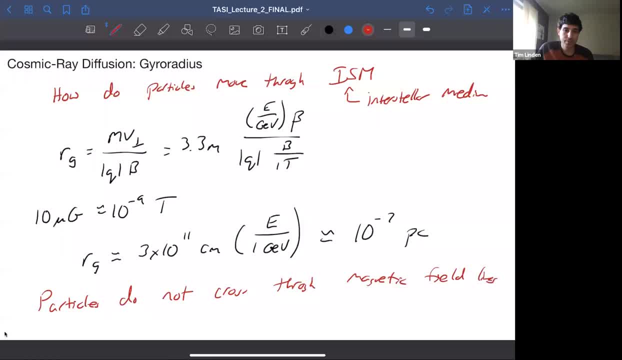 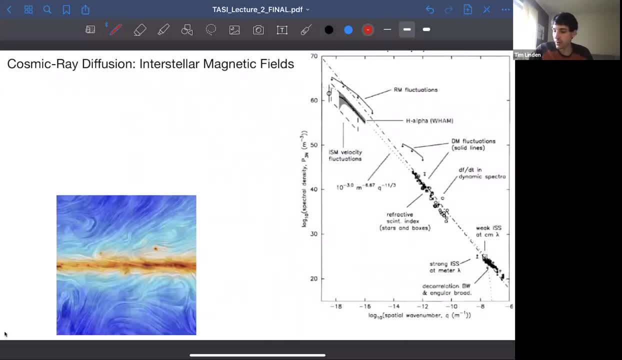 magnetic field lines right, So you might have some story or some picture in your head of what these particles are doing where you know. our galaxy maybe just looks like this now, and there are some magnetic field lines coming out of our galaxy. 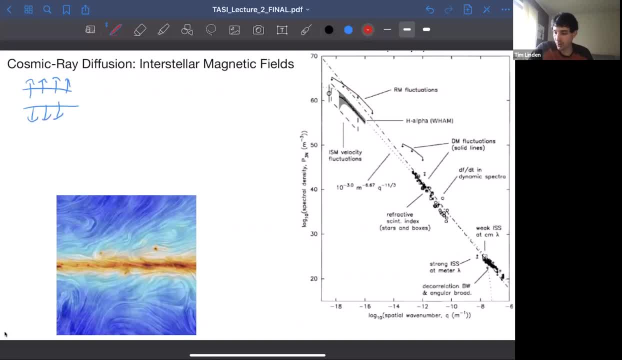 or something like this. And then the particles are, you know, just rotating here, and the velocity of the particles is maybe now C over 3, because they're relativistic and everything just kind of, you know, gets pushed out of the plane of. 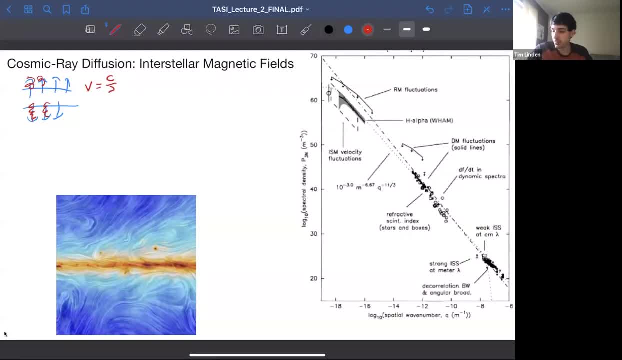 the galaxy very quickly, But that's not the right picture. No, The reason that's not the right picture is because these magnetic fields are extremely turbulent on every scale, And I'm not going to go into the weeds of this scenario. This was. 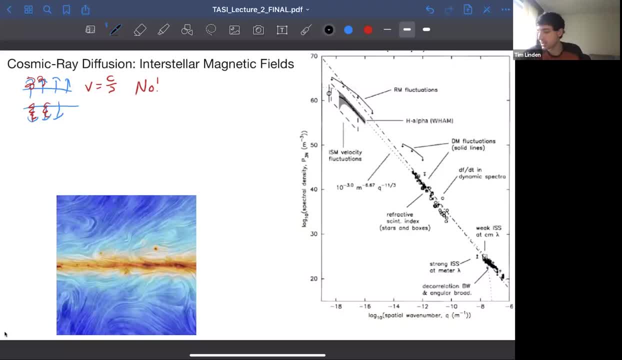 actually so. here is on the right of this is the turbulence scale is the spatial wave number in inverse meters of the electron density distributions. So where electrons overdense and hot underdense in our galaxy, You can change that into the scales of which the magnetic field is turbulent and moving. 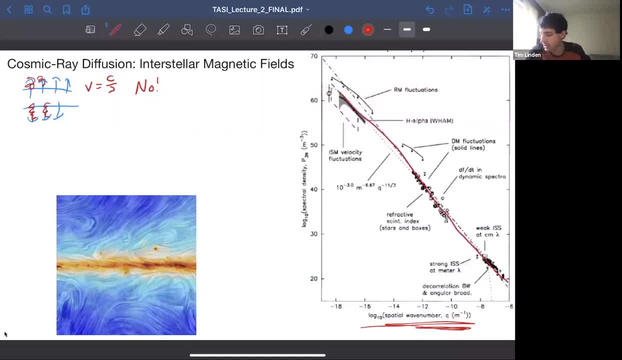 in different directions And there's this really nice power law that continues over 12 orders of magnitude and wave number, which is 12 orders of magnitude in inverse distance or 12 orders of magnitude in distance, And over all of these scales you get different energy And this has a power spectrum where the 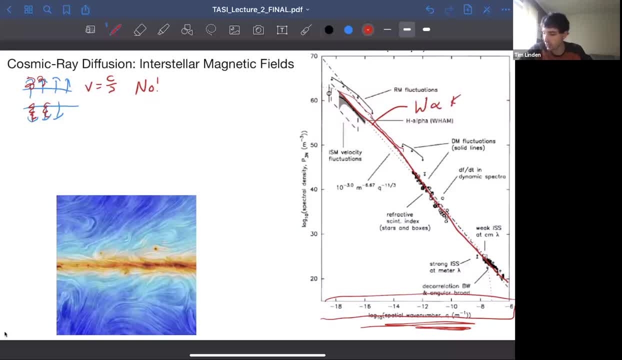 way, the amount of power on different scales is proportional to the wave number of the minus five-third power, And that's been measured now over over 12 orders of magnitude. It was also predicted analytically by Kolmogorov In the 19th century. 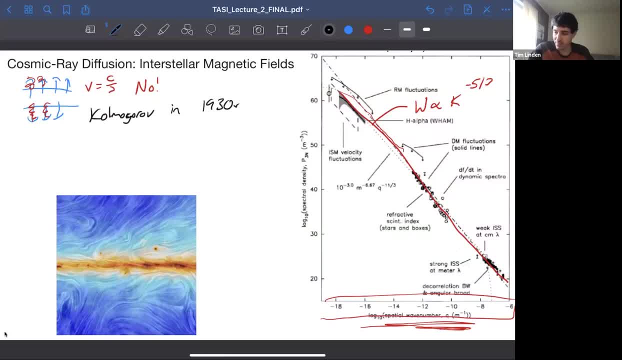 1930s, I believe, predicted this turbulence scale And basically what you do is: here's your different K wave numbers for the inverse distance scales of turbulence. Here's the amount of power in those scales And you inject the power at about 100 parsecs or something. That's the size 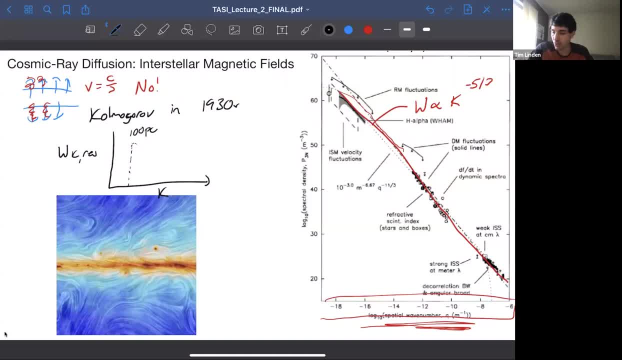 of the supernovae, So it injects a bunch of turbulence at that scale And then basically the turbulence cascades down until there are frictional terms down here between electrons that have very different densities on small scales that can now frictionally interact with each. 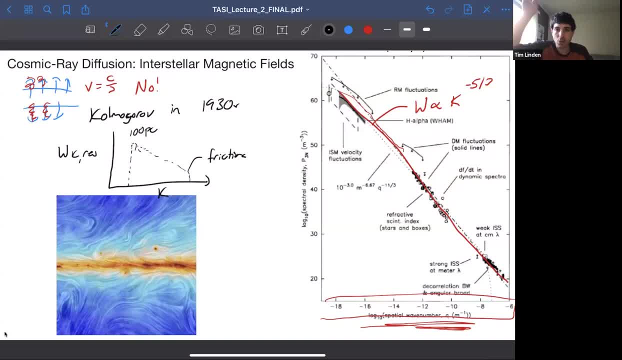 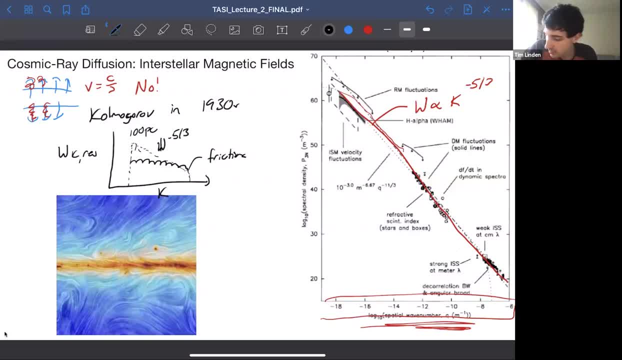 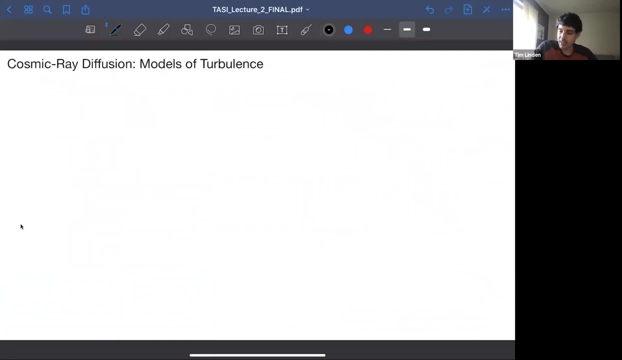 and you get K to the minus 5 thirds. Details of that aren't important. What are is important for our indirect detection studies? Did I skip a slide? I did not, Okay. so what's important for our indirect detection studies is that the scales influence. 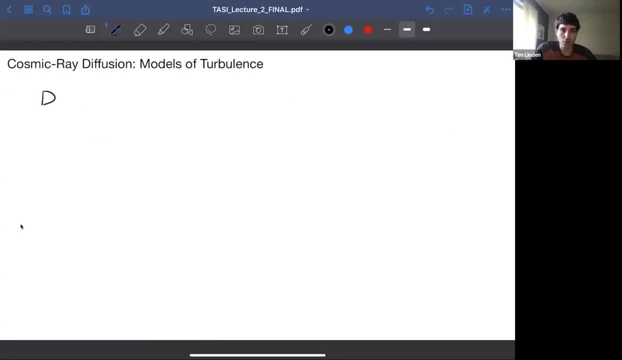 the diffusion of particles. So we're going to have some diffusion of particles. They're going to move from magnetic fields moving in one direction to a different direction. They're going to move from other direction the other direction and you'll find that there's a resonance. 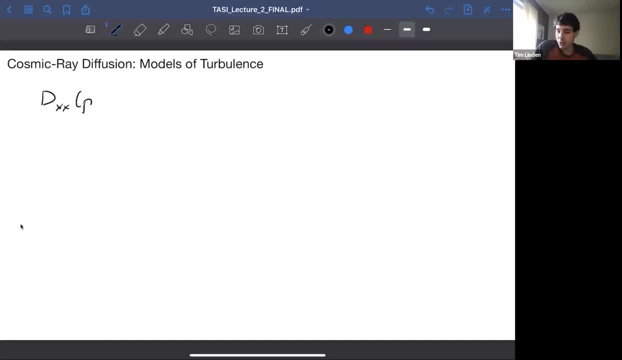 condition- again not going into details- between the gyro radius of the particle and the amount of power that's on that scale. Particles are most affected by wave numbers that have the same scale length as their gyro radius, So the diffusion constants tend to have some, some value where they go with the 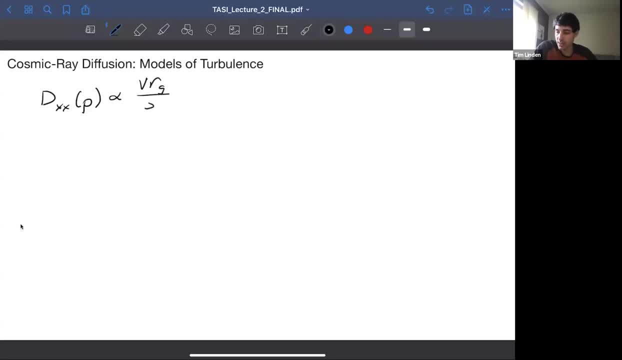 velocity of the particle C, the gyro radius of the particle over 3, because a third of its velocity on average is in one direction. and then this is 1 over the scale of the turbulence and the power that's on that turbulence scale. 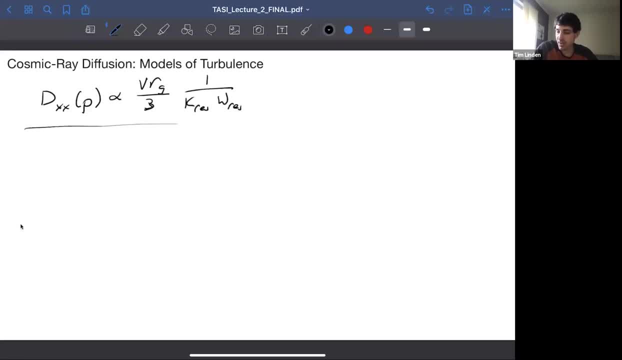 Not important, but you know this is. this is basically the background calculation you can analytically do, And that means that this is proportional to the gyro radius and we already said Rg is proportional to energy of particles. so that's the important part that's coming out of this calculation for our 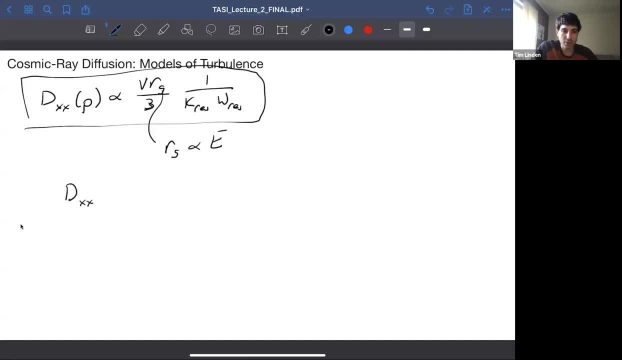 measurement. The diffusion constant in some direction is proportional to e, to the delta, and Kolmogorov again analytically calculated everything right in the 30s because he was impressive, and that means that delta is 1 third in the case. 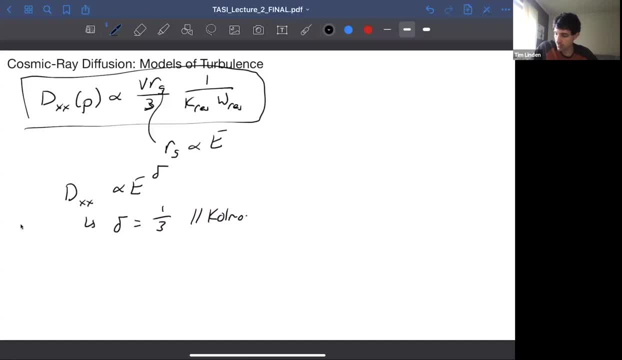 of what we call Kolmogorov turbulence and delta is 1 half for another model by Kritsch and turbulence And Kolmogorov actually fits this model here much better. but there are some reasons that in specific environments you might want this other turbulence models. Okay, so now let's get 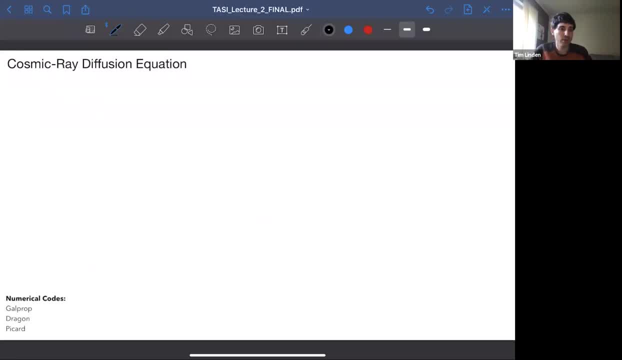 to what we actually want to do. for the rest of this, We have some diffusion equation: Cosmic rays are injected by supernova and or pulsars. They're accelerated to very high energy. then they get out of those regions And they start moving through their interstellar medium, where the 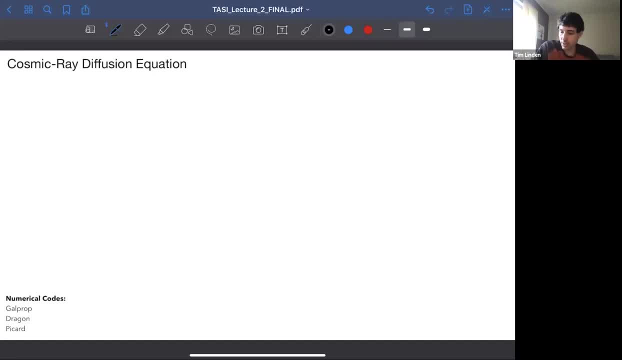 magnetic fields are weak and highly turbulent. So what do they do then? We want to solve for psi, and psi is the cosmic ray density. We want to solve for, maybe, the cosmic ray flux hitting us as a function of time. Cosmic ray flux is a 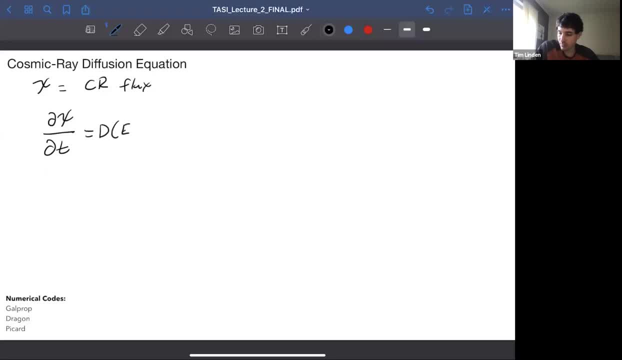 function of time and this is equal to some diffusion Of these cosmic rays and the Laplacian here. this is a diffusion equation plus this second term here. I should just put this in the notes automatically because it's long. I'm gonna explain all these terms in just a second. This is an energy. 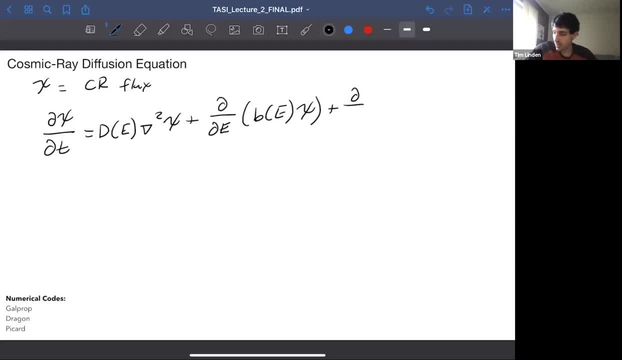 loss term, then a possible convection term. if there's some sort of like wind or other- pressure from charged particles moving the cosmic rays, This is a decay term. If the particles are, say, radioactive nuclei or something they might decay. And then some source term, which is that you know, energies, some. 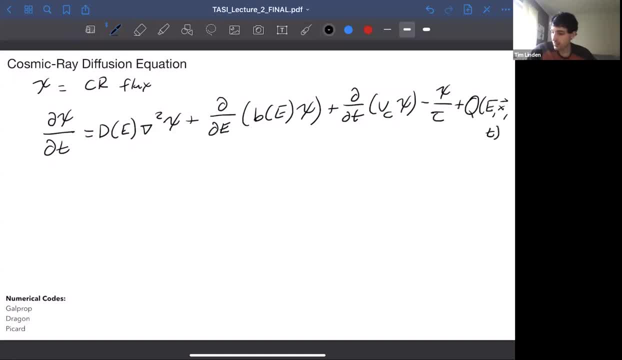 values of X and then time. So let's go over that again. Flux, and maybe this is equal to zero in a galaxy. That's often an assumption that is made, which is that the flux is not changing. everything is in steady state. 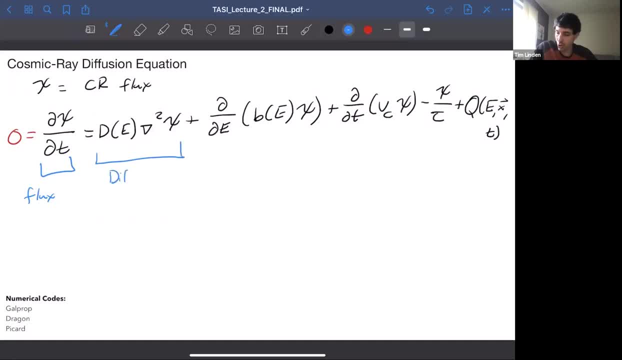 This is diffusion along magnetic field lines or, you know, in magnetic turbulence. This is energy losses. Energy losses might be because our protons are hitting gas and they're having pi zero decays and then the proton is gone, it's lost its energy. Or it could be something like inverse Compton. 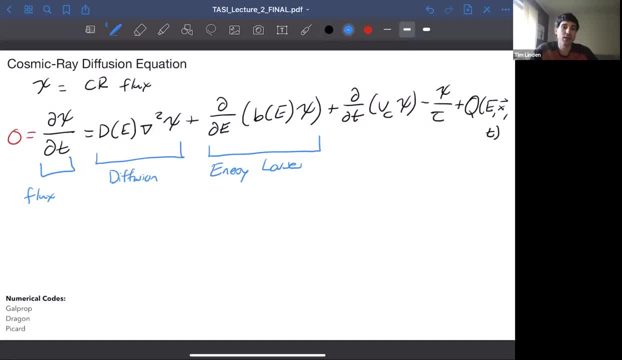 scattering The electrons hit some starlight, or maybe the electrons synchrotron radiating inside the galactic magnetic field, whatever it's losing energy. This is some possible convection term. This is, for instance, if there's some wind pushing gas and things out of. 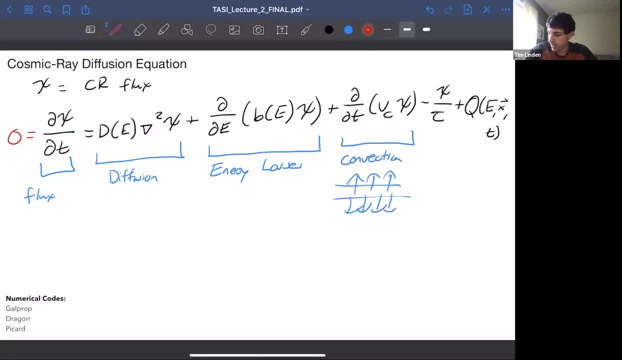 galaxies like that. This is radioactive decay And this is our source And source. you said supernova could be pulsars, could be massive black holes, could be dark matter. maybe Let's be optimistic, Okay, And then, in real life, these things. 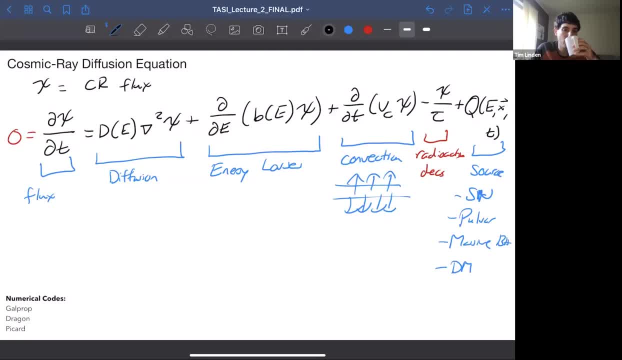 you know, this is some long partial differential equation you have to solve, And so these are done numerically on a grid, And so you know, you have some galaxy here Now. we talked about some some disk here that was maybe 0.5 kiloparsecs, It turns out the diffusion is: 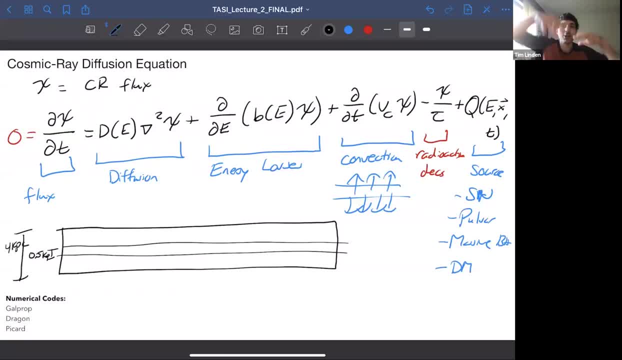 important over a hundred, a larger height of like four kiloparsecs or something like that. So you know, if something goes above the plane of where the stars are, it can sometimes get knocked back down by magnetic field. So you have to set your boundary condition to be a little bit higher. This is the center of 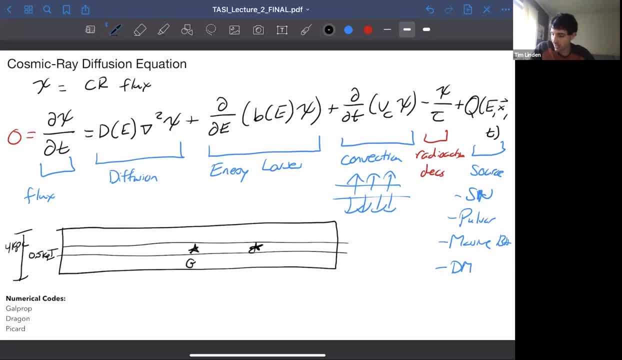 the galaxy. This is the position of the sun, galactic, center, sun. And then this we usually simulate, you know, 20 kiloparsecs or something out here, And these are done by different numerical codes which you can find on the web here and solve and, you know, put them in, install them. 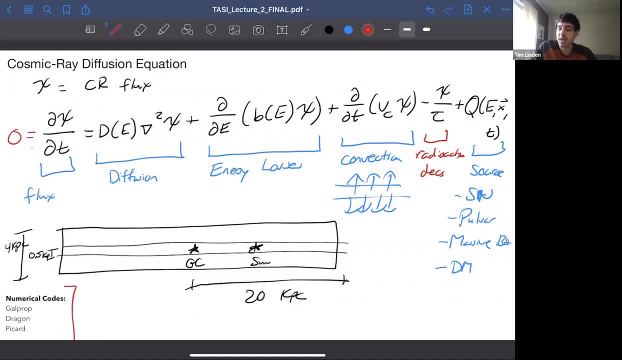 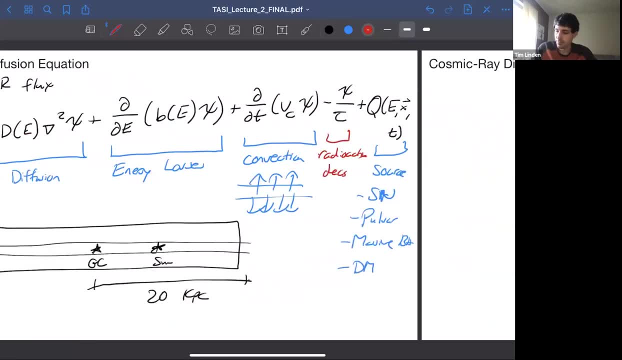 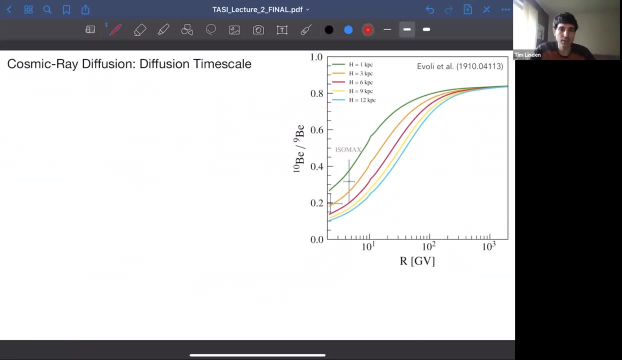 on a computer, run them for a while, And then you solve out this steady state- usually assumption- of what the cosmic ray density looks like at Earth. So how long do cosmic rays diffuse in our galaxy? We can study that and we can model it with observations. It's not just some like. 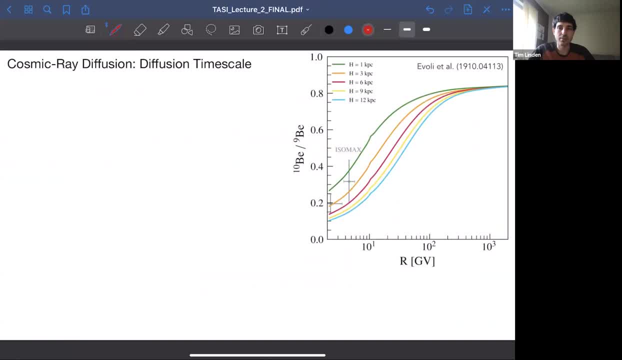 you know, fact we have to pull out of a hat Based on some starting model of what cosmic ray diffusion looks like. So this is done in kind of a cool way. So you look at the ratios of different particles that might decay or something. 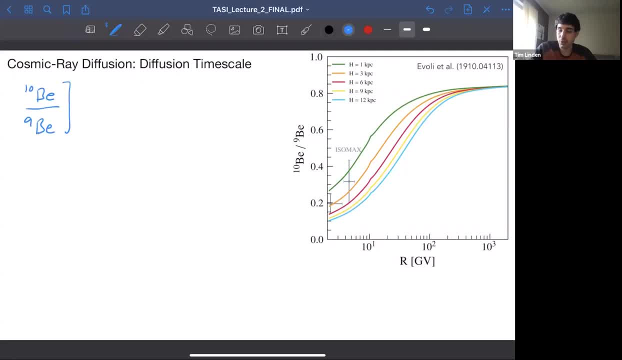 like that. So beryllium is not produced in supernova, because it's on the fusion chain. it goes really quickly to carbon, which is more stable. So you can look at beryllium-10 and beryllium-9.. 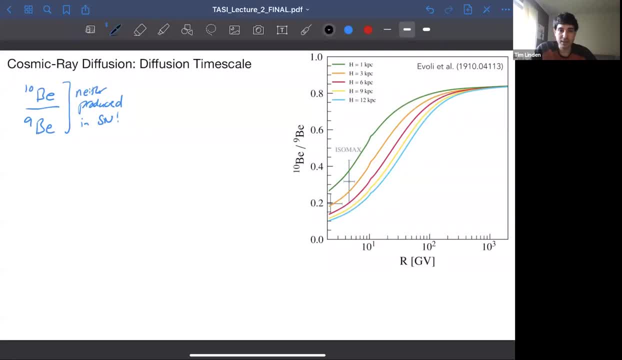 And the way that you produce it. then if it's not produced in supernova, is it's the spallation of carbon, Carbon cosmic rays hit gas and gas is just a proton And it goes and, you know, spallates off some nucleons and produces beryllium plus some other junk. 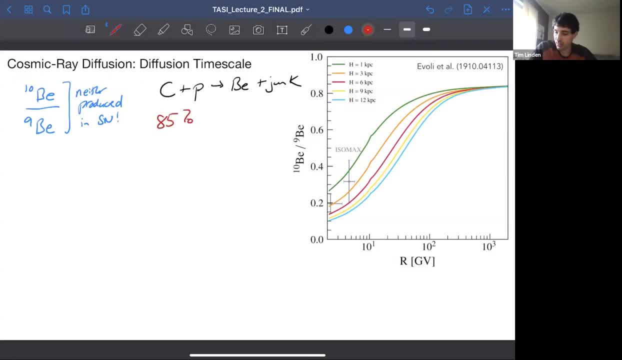 And when you do this, which you can do in a lab, you get 85% beryllium-10 and 15% beryllium-9.. But beryllium-9 is stable, Beryllium-10 is not. And tau is around 1.6 times 10 to the sixth years. That's nice If tau was one. 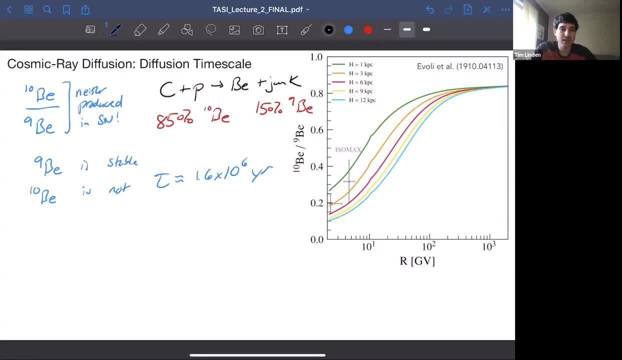 second, you'd never see it in astrophysical context, But a million years you might see the effect of it decaying. So we want to see the ratio. you know somewhere these beryllium atoms are made, somewhere on an. 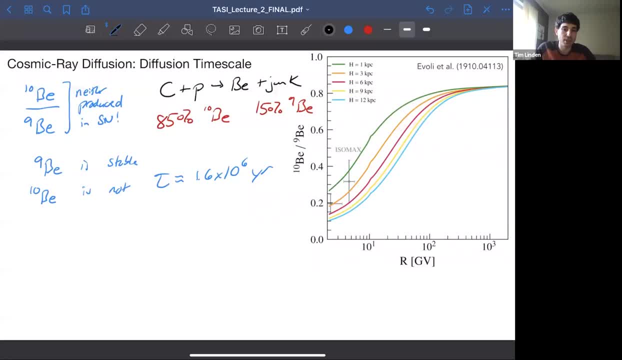 average position in our galaxy and then they diffuse through the magnetic fields to us And so we want to calculate the ratio. See up here, at really high energies where things diffuse very quickly, the ratio is still like 80%. But down here the beryllium-10 over 9 ratio is down like 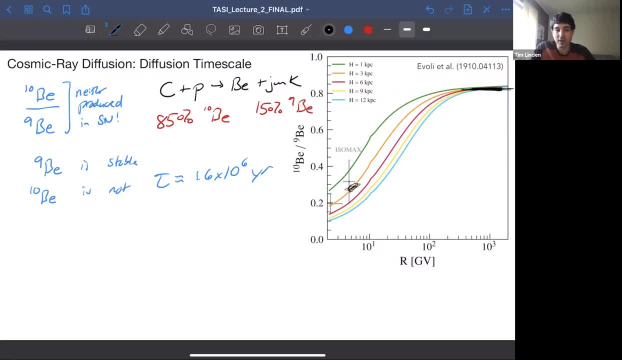 30%, And that's because these cosmic rays are moving slower. They take a longer time to get to us than a lot of the beryllium. We can measure basically how long it takes particles to diffuse different distances using this method. So how do we do that quickly? 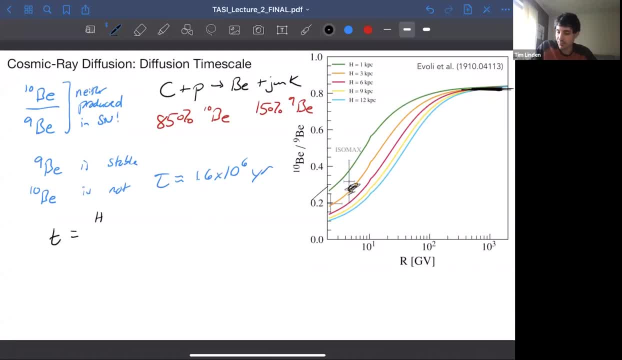 We have some timescale for these things to diffuse. Mostly they diffuse up and down because the height of the galaxy is small And that's the height of the galaxy. This is the random step size that things tend to diffuse, that the magnetic field tends to be. 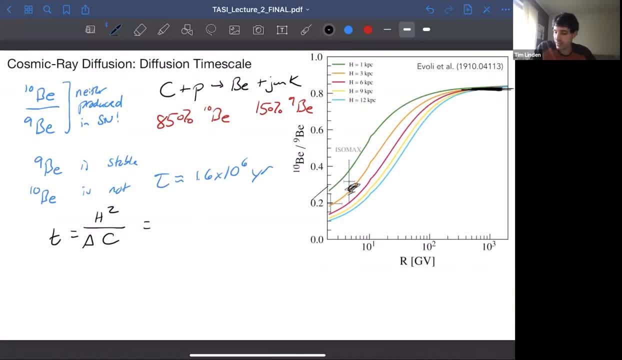 turbulent on and that's the speed of light. So I'm going to speed up this calculation and I'll do it in detail here. But this is 10 to the 22. centimeters is the height, X-axis is rigidity, which is 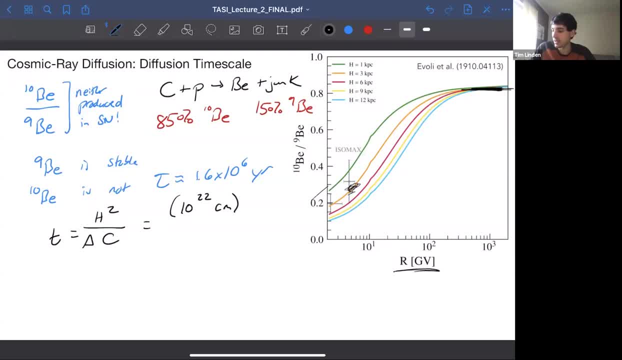 basically equivalent to. you know, it's the extra charge over mass, or, sorry, energy over charge of the particle. basically, And so at very high rigidity, it's equal to the energy of the particle. but when the particle becomes non-relativistic, there's some correction factors. 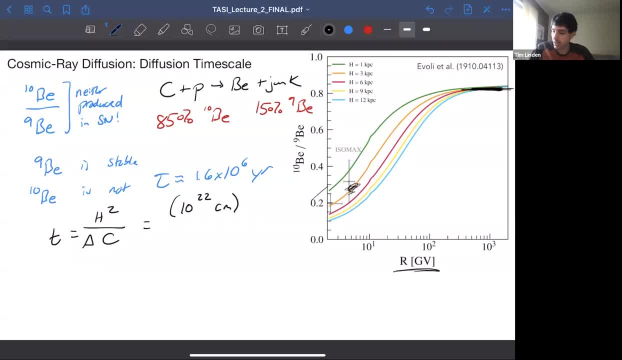 It becomes like mildly relativistic. So if the height of our diffusion is around 4 kiloparsecs or something like that, that's 10 to the 22 centimeters. This is delta. speed of light is 3 times 10 to the. 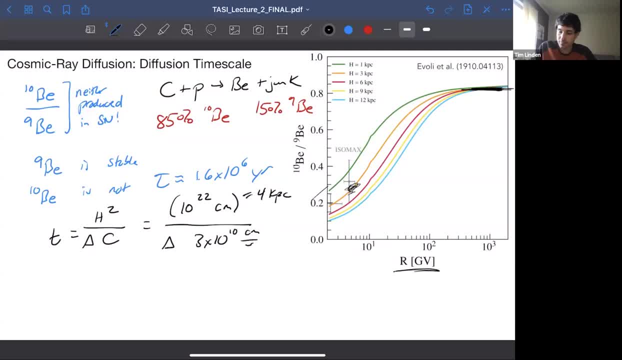 10 centimeters per second And you can calculate out from solving this that delta, the step size to get you out of here in a time frame. and the time frame right is that we need to go from 85% beryllium-10 to 30%. 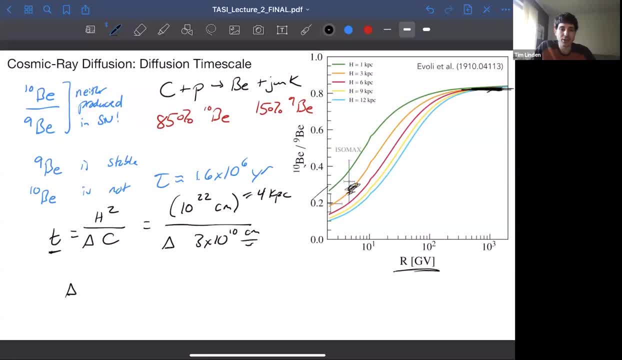 beryllium-10,, which is four decay time periods, or about three 3.6 decay time periods. So time here is 5 times 10 to the 6 years. That means that delta is around 2 times 10 to the 19 centimeters which 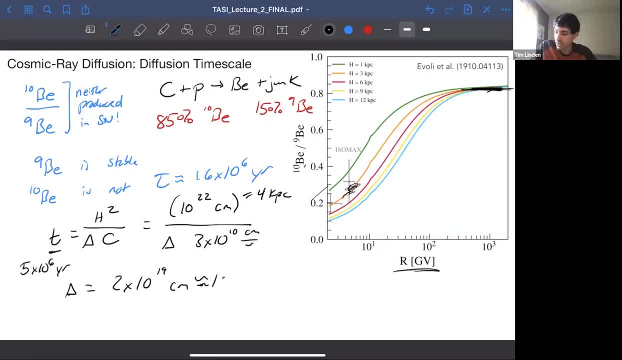 is around 10 parsecs. So the average scale at which the particles move before they bounce in another random direction and interact with the turbulence is around 10 parsecs or so. That means the diffusion constant, which is LC over 6, 6 just comes from this as being in three dimensions. 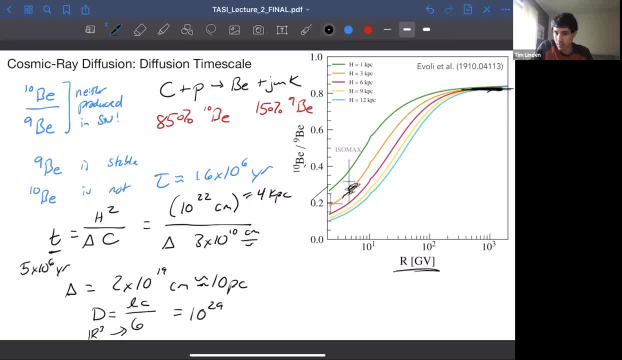 is equal to 10 to the 29 centimeters squared per second. That's another random number to know. The better number that you get if you do everything very carefully is 3 times 10 to the 28 centimeters squared per second, And this is a rigidity dependent, remember. 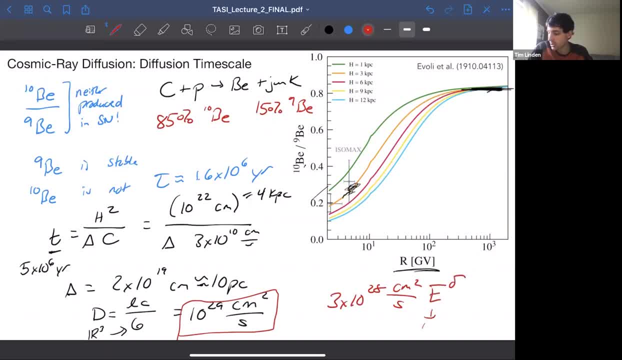 e to the delta, And this is defined at 1 GeV. How do we know that the time scale? we know that the time scale is 5 times 10 to the 6 years, because we here started at 85% beryllium-10.. 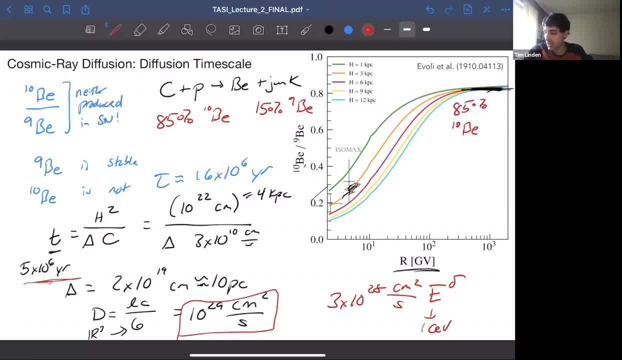 The beryllium-9 stayed constant, but the beryllium-10 started radioactive decaying, And so we went from a ratio of 6, 10 Be to 1, 9 Be to a ratio of 1, 10 Be to 2, 9 Be. 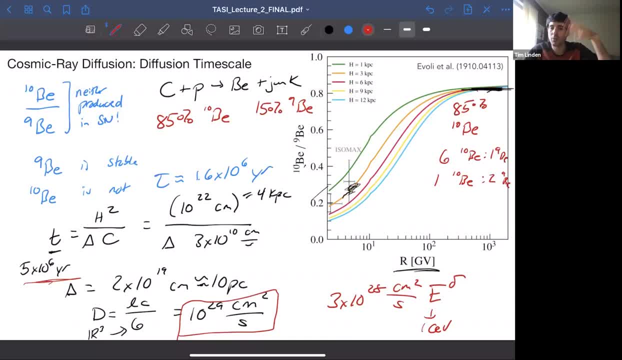 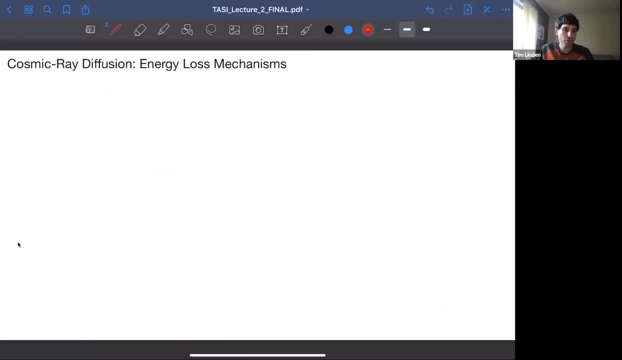 And so that is a 4, or, I think, a 3.6 exponential decays, or half-lives of this. So 3.6 half-lives times 1.6 times 10 to the 6 is that number? Okay, these things also lose energy while they propagate. 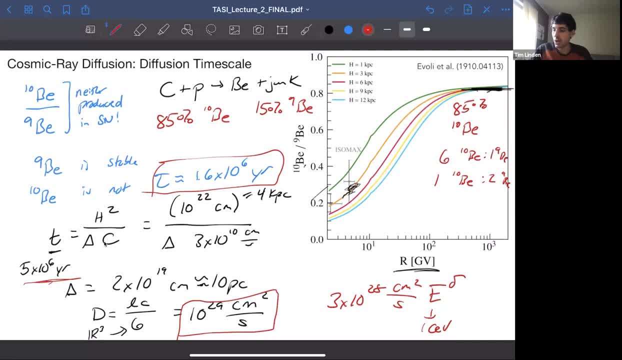 That is the observed. This is observed. Oh yeah, so I don't have the right. oh, actually, it's on this plot, right? So there are different assumptions of what the height of the halo is and they give you different predictions for the beryllium-10 to 9 ratio at the same diffusion constant. 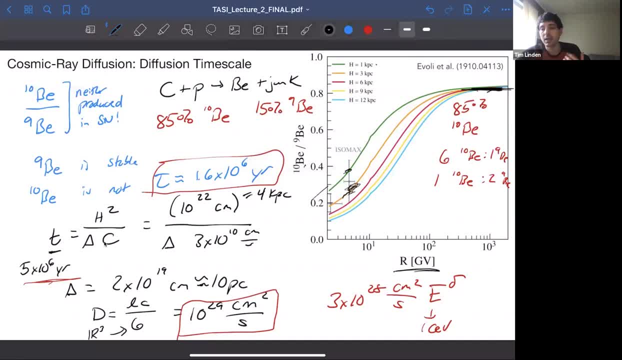 So in a real scenario, you're fitting the halo height and the diffusion constant at the same time. If you increase the halo height, you'll increase the diffusion constant that you need to get the model to work correctly. There are more observables than just this. 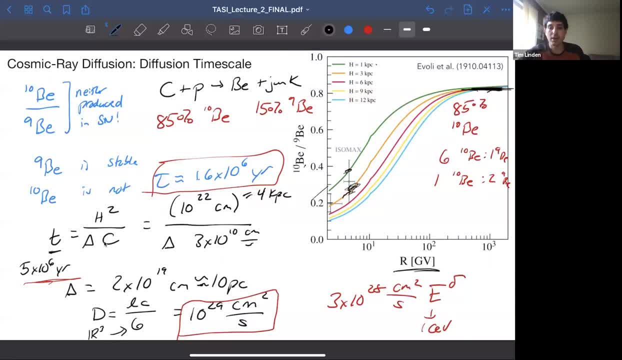 There's also a boron-to-carbon ratio that works in a slightly different way. There's antiproton production, There's helium spectra, other things that you can use. GV is gigavolts, which is, yeah, a potential. 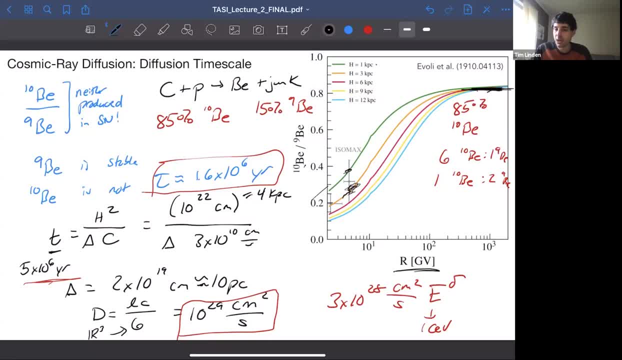 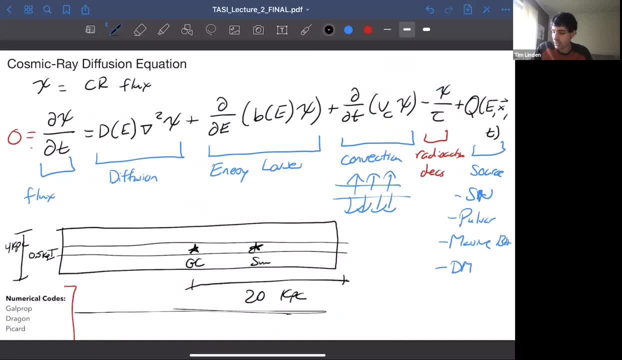 So that's the units of rigidity. Why don't we care about radial diffusion? Good question: This is 20 kilovolts. This is 20 kiloparsecs here and 4 kiloparsecs here. So if all of these things are moving in random directions, then a lot more things are going to leak out of the top of our diffusion box than they are going to leak out of the sides. 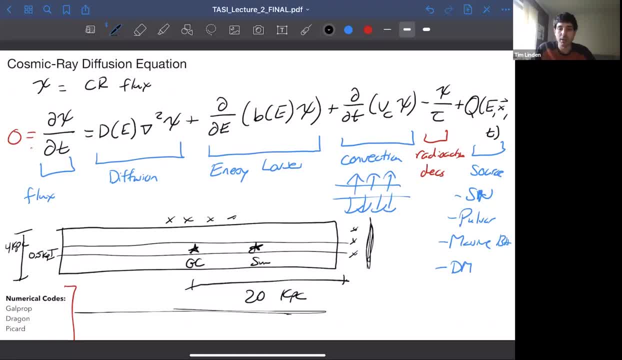 In detail. you know, if you had a numerical code you'd want to deal with both of them in detail. but you know, if you want to do the simplest thing here in one dimension, just deal with the height, because it's smaller. 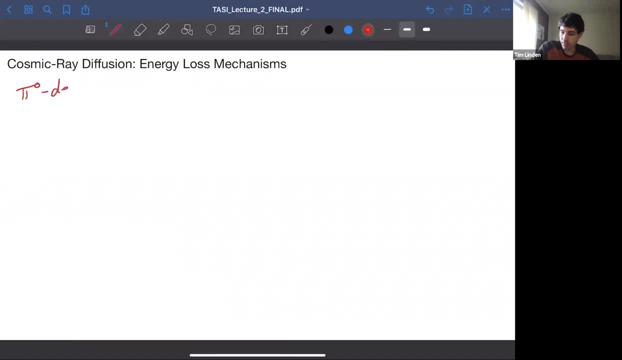 So how do these things lose energy? So for pi zero decay, we can calculate the timescales that these things happen at, and I'm running short on time so I'm going to just get the answers here. The energy change from pi zero decay: if a proton hits gas, it basically loses all of its energy and disappears. 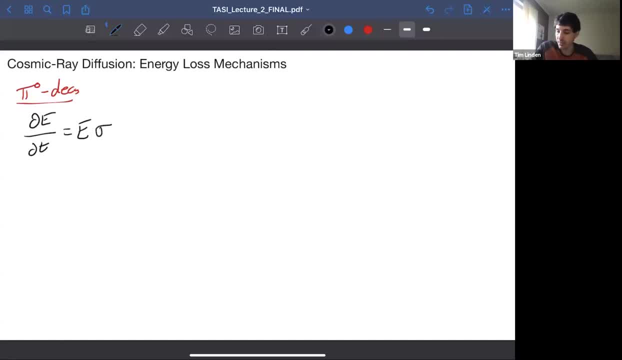 So ddT is E and then your rate is just whether that happens or not. That's the Proton-proton cross-section. This is the density of gas and then the speed of light that this thing is moving. The gas density is: 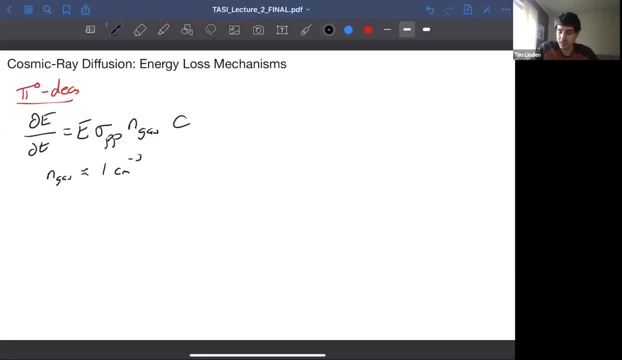 really actually very close to one percentimeter cubed in interstellar space. This is the proton-proton cross-section. It's 50 millibarns, and then you can put those numbers through and you can find the time or the timescale at which a proton finds a gas molecule in our galaxy. 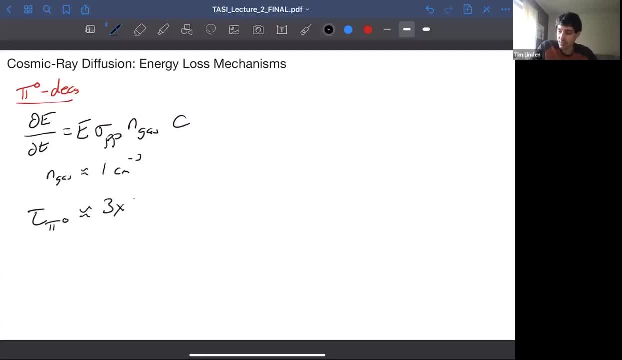 and then has a pi zero, decay and disappears. basically It's around three times 10 to seven years. You can think about maybe inverse Compton scattering There. ddT is four thirds times the Thompson cross-section. speed of light, radiation density of 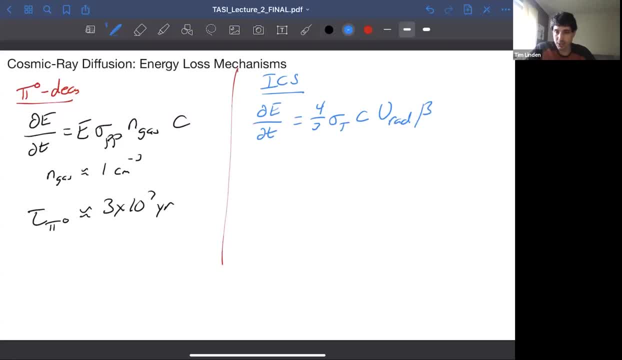 starlight in our galaxy, beta squared, gamma squared, which are just the relativistic factors. Again, really nice number to know. Radiation density from starlight in our galaxy somewhere along the plane is again one eV per centimeter cubed. 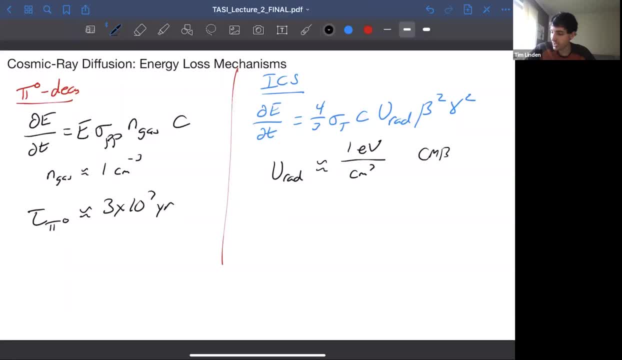 Nice number to know. Interestingly, CMB energy density- another nice number to know through the whole universe- is 0.26 eV per centimeter cubed. So these are similar. You can push those numbers through again. I'll leave that as an exercise. And you find that the timescale 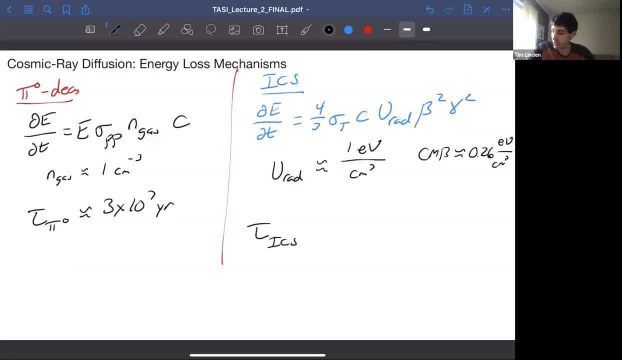 at which you lose an electron loses its energy from inverse Compton scattering is around three times 10 to the eight years. But important point, it has this energy scaling in it. Very strong energy scaling here comes from this factor of gamma, which is the relativistic factor of the electron. 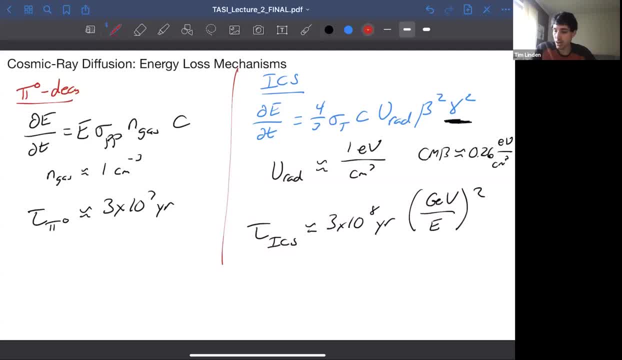 So what that means? this cross section here is energy independent, or very roughly energy independent. It has a very weak energy dependence, So low energy protons stick around, you know, on similar timescales as low energy electrons, but high energy electrons die off very fast and that's important for a. 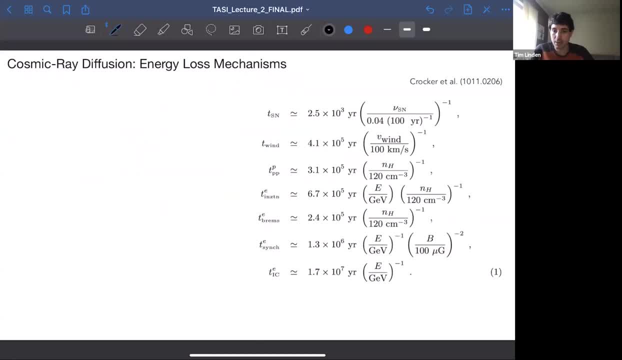 lot of dark matter searches. Here is all of these timescales. Yes, so if you thought that the so the question is just a good question. we want to find the diffusion of the particles to Earth, so why do we want to care about whether they leak out of the galaxy? So the idea is, once they leak out. 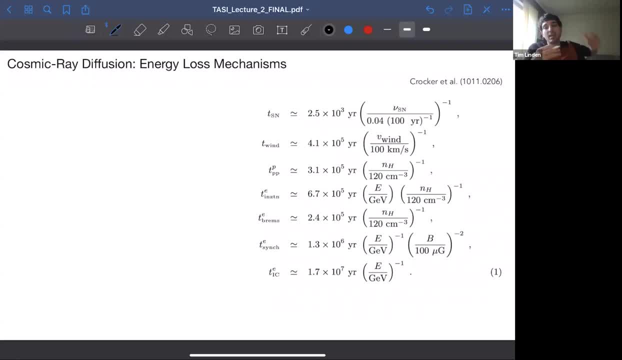 of the galaxy. they never come back again. Otherwise, if the gas density was zero- and let's say that the edges of the galaxy have mirrors that just bounced everything back then the density of high energy particles, that we would find protons, and everything would drop. 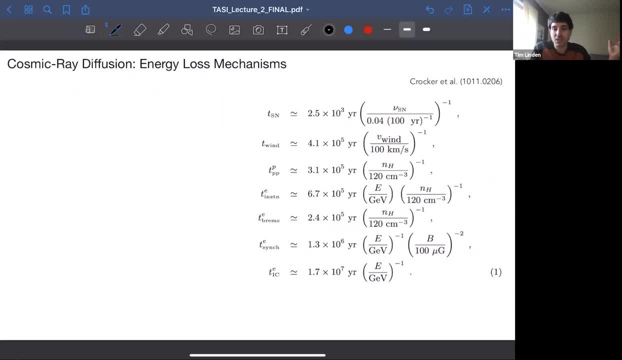 Right, be very high, because everything would just be bouncing until it finds our detector, And so you would have the whole age of the universe's. you know, supernova, all the supernova that went off in this galaxy over all the history of the universe, would still be in the galaxy, and the 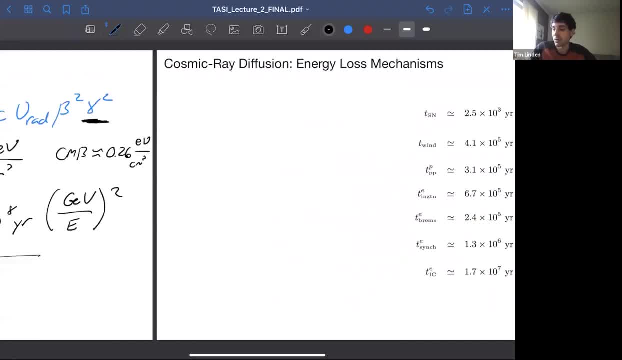 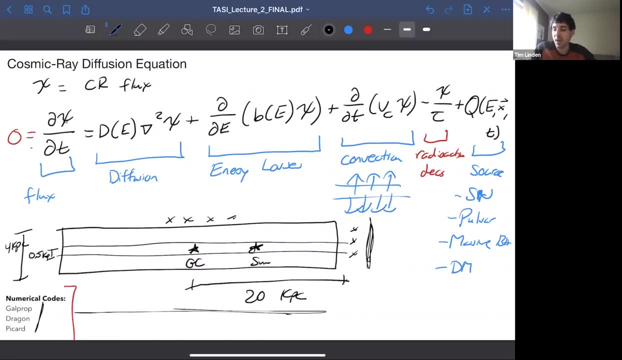 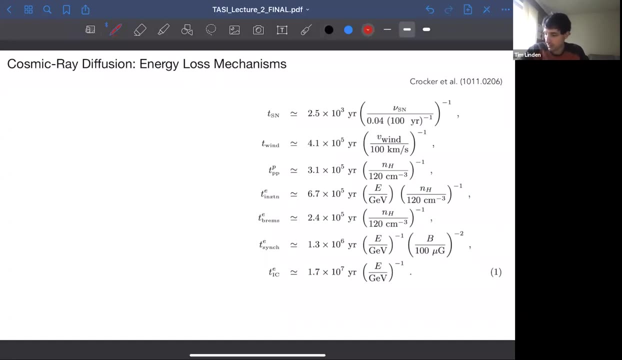 rate would be much higher than things that make Earth make it to Earth. So eventually, yes, you use all these codes and you solve them for the flux as a function of time at Earth. Okay, Here is. if people have been tracking me on the archive, they know that more than any other paper. 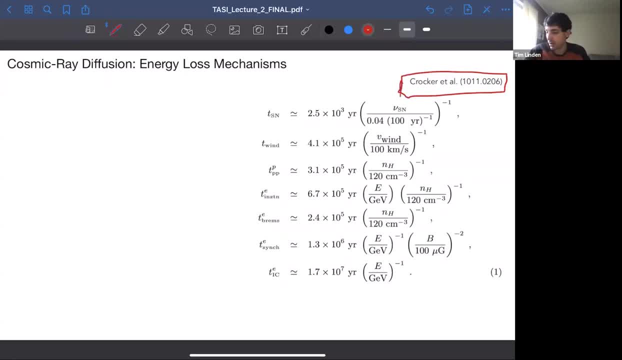 that I've ever looked at in my life is this paper called Wild at Heart: the Astrophysics of the Galactic Center by Crocker et al. And the reason is- and it's a lesson for writing papers- they have this very nice table of every single time scale. that's important, And it's in nice units and it's 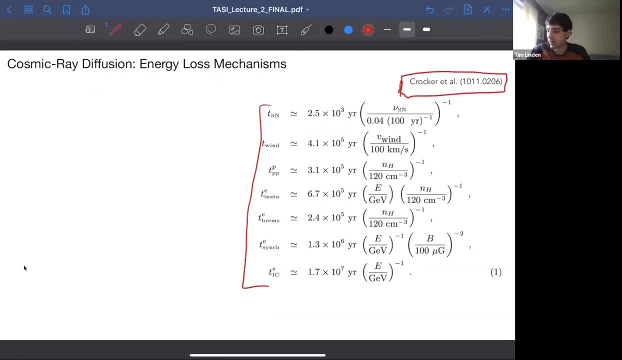 easy to memorize- or it's not easy to memorize, which is why I look at it about every other day, but it's very easy to use as a reference. The only time scale that matters for protons and energy losses is this: 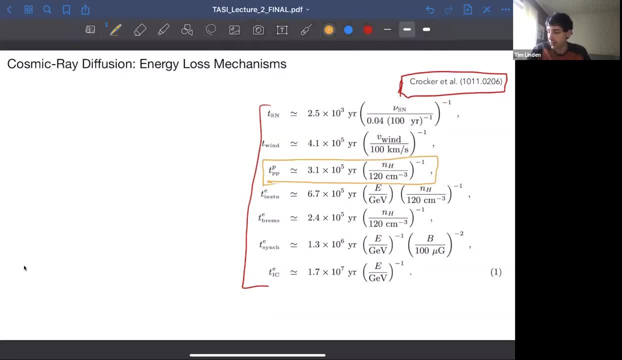 pion-decay proton-proton interaction. Here they're quoting a gas density of 120 centimeters, because they're talking about the center of the galaxy. multiply it by 120 if you want to get you know something closer to us. or, yeah, the time scale by 100. Then electrons have all of 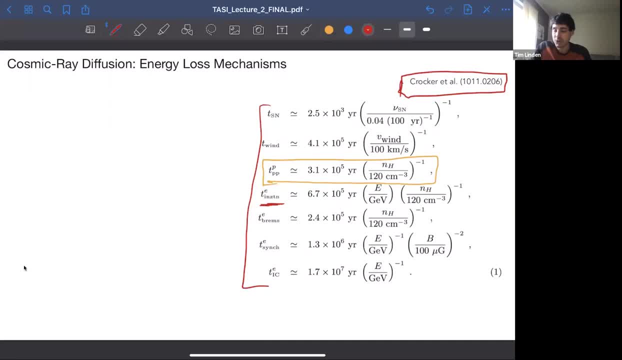 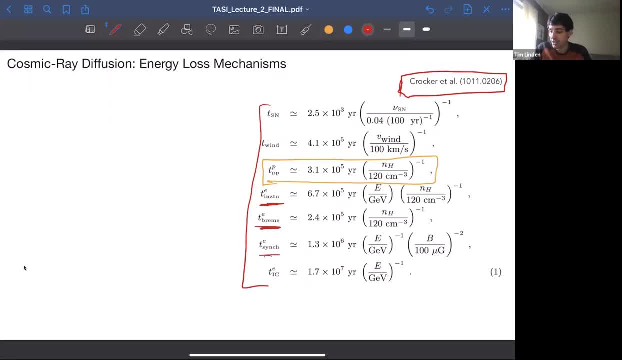 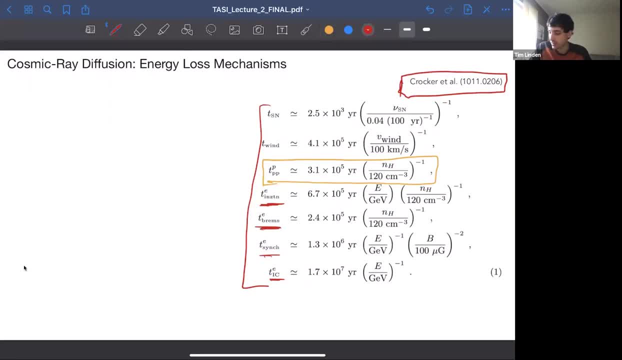 inverse Compton scattering, which both have this energy scaling. that's very strong matter quite a bit. So let's see, And this depends on the gas density here, This depends on the gas density, And then this depends on the magnetic field strength for synchrotron, And then this: 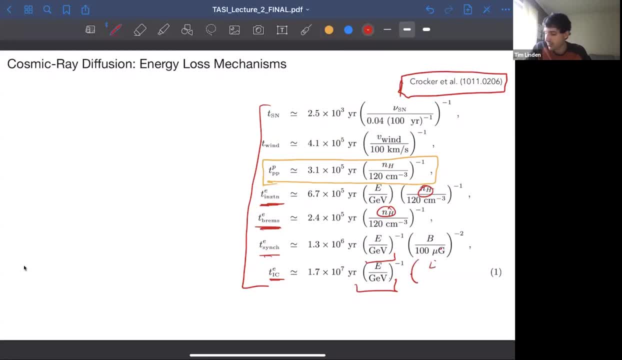 they didn't bother to write out the flux of the ISRF. I forget what number they put in here: over 1 eV or something like that. It's the one fault of this plot. Okay, That means that we can be in different regimes. 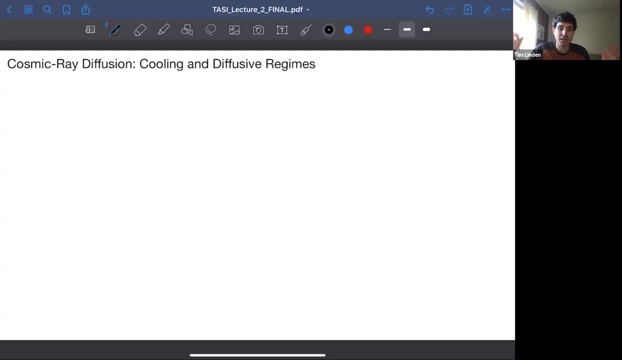 Some cosmic rays are going to cool very effectively And this is going to get to the point of why we care about all of this at the end. So I know we've kind of gone on kind of a garden path here, But we're going to get to exactly. what do we expect from astrophysics? 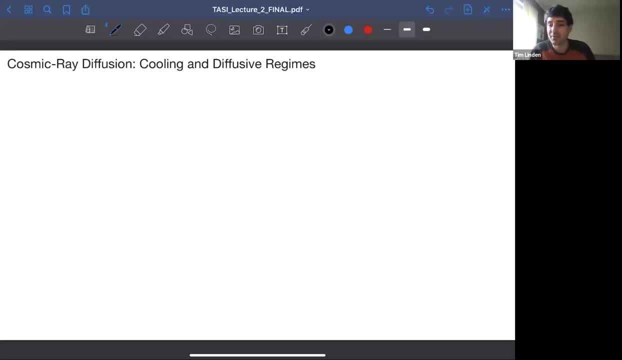 and why is dark matter going to be different here? And we're going to do it all in the next 10 or 15 minutes. So we can be in a diffusive regime where the particles aren't losing energy, They're born and then they just escape from the galaxy, Or we can be in the cooling regime, The 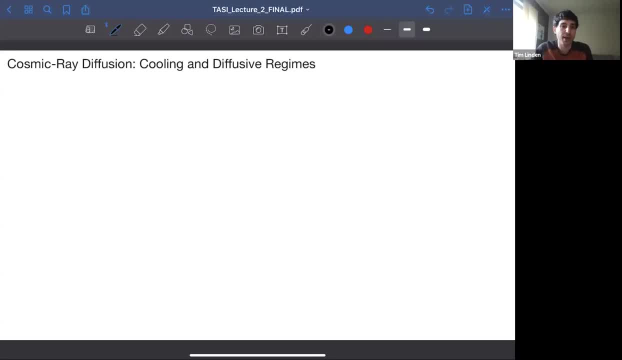 particles don't escape from the galaxy. They cool and lose all their energy before they make it to Earth And those are going to give us a different spectra that we care about. So in general, if I want dnde for some particle Is equal to some source term. And then some term for how long these particles stick around, Right, Which is you know what sort: 26 00.01. 40.41elsdnn. air Mars, soilibi fa que 2,3 nu r2,nit CarmeinC Следdor, second calcium pressureí,0.9mH. 0.7m. 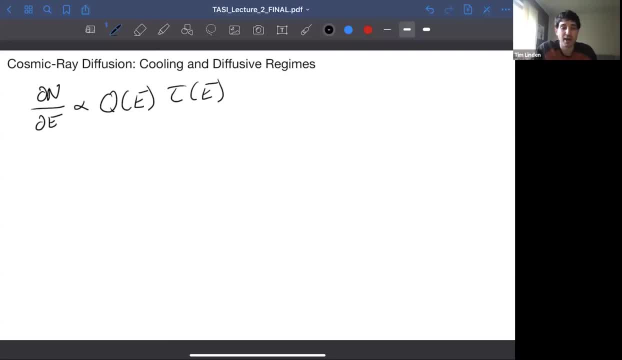 which is the same as saying we said before, particles that stick around a lot longer, you're going to have a lot larger flux even for the same source If you have diffusion out of the galaxy being the reason that you lose your particles. 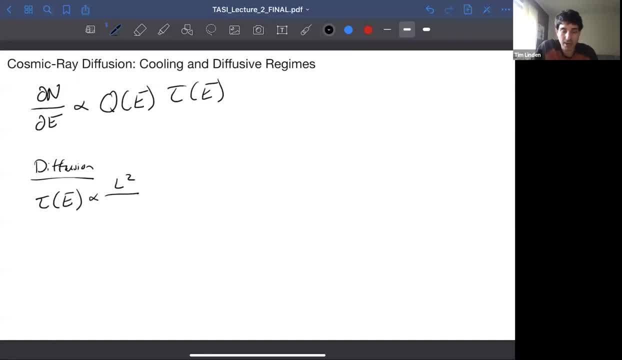 then that time scale is proportional to the halo height you're escaping out of over that diffusion constant, that step size And what we said. this is just some constant. So this is equal to constant And dE has some proportionality of E to the minus delta. 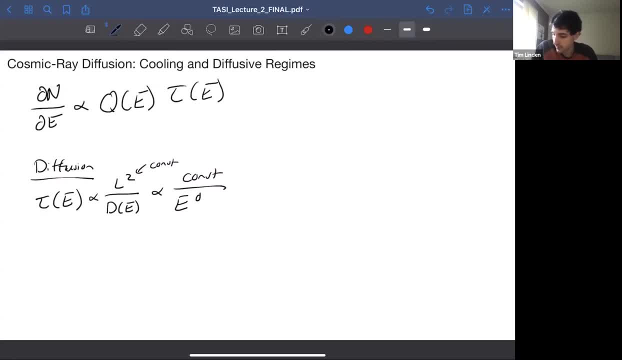 Sorry, the diffusion constant is E to the plus delta. High energy particles have bigger gyro radii so they move more effectively through the galaxy, which means this time scale is proportional to E to the minus delta, which means I need to soften by some number. So the average particles that are getting to me. 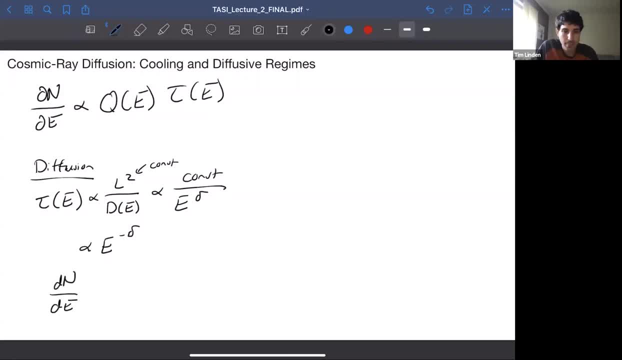 dN. dE is proportional to E, to the minus two from first order Fermi acceleration, or maybe 2.2 from second order Fermi acceleration minus delta, where delta is maybe 0.3 for Kolmogorov, 0.5 for Krachian And you get something. 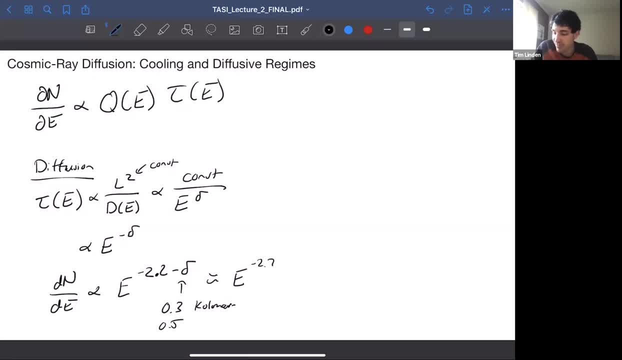 when you do all this correctly, of around d to the minus 2.7.. And that is the spectrum of cosmic rays. We had a little bit of a break there. So that's the spectrum of cosmic rays We actually observed for protons. That tells us that protons diffuse out of galaxies. 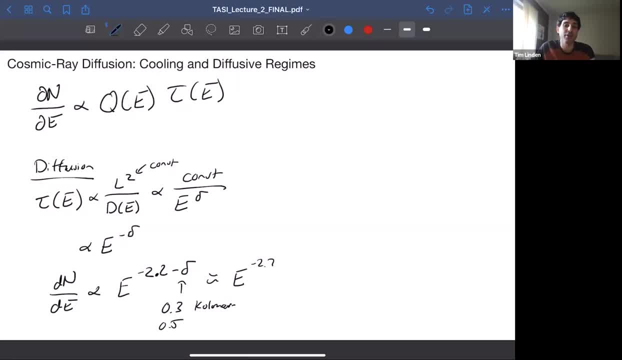 Most protons don't interact with gas in the Milky Way before they escape. Most of them make it out faster And we know that because of the spectrum, Cooling regime is slightly more complex. here, because you have to worry, It's actually the question that was just asked. 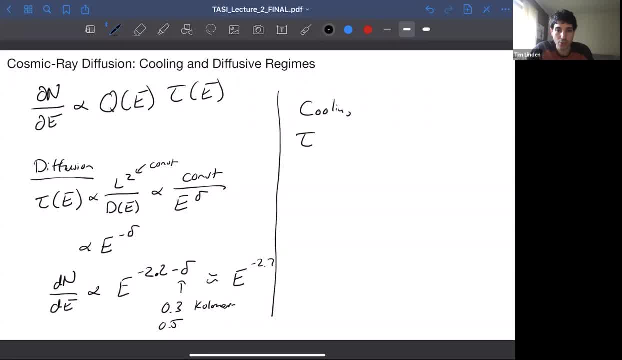 You need the particles to not cool all the way that they disappear, But before they disappear you need to cool all the way that they disappear Before they diffuse to us. So the faster the diffusion, the harder the spectrum for the same cooling rate. So the time that you get, if you do the calculation which I'm not going to do here, 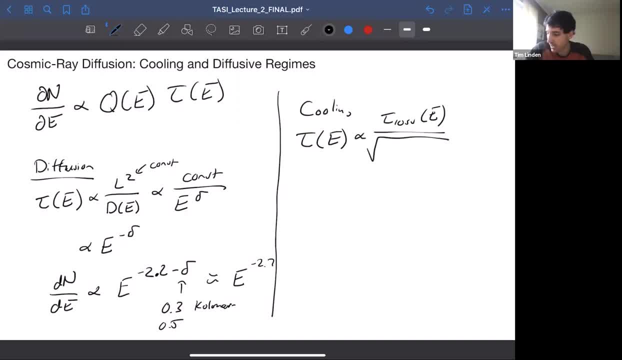 is that it goes as the energy loss timescale divided by the diffusion constant times, the energy loss timescale, the square root of these two things, And so this becomes proportional to E, to the minus delta over two minus, let's say gamma. 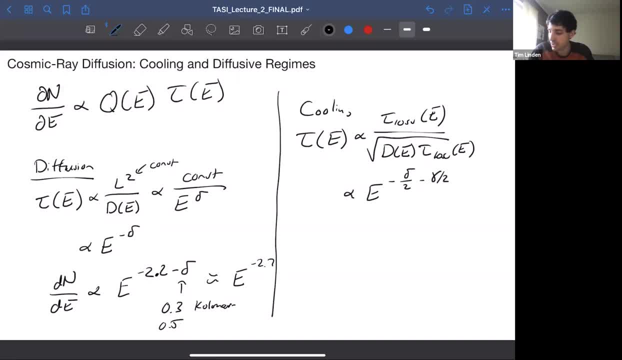 Over two, Where gamma is the energy loss timescale that you get from these different calculations for what is causing your energy loss. So for electrons, Tau of E is proportional to E, to the minus 2.2, because they're accelerated by supernova. 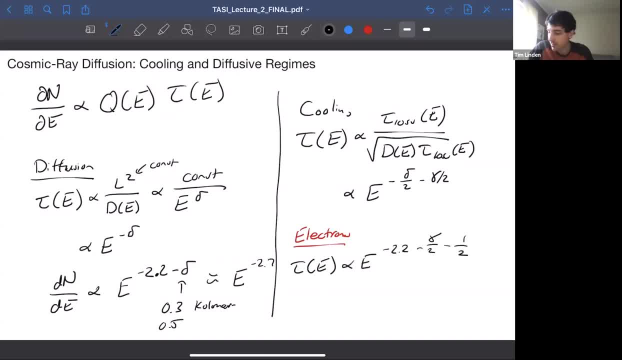 minus delta, over two minus one half. That's from that synchrotron energy or synchrotron energy. So that's the energy loss timescale that you get from these different calculations, And so these tend to have spectra that are around E to the minus three ish. 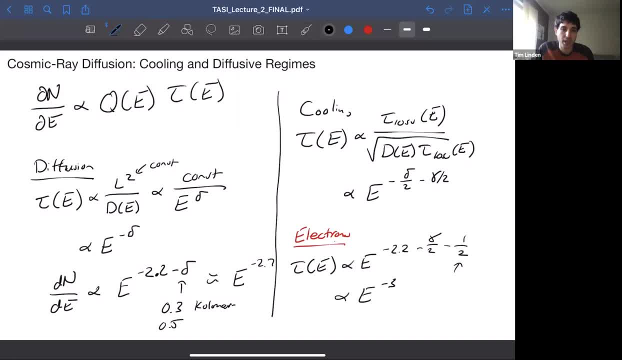 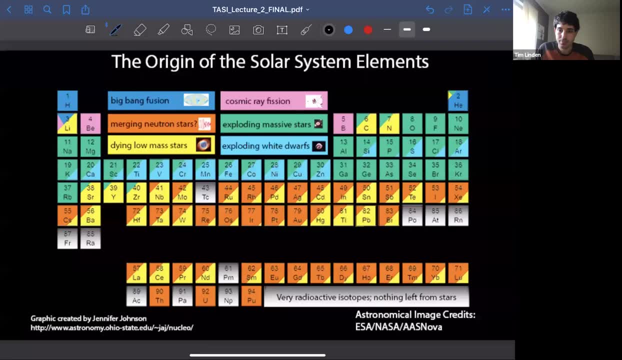 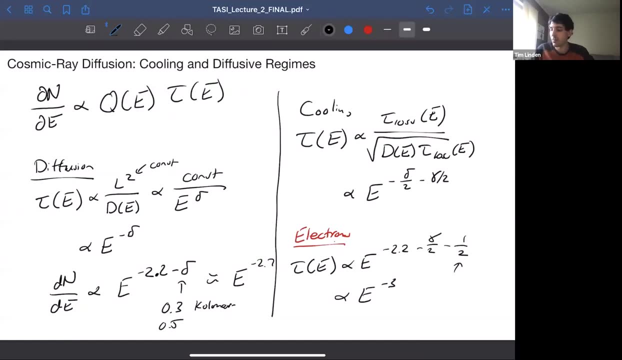 Right, So the electron spectrum is observed to be softer than the proton spectrum, And this is because electrons cool in a different way, Sure, So explain the cooling regime in a little bit more detail. Right, So I have an electron that's produced at some energy E. 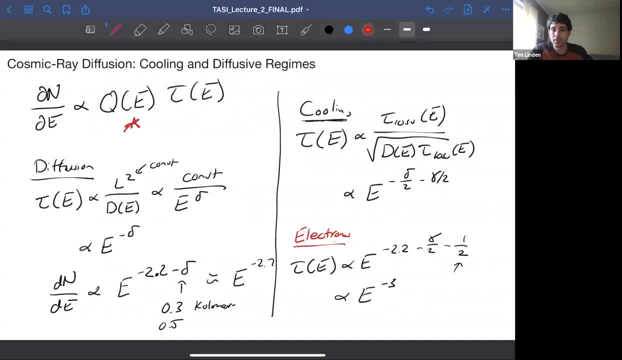 So that's my Q of E term And I want to see how many electrons do I have at energies, you know, E minus delta, E, where that's some small energy scale that I care about based on my energy injection spectrum of electrons. 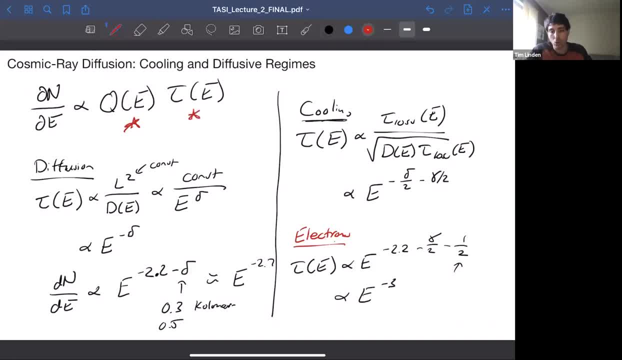 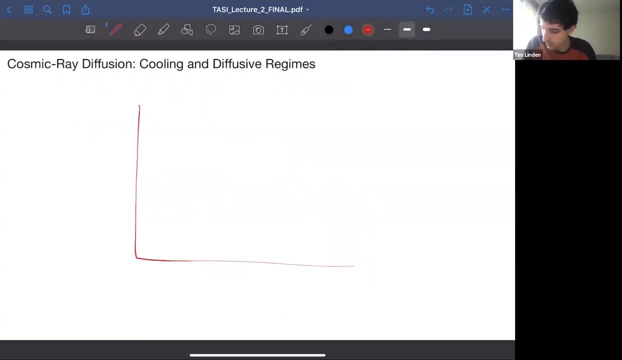 And so that depends on how many, how much they cool before they make it to me. So in real life, you know you'd start with some. I said I'll try to follow. Well, let me. E is a function of E. You'd start with some injection that looks like this: 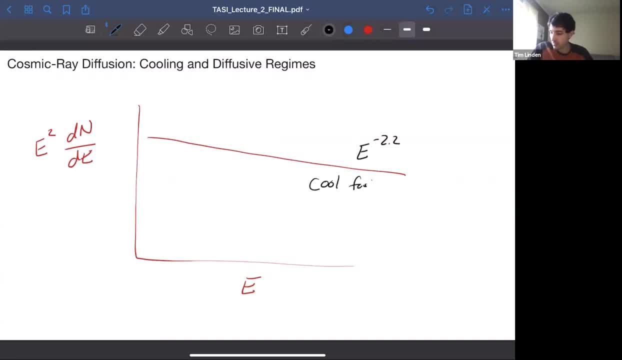 But these things cool fast, These things cool slow. So in a cooling dominated regime, some of these things have come over this direction. These things are basically stuck around. So you'll get now some other spectra. So this is E to the minus three. 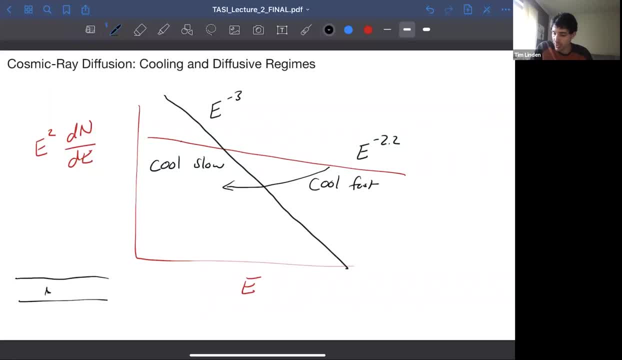 So the spectrum, you know the cosmic rays, are born over here when some supernova goes off with this spectrum. But by the time they make it to this check mark over here, they have cooled quite a bit And the spectrum has become softer. 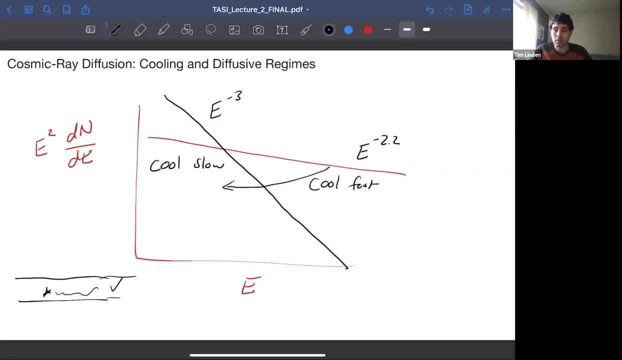 Should TALV be dependent on the position of the Earth from the sources? Yes, certainly, If things are totally cool, if things have cooled all the way- and this is maybe worth calculating on your own- you just law just converts to another power law. So if you undergo four cooling time scales, 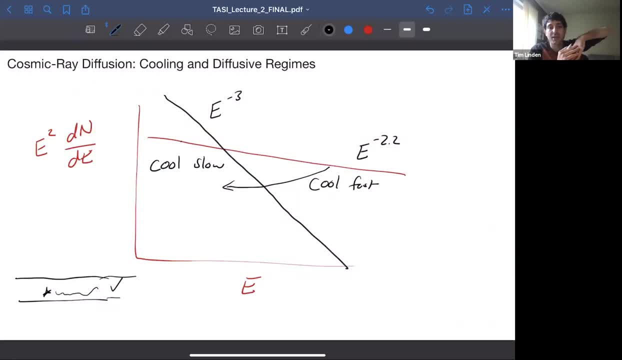 ten cooling time scales, a hundred cooling time scales. you keep the e to the minus three spectrum and the total amplitude of it just goes down. But also you know, when you do these on numerical codes, you calculate where all the supernovae are in the galaxy, or you know some approximation of 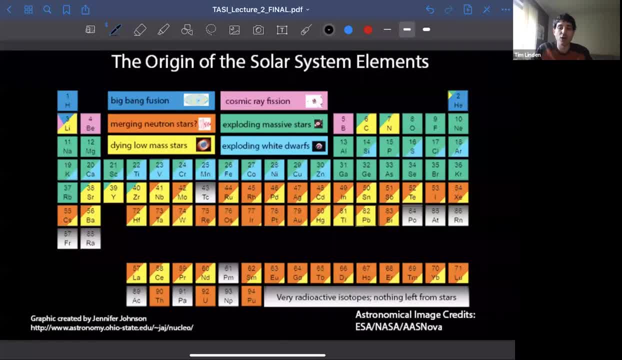 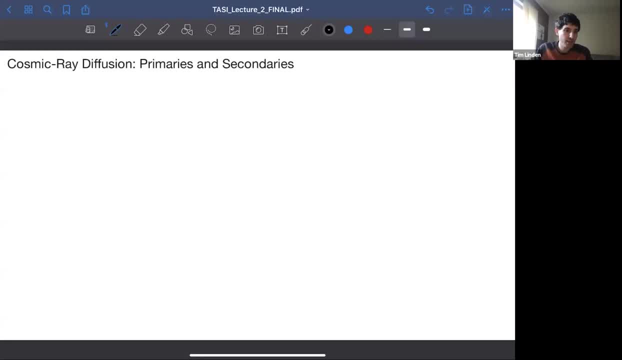 that and then do the calculation. that way, Some of them are quite nearby, and then the spectrum from them will be harder. Okay, And then the last thing in the few minutes I have left is thinking about primaries and secondaries. Primaries are produced by sources. 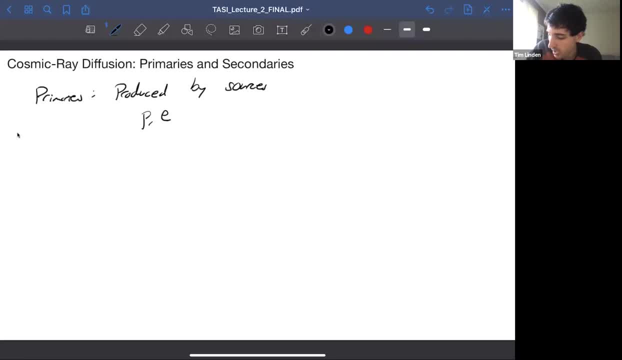 So these are the protons, the electrons, the helium atoms, etc. Secondaries are produced by interactions, So this is positrons, for example, proton plus. proton goes to junk plus E plus is normally thought of as a secondary. Same thing with antiprotons: it's a secondary. 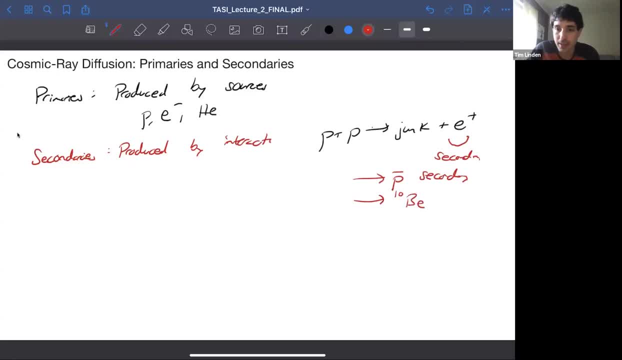 Same thing with beryllium is a secondary coming from the spallation of carbon, etc. And the first thing that's interesting right, is that secondaries are produced with the steady-state cooled spectrum of the primaries, So dN, dE. 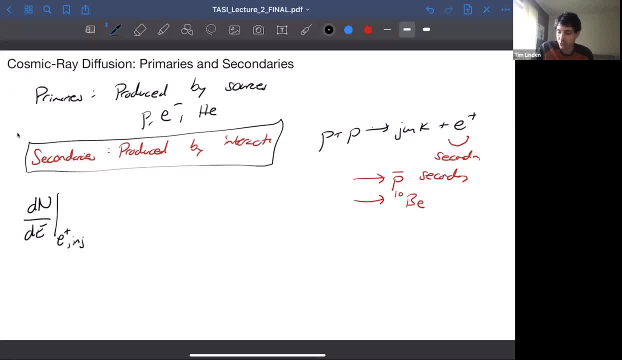 of positrons that are injected because they're produced by protons that are already cooled. they're injected with a spectrum e to the minus 2,, 0.2 minus delta And then they cool because they're produced not near where we are and we're, like we said, electrons cool relatively rapidly. 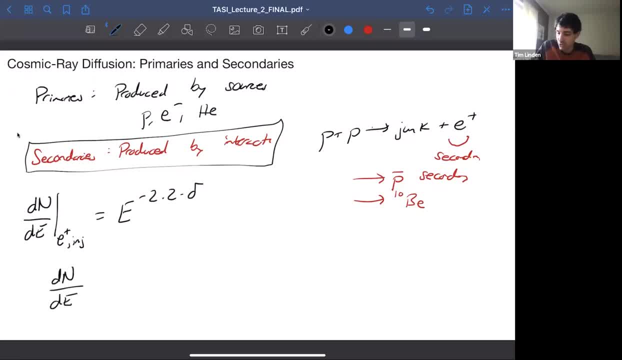 So the spectrum of positrons that is expected to reach Earth is e to the minus 2.2, minus delta, minus delta over two from the electron cooling, minus one half Another way. but the electrons are produced mostly as primaries. There's a bunch of electrons. 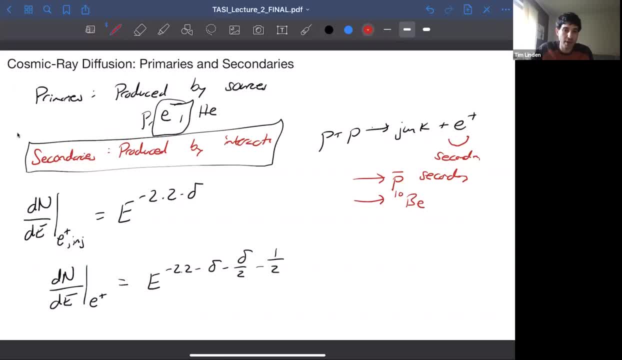 near supernovae and so they get accelerated. This is a supernova-only picture and I'm not dealing with them, So we'll get this guy Chekhov Laiz pointed out. Here's one of the main Weather-Med spacecrafts, which is used mainly to detect electric electricity light resistors. 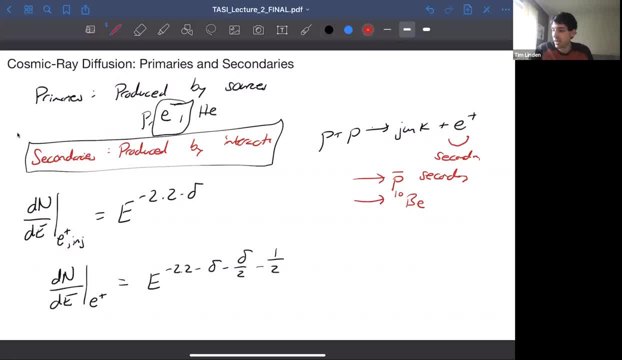 And it's actually driven by a ne viruses. so it's essentially powered by an electron behind the surface of an electron. So even if you scrape one with the spectra and makes it dark- and I'm not dealing with the pulsars yet- We're going to talk about that a lot next lecture. 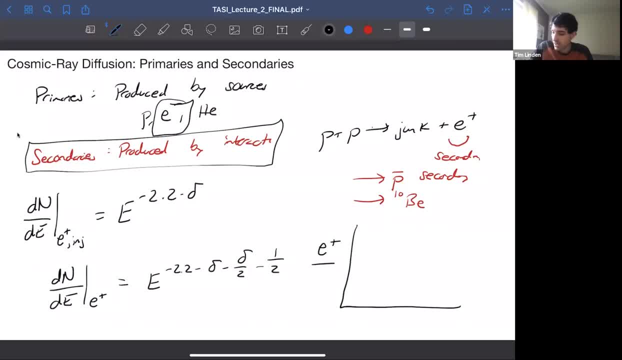 And what that means is that the spectrum of positrons divided by the spectrum of electrons should have fall as e to the minus delta over two. Sorry, e to the minus delta, Because it is getting this extra injection from the protons, so it has a softer spectrum. 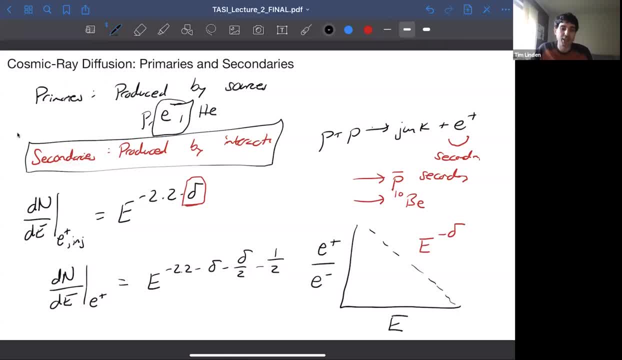 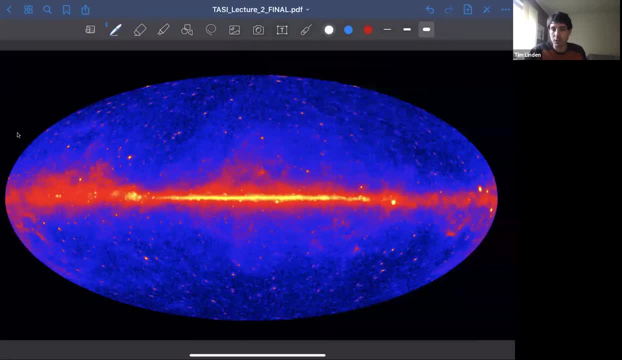 Which means this is the astrophysical expectation. It's just some smoothly falling spectrum. So let's hunt for dark matter against this, And I'm going to just give a picture of what we're going to do in the next lecture. This is a map of gamma ray emission over the galaxy. 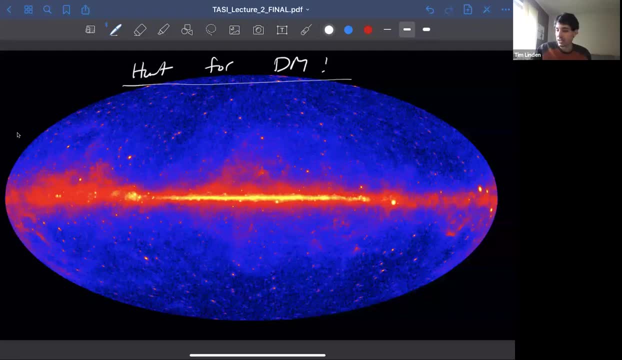 And we're going to look at all of this astrophysics which we're modeling. It's supernova going off, maybe here Protons. everything diffuses out. of. here It interacts with gas along the plane of our galaxy. here It produces gamma ray emission. 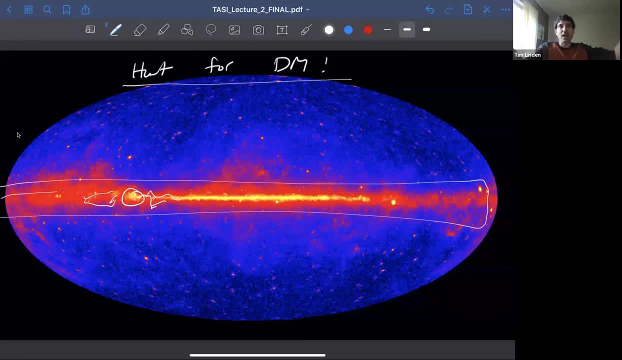 That gamma ray emission comes to us. This is us looking out over the whole universe, so we don't exist anywhere on this plot. Or maybe some of these produce electrons and positrons and then they diffuse somewhere around here? How do we look for dark matter on top of something that looks like this? 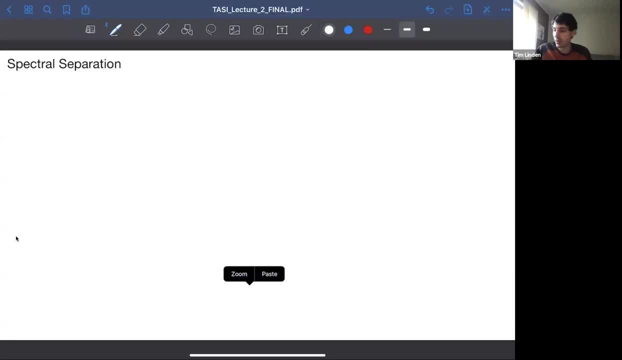 And a couple ways we do that are, first off, what have we learned so far And what can we do? What can we do with the spectrum? What did we learn We learned? the backgrounds are powerless. Something that's about e to the minus 2. 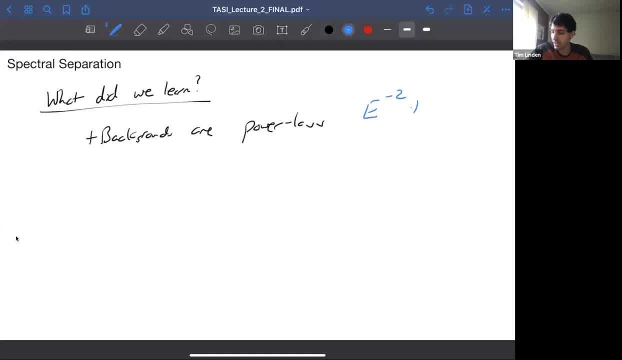 for first-order Fermi acceleration. if you're really near the source, to e, to the minus 3 or something like that for electrons and positrons, that might make it to Earth after they cool. But in any case these are power laws over many orders of magnitude. 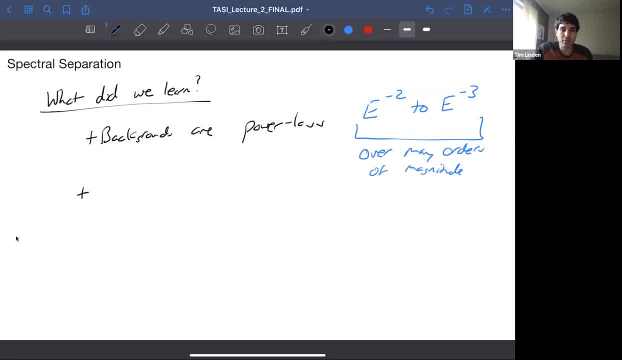 Dark matter, on the other hand, is not a power law over many orders of magnitude. We know that dark matter is non-relativistic And mass of chi in our WIMP models is around, you know, 100, let's say: 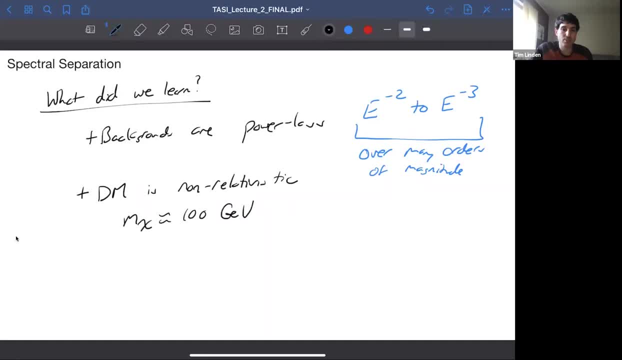 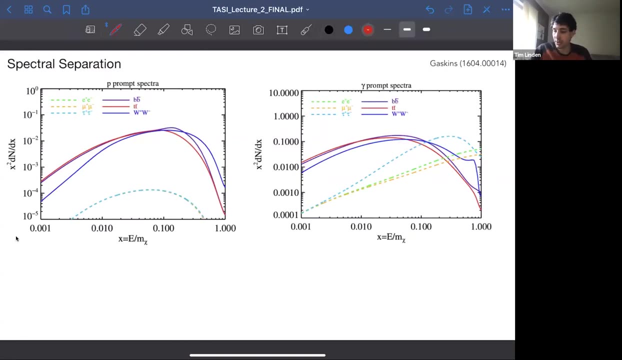 let's just say around 100 GeV. give or take some orders of magnitude So we can look for spectral bumps. This is what that might look like in some detail. So here is these results I think are from the code PIPIA. 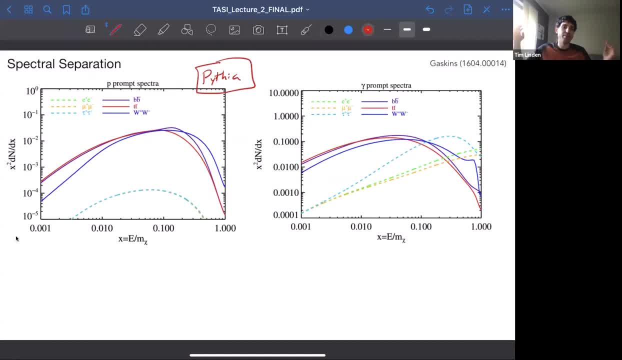 which is a particle production code. You have dark matter. annihilation basically works like electron-positron production. So electron-positron colliders produce whatever your mediator is. The mediator decays to say bottom quarks, top quarks, W plus, W minus. 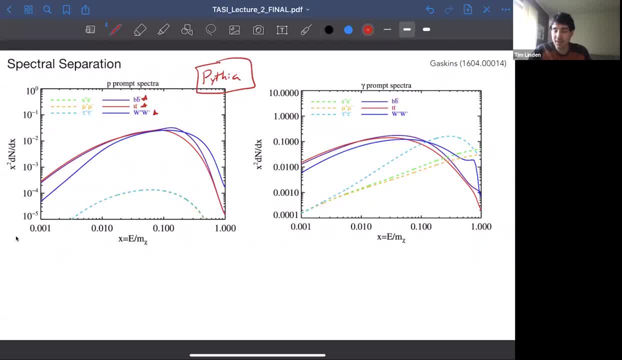 or some sort of you know taus or anything like that, And then you just let those hadronize or do whatever they do. Let's explain this plot in a little detail. This is x- e divided by the mass of the dark matter: particle. 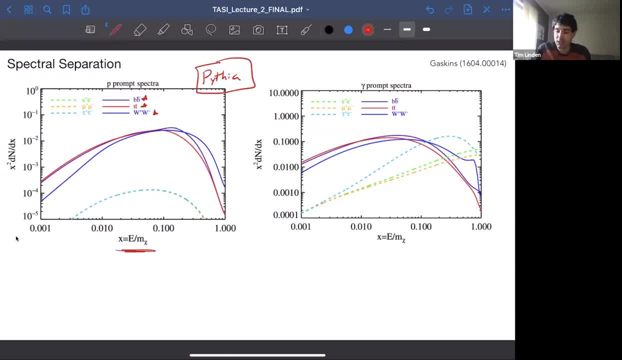 So if the dark matter particle gets a factor of two higher, this energy scale just goes up by a factor of two. Then this is e squared d n d e. So what you see is this bumpy non-power law structure in e squared d n d e. 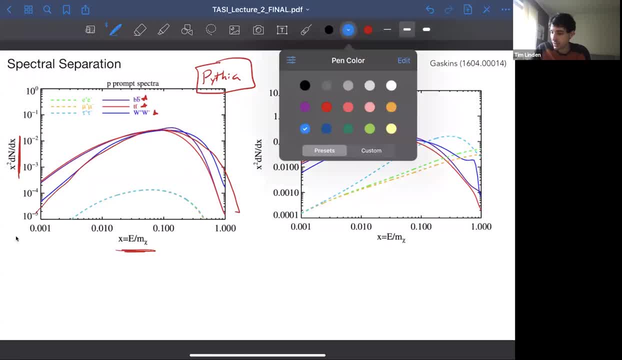 Remember, astrophysics on these units should be doing like e to the minus 2.7 or something like smoothly, like this Right. So most of the power for dark matter comes out in protons at about one-tenth of the dark matter mass. 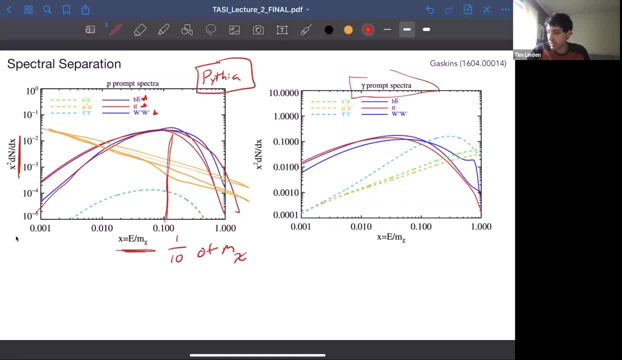 What about gamma rays? And now we can look at different final states again, depending on what the dark matter interacts with. That's what you get to do as a model builder. Again, the power comes out here, let's say between. I usually think of it as about one-twentieth. 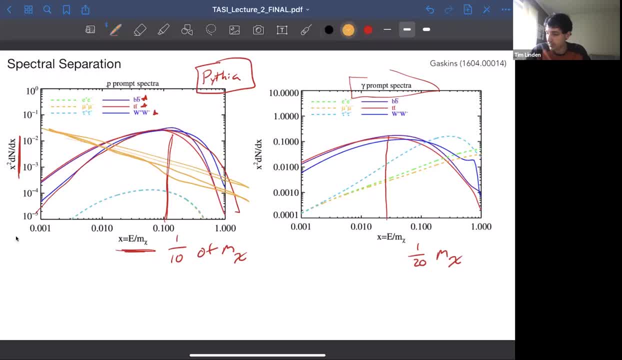 of the dark matter mass, And again, the spectrum should be something that looks kind of like that. So we're going to look for bumps over that. That's the first thing we're going to do. Second thing we're going to do is angular separation. 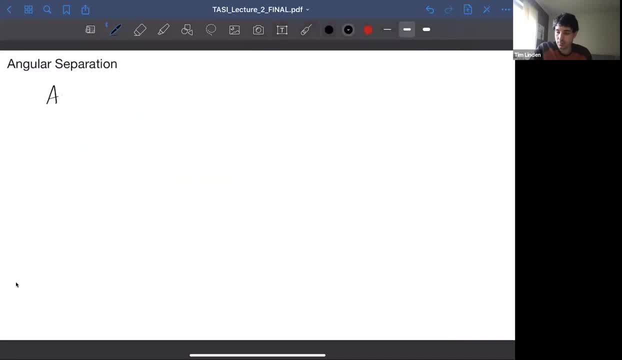 What do we know? We know astrophysics is bright. Supernovae are big, bright things. The power of pulsars we learned was extraordinarily high. It's bright where the supernova pulsars are. It's bright where the gas is dense. 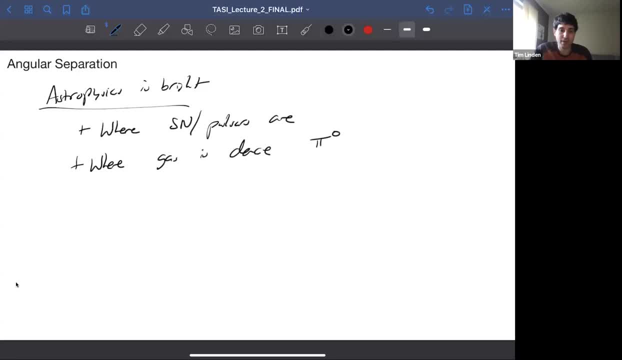 Because that's where you have pi zero decay, which is the brightest part of that signal. And it's bright where you know where starlight is bright. We might want to avoid those regions. Dark matter is spherically symmetric, So look. 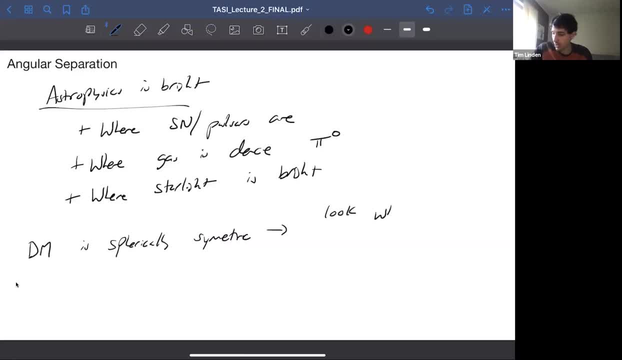 where Tm over astro is high. I don't know why is high is in the denominator. Okay, And so the very last calculation I'm going to do today, And so I'm going to keep everyone here just about five more minutes. I apologize for that. 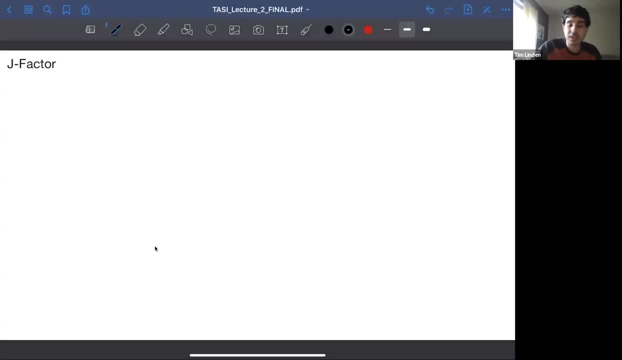 But if you want to leave, you can leave. No one will notice. So the J factor is the astrophysical part of dark matter annihilation. So what goes into looking for dark matter at some point in the sky? The dark matter cross-section. 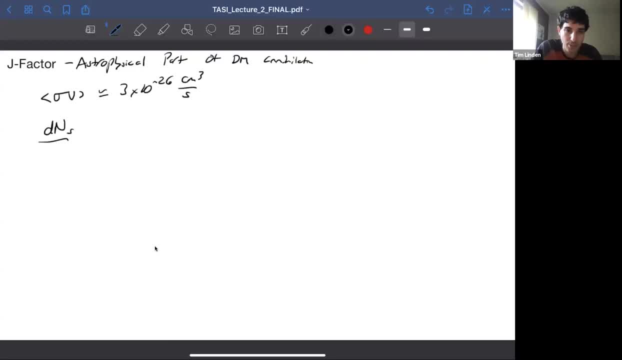 The number of particles of the standard model particles you're looking for as a function of energy, And the number density of dark matter square, which is a row squared, So you can separate this out and say that the flux of some standard model particle you're looking for is a number of particles. 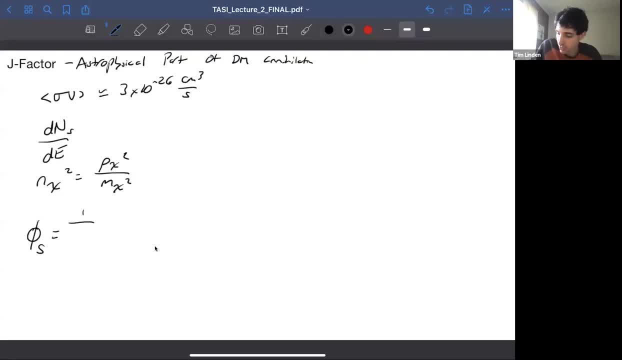 What you're looking for from dark matter annihilation is equal to one over four pi And it's just a steradian measurement that comes along Sigma V over two times the dark matter mass. Remember this is because two dark matter particles are needed to annihilate. 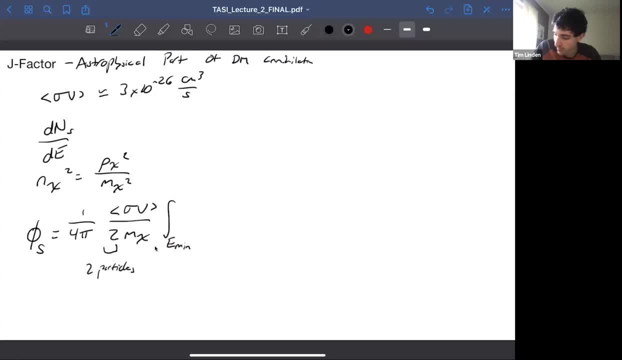 This is some energy region that we're looking at, from energy min to energy max of dn, the standard model Particle that we care about, dE, dE. And then we're looking at some region of the space of space. So we're looking maybe over some angular region. 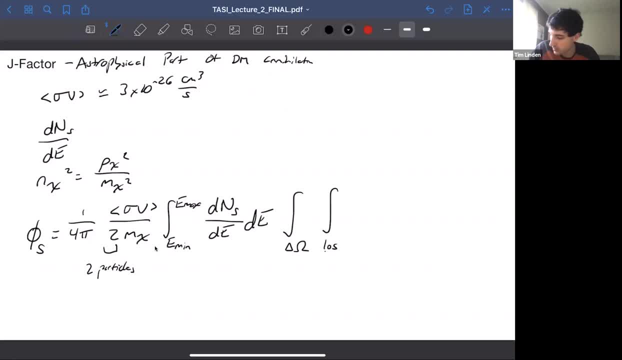 We're looking over a line of sight. This is important because with the telescope we generally don't know how far away something is when we're looking at it. So if I look out for my dark matter in some direction here, I see the dark matter annihilation that happens here. 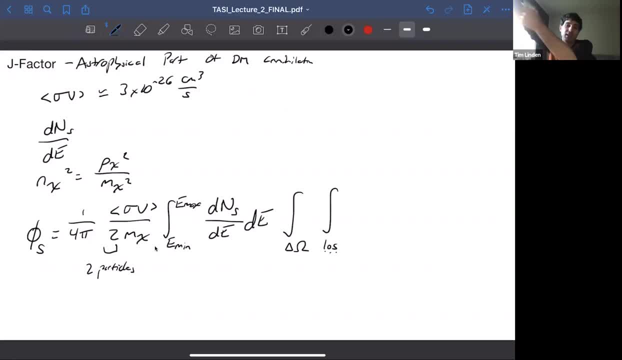 And I also see the dark matter, annihilation- that happens here, And I see all the astrophysics. that's along that line of sight too. This is rho squared, So this is the distance here of wherever I am along my line of sight. 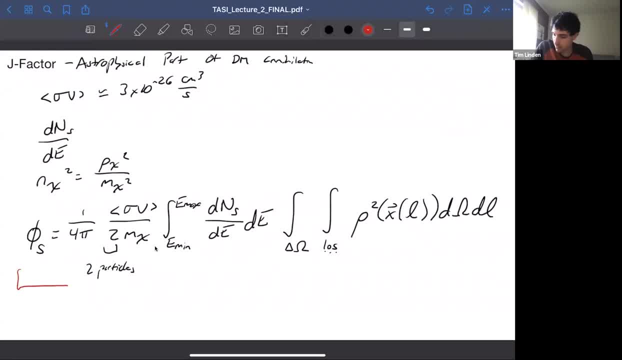 And what's really nice is that this separates oops Stuff from here to here is particle physics And there's no astrophysics there. That means that this is the same everywhere in the universe, Unless you have your dark matter model change. 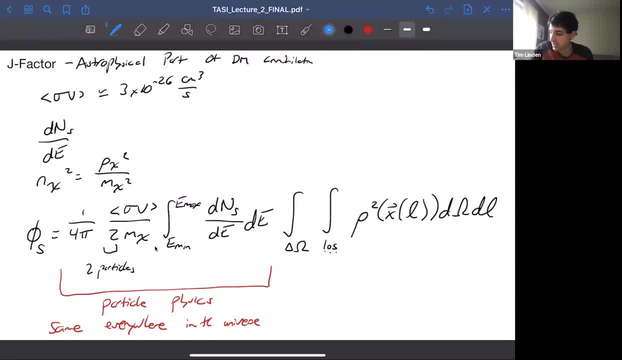 as a function of cosmology or something like that, But at least in a galaxy size scale. that's the same everywhere, And this is astrophysics. Why is dark matter spherically symmetric? Because it can't the reason baryons form a plane in the galaxy. 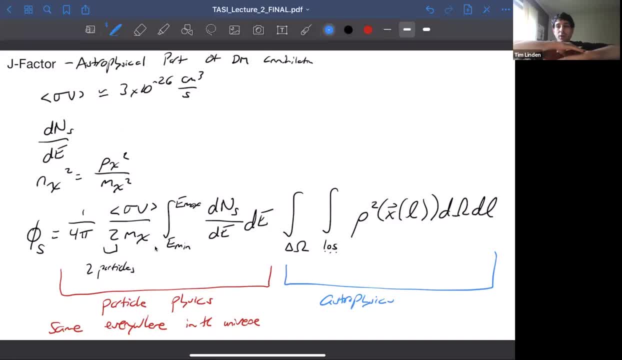 is because they can have inelastic collisions where they shed photons and lose angular momentum, And that allows things to collide And that allows things to cool, And because of turbulent cascades, where things cool, they start to form a random plane. The reason for that is electrons are coming in. 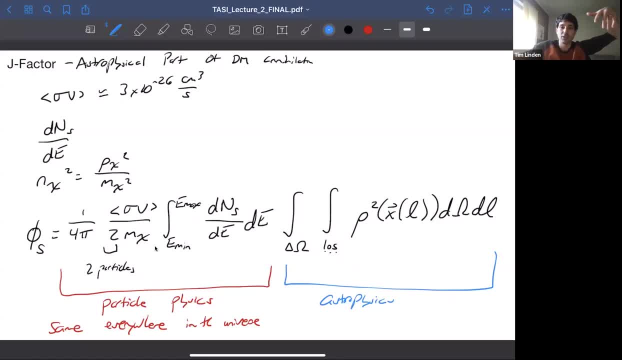 they're like gases coming in from all directions to form a galaxy. If you cool a little bit more effectively along this plane at the beginning, things get a little bit denser here. They fall in farther. That blocks light, which makes the things out on the outskirts here colder. 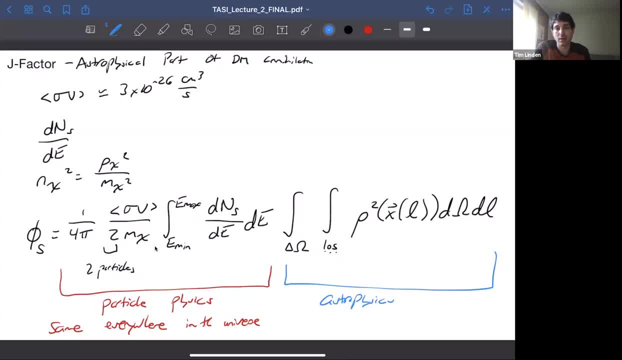 And then things more effectively fall in this direction again as well. So over time, that's how you form a dish. That's how you form a disk. galaxy Dark matter can't do that. It can if there's a dark photon or something like that. 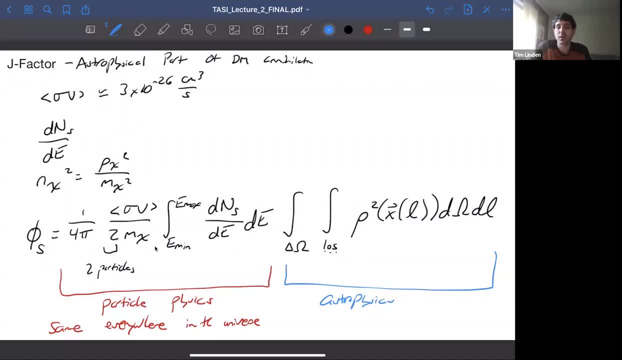 But in general you can't do that, And so you form spherically symmetric profiles. So this is all astrophysics And it doesn't depend on the dark matter model. So in general, you could go out and just do gravitational studies. 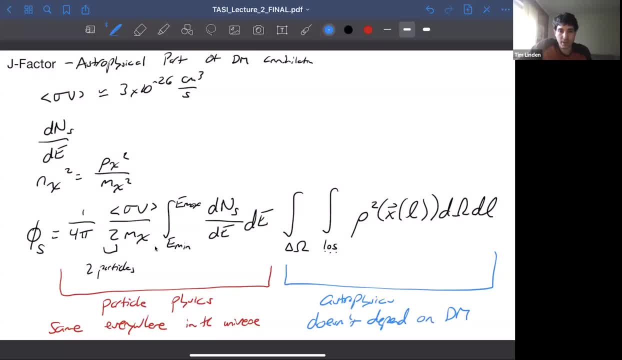 of where dark matter is, Look at dwarf galaxies or something like that- And you could calculate all this stuff and then apply it to some particle physics model you want to deal with. Alternatively, if you have two different sources, you just put in the particle physics model. 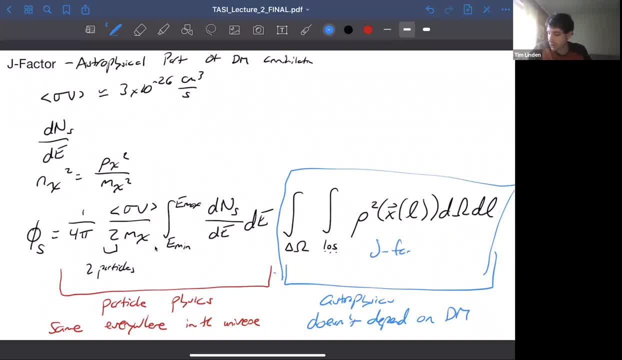 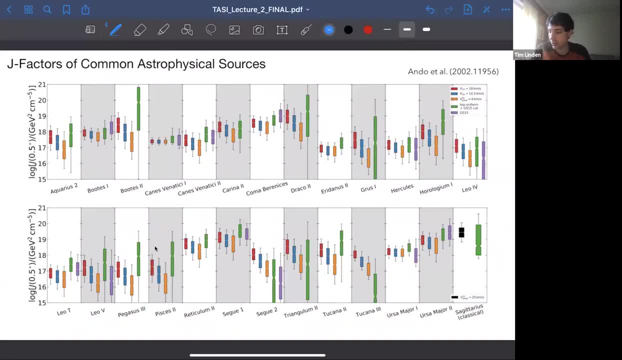 and then the difference in these observable things- and this is what is called the J factor- tells you how much signal I expect in one area versus the other. And to close, these are just some different J factors of common sources. These are dwarf spheroidal galaxies. 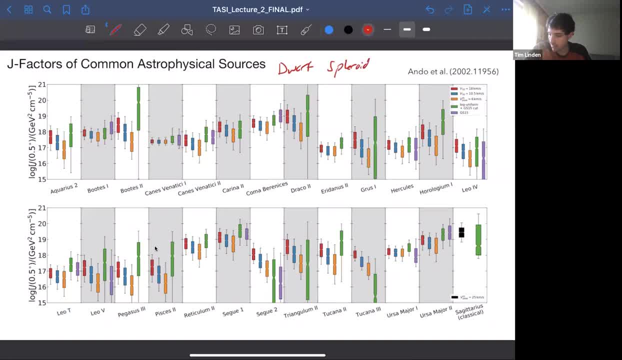 in the Milky Way with big air bars And this J factor is on the order of 10 to the 17, up to 10 to the 20 or so, And the units of this J factor are weird but you can calculate them at home. 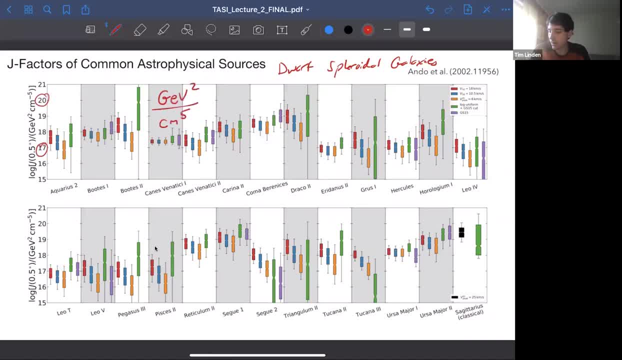 Gv squared per centimeter to the fifth, And you multiply that by sigma v, Sigma v has units centimeter. third, per second. You multiply it by 1 over the Gv squared from the mass of the particle, You'll see it all works out. 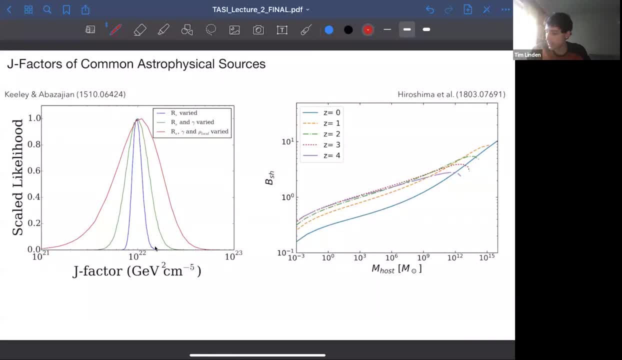 This is the J factor of the galactic center. Here it is on the order of 10 to the 22,, which is a much bigger number. This is just the likelihood ratio of different models, And then this is basically a substructure. 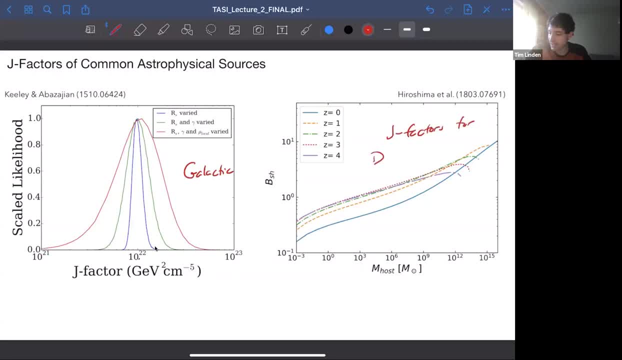 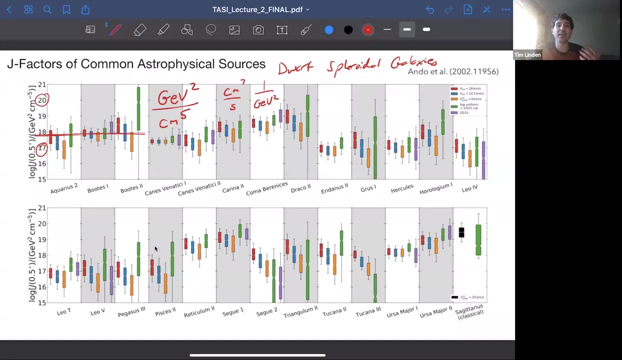 which gives different J factors. This is proportional to J factors for distant galaxy clusters. There's not a number here, But let's compare that like 10 to the 20 to the 22 to 10 to the 18 or something here. 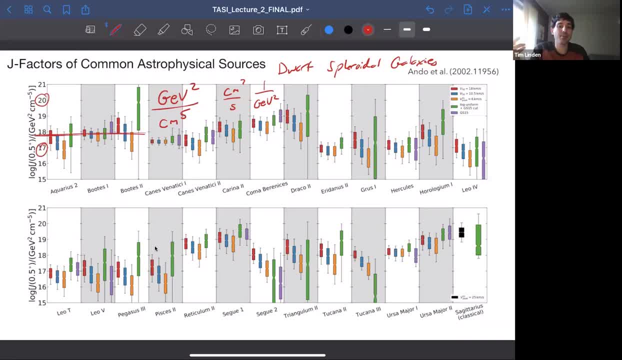 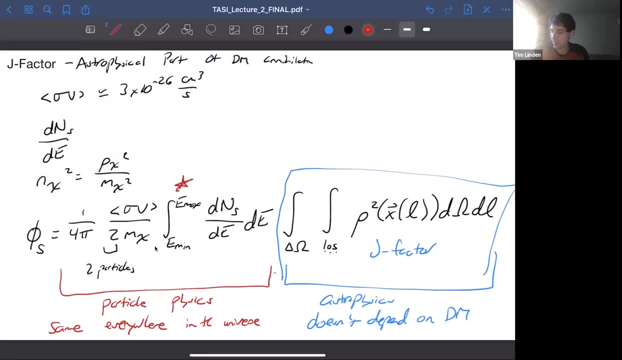 That means if I have any signal that comes in dwarf-steroidal galaxies and I say it produces 12 photons, I'm supposed to see. it produces 12 photons, I'm supposed to see, because I calculated this. I just apply the ratio of these two J factors. 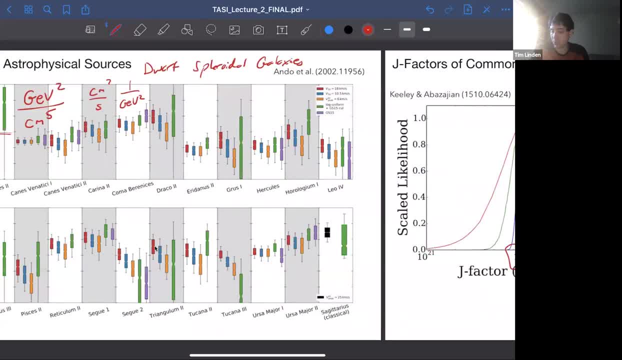 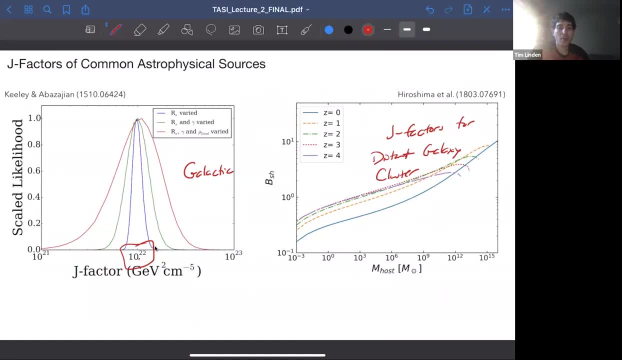 between the dwarf-steroidal galaxies and the galactic center, and I say that it's supposed to produce 10 to the 4 times as many photons at the galactic center than it is at dwarf-steroidal galaxies. And so I just get to. 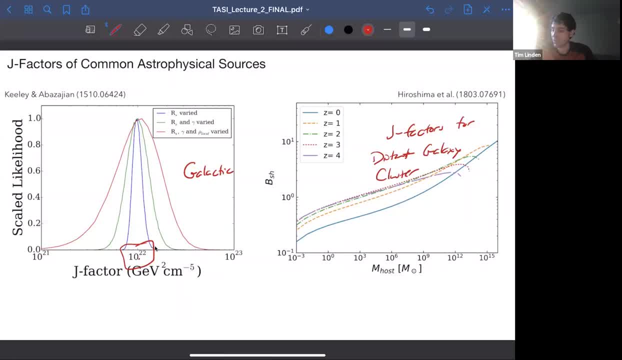 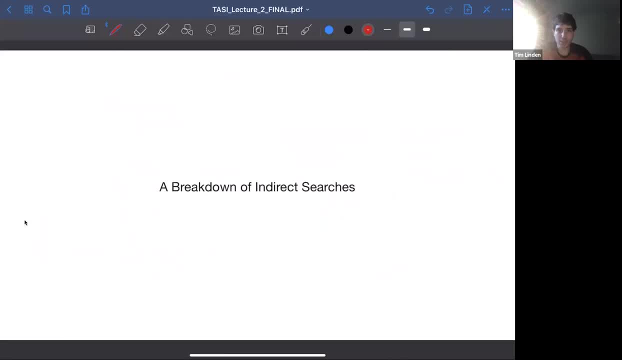 calculate these ratios in different astrophysical systems. So that's what I'm going to close with for today. I'm already over time, But we know now what astrophysics is supposed to look like. We're supposed to get power laws of cosmic rays. 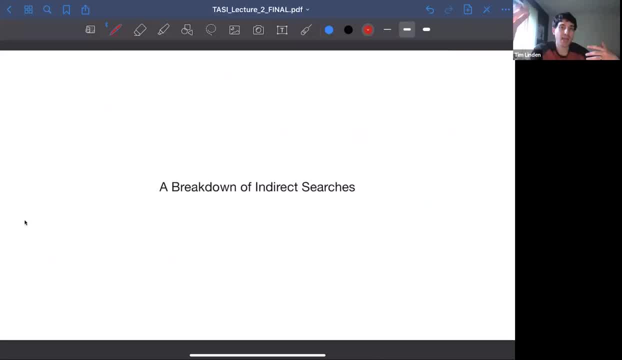 primaries, secondaries that are accelerated to high energies. Then they interact and produce gamma-ray emission that we can see, And in the next talk we're going to go over all of the different things that we can potentially observe. We're going to do a status. 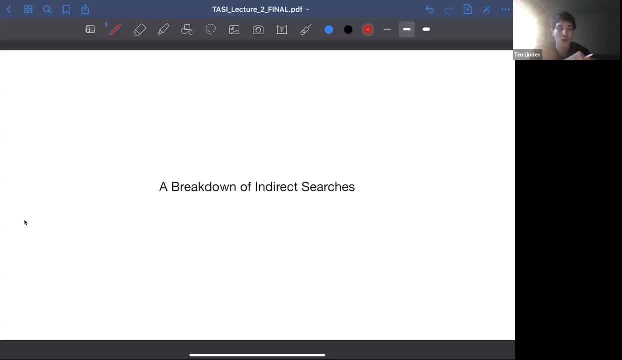 of all of the current indirect searches that exist in the literature, looking at things like gamma rays, neutrinos, cosmic ray searches, searches with gravitational waves and things like that, And then we'll also look at maybe how these apply a little bit to non-. 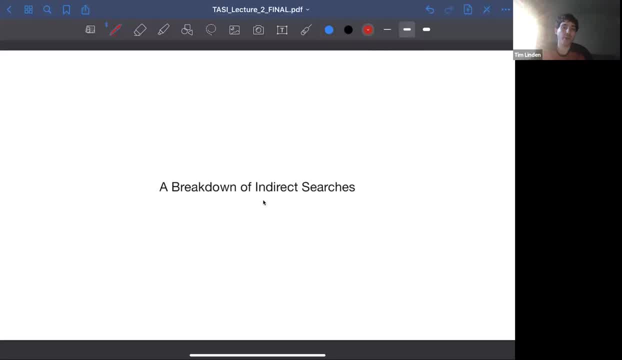 WIMP models, because you might want to do indirect detection on something that isn't a pure WIMP. So I'm there and if there are any other questions, I think a couple of questions. Okay, Since the J factor depends on the dark matter density profile. 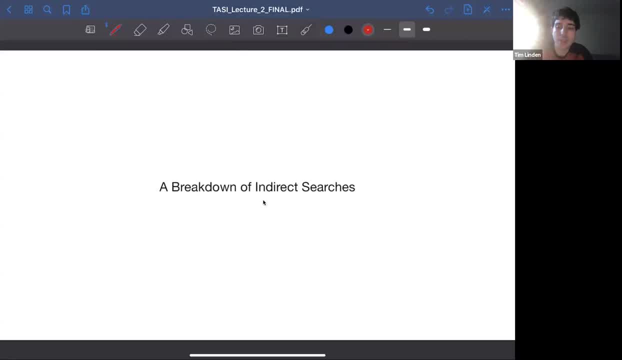 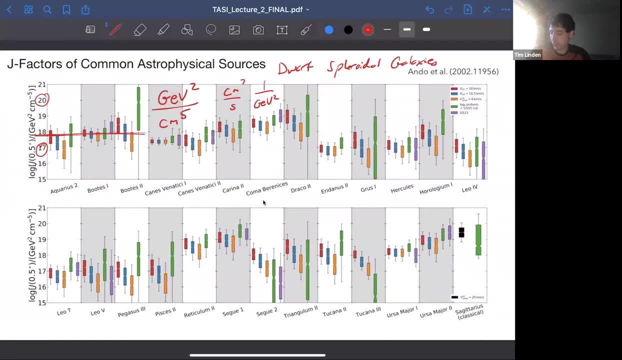 which also depends on dark matter properties in some way. yes, Good point. So here for dwarf-sphoretal galaxies. this is measured from rotation curves And it does depend a little bit on, say, NFW versus Berker. 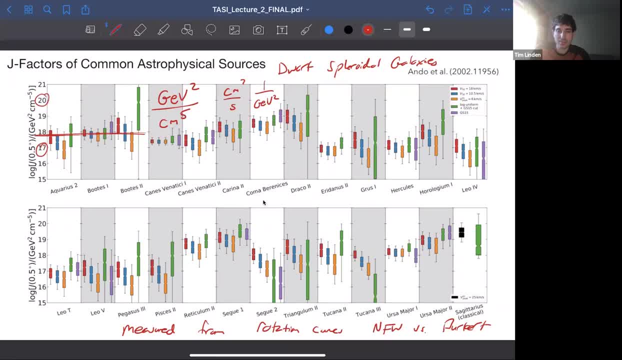 There's a really interesting calculation coincidence of figures for dwarf-sphoretal galaxies in particular, which is one of the reasons there's such good indirect searches, where we said, at the center of the galaxy, the difference between a Berker profile and an NFW. 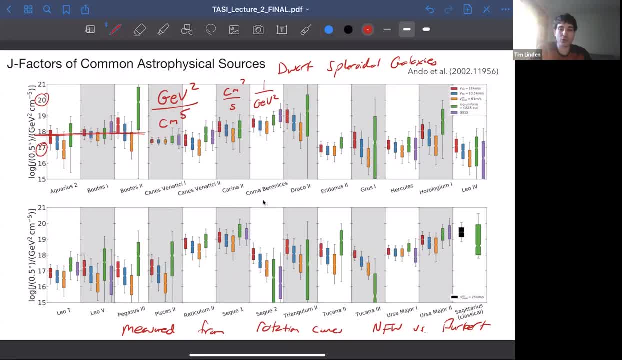 profile was like 10 to the 4. In dwarf-sphoretal galaxies it's around like 20%, which is a much smaller number. It's much smaller than all of these other uncertainty events. And then this just comes from stellar kinematic. 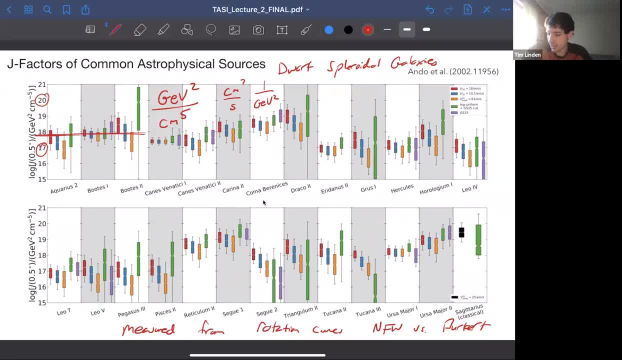 data because remember we said that the mass-to-light ratio M, dynamical over L, was around like 860 or something like that, some huge number for dwarf-sphoretal galaxies. Any rotation of the stars that exists is because of the dark matter. 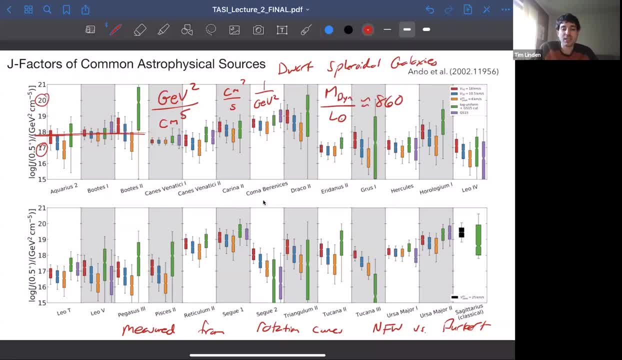 So it's actually relatively. it's statistically difficult, but the idea is relatively straightforward for how you would calculate how much dark matter is there and how much annihilation signal you expect. The other thing is that within the model of cold, collisionless dark matter, 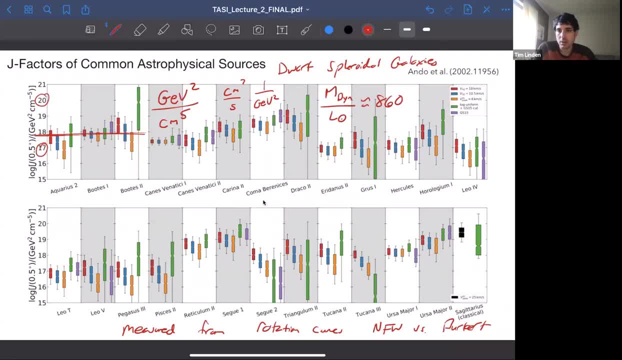 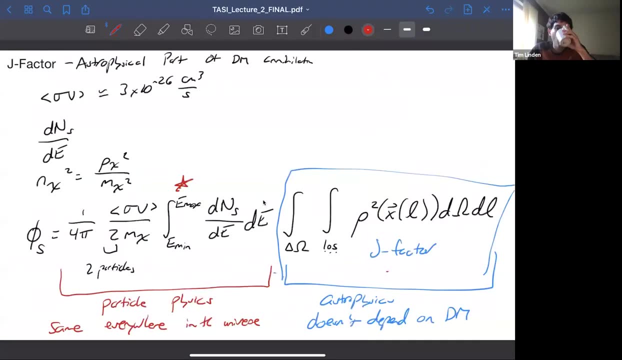 it doesn't depend on whether the dark matter the WIMP miracle, if it's just a cold, collisionless dark matter particle, doesn't change the density profile if the dark matter particle is 1 TeV or 100 GeV Right. 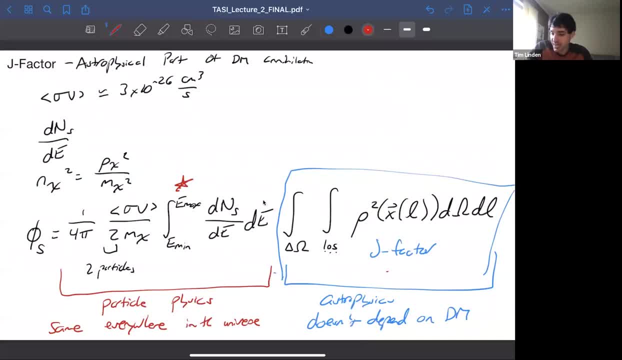 You do get different rates of the particles finding each other in this term, but this comes out here in this particle term that depends on the mass. So that's still part of the particle physics model. And then the density does not depend on on Mkai. 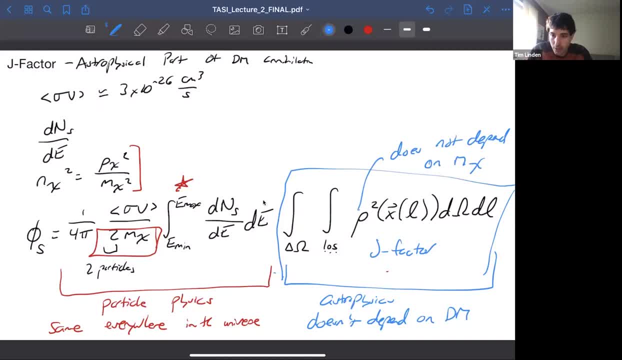 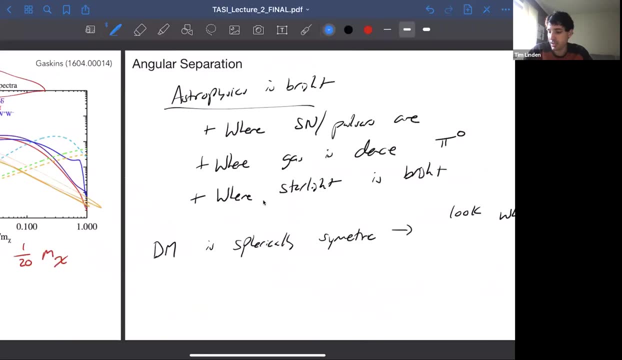 Okay, What is the basic principle which tells the energy spectrum for cosmic rays? tells whether the energy spectrum for cosmic rays is a power law or not. What makes the background spectrum a power law for all of the different types of sources? Yeah, so that comes from this calculation. 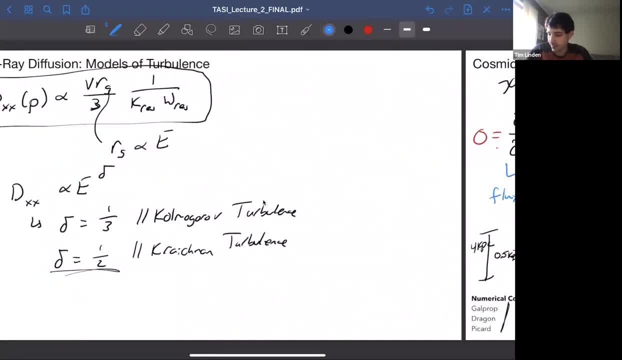 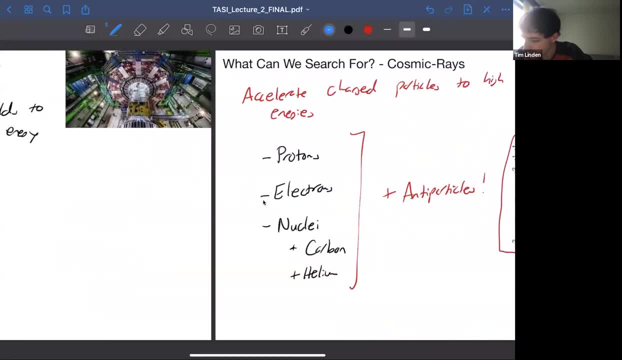 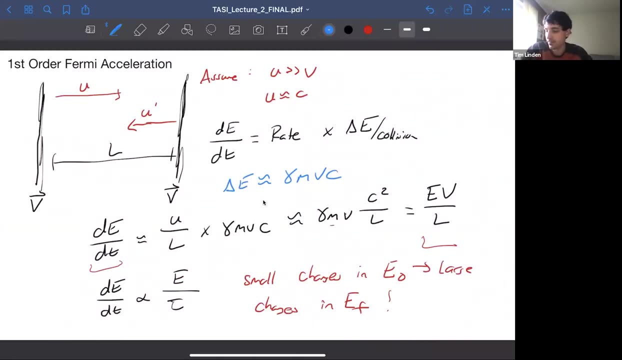 of Fermi acceleration. that sorry to make everybody dizzy by floating through 40 slides here, There's probably too many slides. This comes from this part of Fermi acceleration, basically dE. dt is proportional to the initial energy that you started with divided by some. 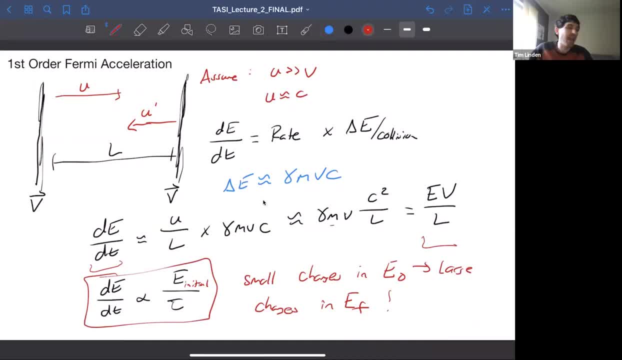 timescale, which you're doing- acceleration, Which means that if you start with any distribution of particles, magnetic acceleration tends to push them into a spectrum of particles. So in the LHC it's very fine-tuned so that this doesn't happen, right? 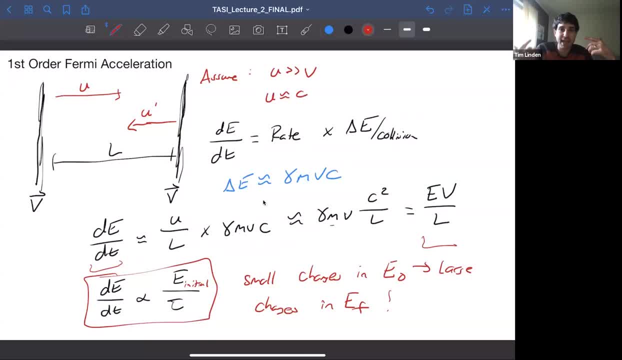 So what you have is that every particle stays in the LHC ring for exactly the same amount of time and it starts from some injector ring with almost exactly the same energy, so that the spectrum you get out of the particles is as much of a delta function as you. 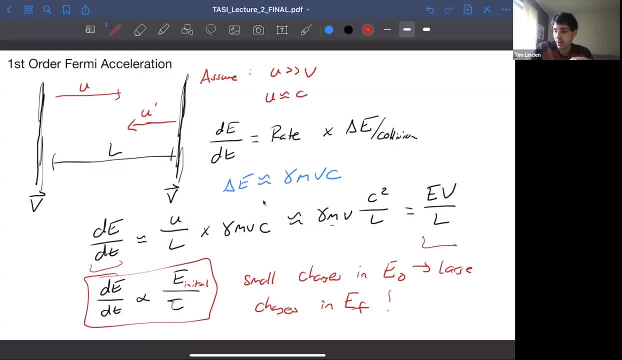 can make. On the other hand, if you're using particles, these mirrors are changing over a function of time how far along they are away. Some particles are escaping, some are bouncing back and forth a million times, some five million times, and they're all starting with. 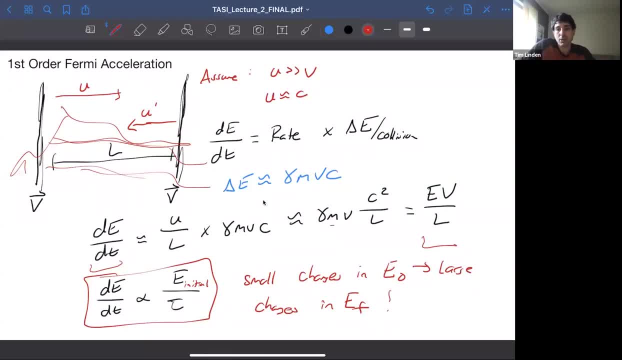 slightly different energies than what you get out as a power law spectrum. Nature loves power laws and once you produce power laws it is relatively hard to break power laws. So lots of high energy astrophysics produces power laws over long energy scales, Anything else. 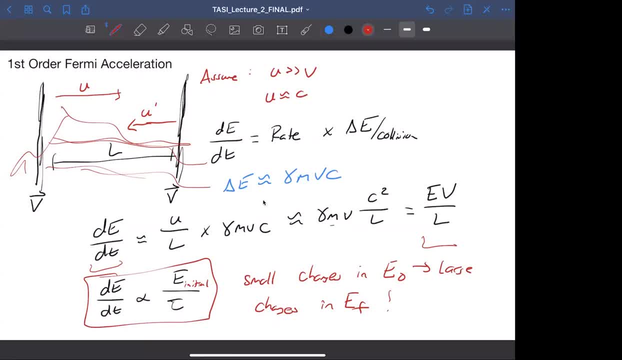 I know we're quite a bit over time now, You know. I think we should thank Tim again, virtually as we've been doing, And we have the longer break now. The next lecture is at 2 at TASI time, and then we have the coffee break. 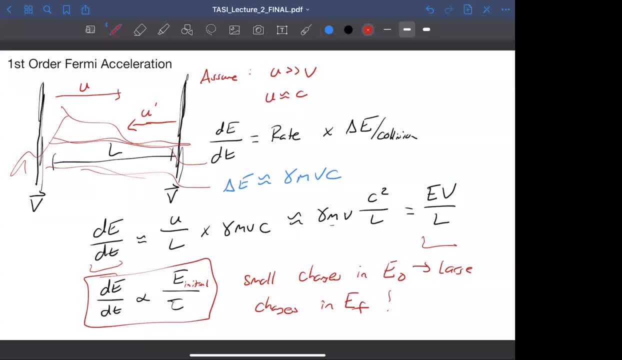 half an hour before, And I want to remind everybody- and I'll do that many times- that there is a lecture after the next lecture, so keep that in mind. And we don't have any lectures tomorrow, All right, so I'll see everybody later. Thanks, Tim. 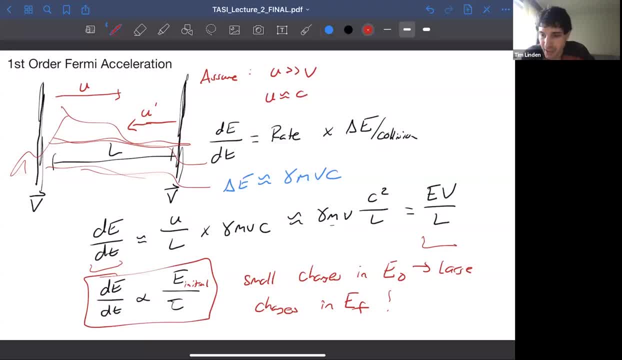 Thank you. I'll quickly answer the next question that came up, which is: is the e to the minus 2 scaling from first order Fermi? Yes, It's explicitly true for first order Fermi and it's approximately true for second order Fermi as well. 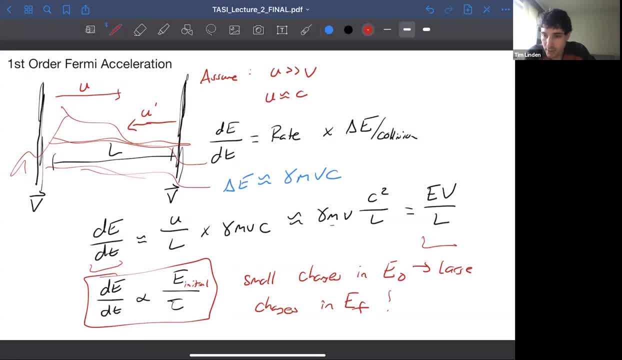 Where do I find a derivation for the equation with the J factor? The place that I go to to find it is the thesis from Alex Sterlik-Wagner, who calculates this and describes it in some detail Thesis. He has a really nice explanation of that. 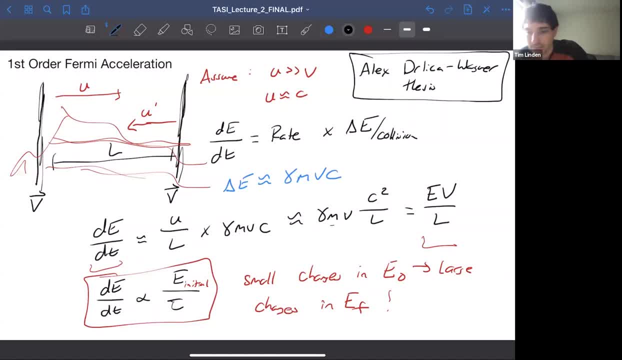 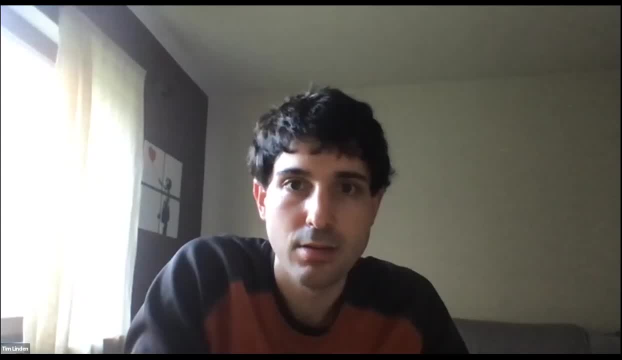 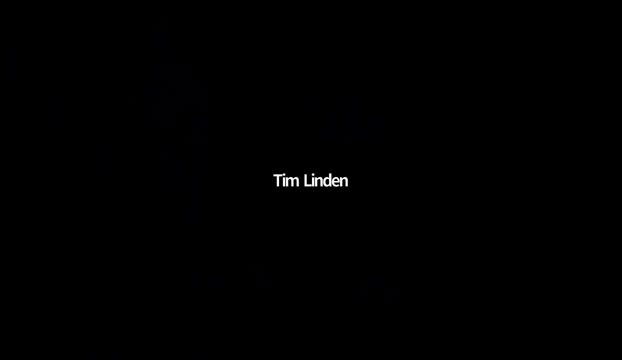